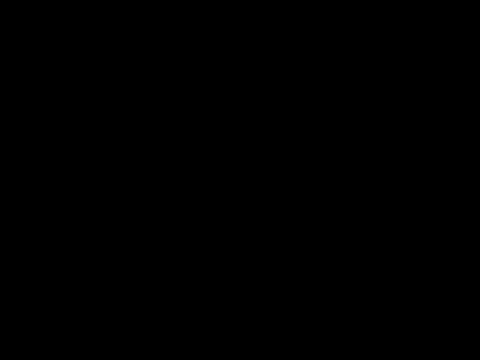 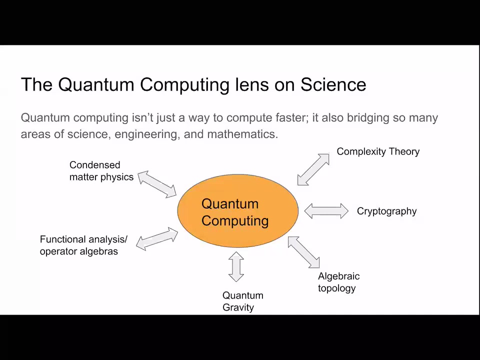 So probably all of us are aware like what an exciting time it is for quantum computing, right You know? we're starting to see that quantum computers, which are these like fundamentally different types of it's, like a different method of computing, is starting. 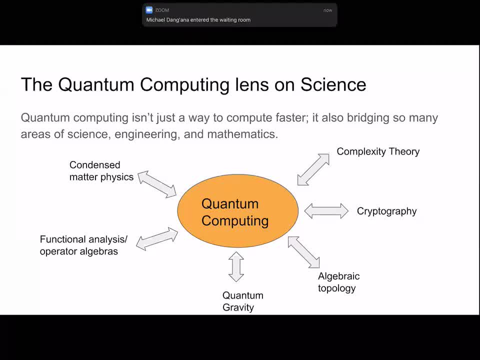 to like emerge in the real world And you know, for a long time they were just like theoretical constructs. But you know, now we hear of like companies like Google and IBM and Intel and like you know these startup companies, you know they're racing to build. 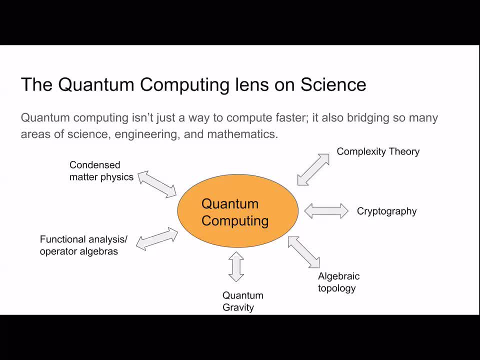 these machines and trying to figure out how to make them solve useful and interesting problems, And I think you know a bunch of you are probably involved in thinking about these sorts of things. This class, though it won't be talking so much about building 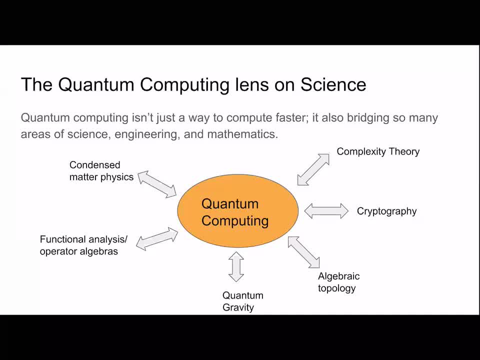 quantum computing. It's going to be talking about how to build quantum computing, And it's going to be talking about how to build quantum computers or even, you know, designing algorithms for them. So that's not really the focus of this class, But instead we're. 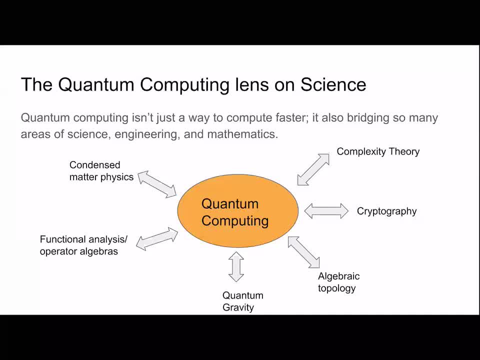 going to talk about another reason why quantum computing has been so exciting these days, And that's because it's giving a bridge between many diverse areas of science, engineering and mathematics. okay, You know, you see all these topics here that look very 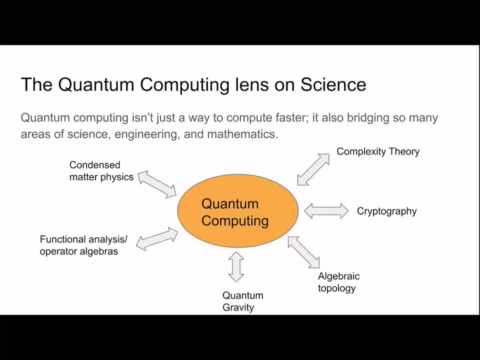 very different. you know, normally don't look related to each other, But yet quantum computing is a bridge between them all And as a bridge it's causing basically a cross-fertilization of ideas that you know, pushing the frontiers in all these fields. So this class is really 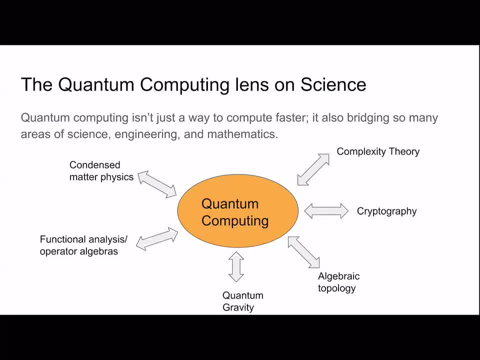 going to focus on this aspect, like how quantum computing, as you know, both a technical and a theoretical field. it's giving us insights into things like condensed matter, physics or complexity theory or, you know, pure mathematics. So the you know, the theme of this course is 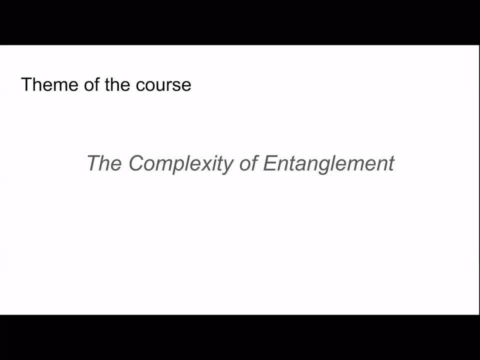 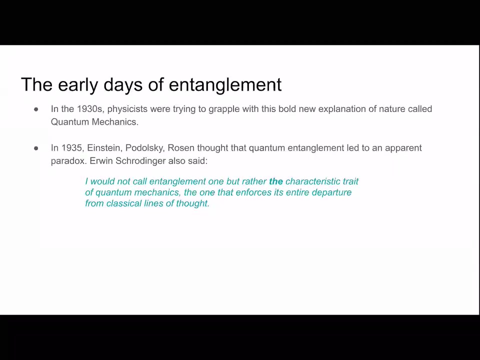 specifically going to be on something I call the complexity of entanglement, right, And I'm going to explain what that means, and I'll have to go into a little bit of history to do so. All right, So let's go back way, you know, to the way back to the beginning of the 20th. 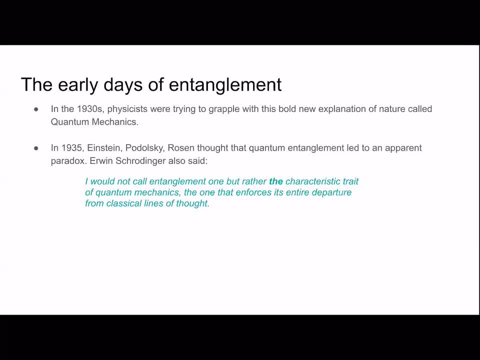 century, Back in the 1930s, you know physicists were trying to grapple with this new explanation of nature that was called quantum mechanics. You know it was just being worked out and it was just really strange. and it has all sorts of weird, you know, concepts that you 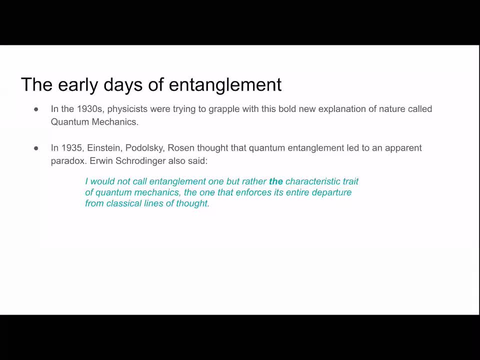 know you've heard of like things like you know, wave-particle duality or superposition or the uncertainty principle or entanglement and things like that, And all these things were like super weird and they were just trying to figure out, like how does this? 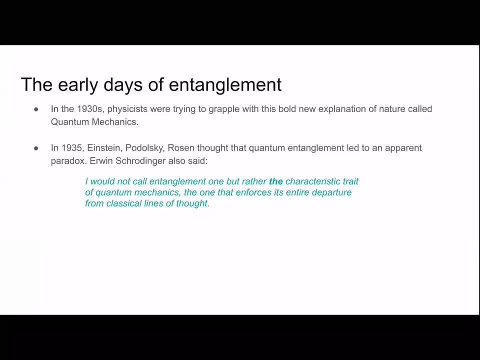 relate to our previous worldview, our previous like understanding of nature, And it didn't take long for you know the, the leading physicists of the day, to to key in on one of those really really strange things called entanglement, and they realized that this is. 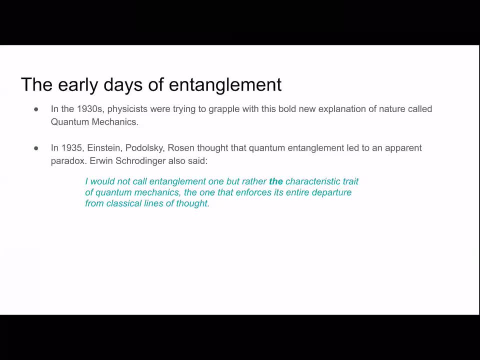 really more strange than these other things I've mentioned. So, like in particular in 1935, Einstein, Podolski and Rosen, you know they were thinking really hard about this new theory. They realized that this quantum entanglement led to an apparent 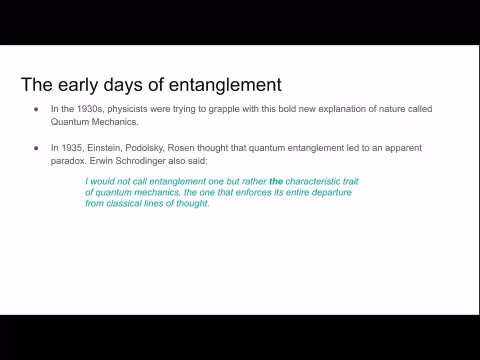 paradox. Okay, And you know quantum entanglement. basically is this phenomenon where you can, where you know the state of these two particles can't be described as the state on one particle with you know separately the state on another particle, Like their identities. 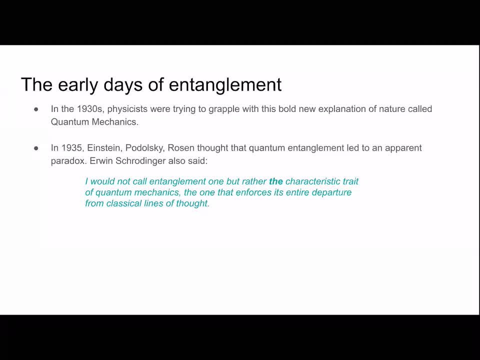 the state is, you know, intimately linked in some very strange way. And Erwin Schrodinger had this famous quote. you know, Erwin Schrodinger is like one of these, you know, famous founders of quantum mechanics. He says that I would not call entanglement. 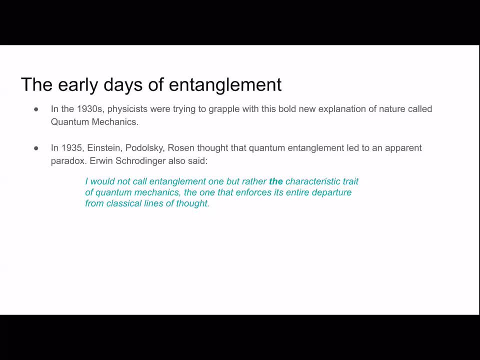 one of, but rather the characteristic trait of, quantum mechanics that enforces its entire departure from classical lines of thought. Okay, And so this is a pretty powerful statement. It really shows that he kind of understood, like what one of these key things that makes. 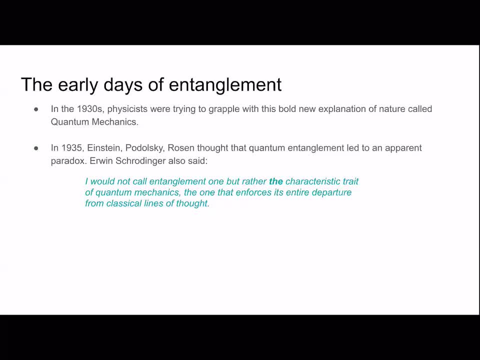 quantum mechanics, so different from classical physics. But still, you know, even though they kind of had this feeling, they had this idea, they didn't really understand why it was different. They just they just really had this feeling And it would really take until basically 30 years later before we. 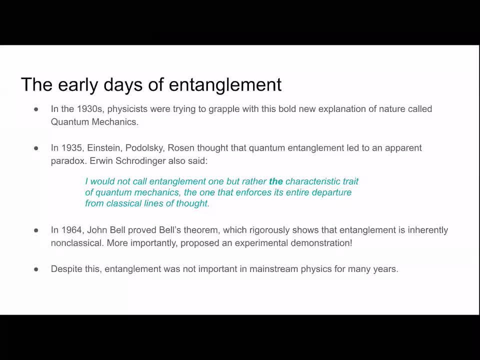 actually started having a concrete idea, explanation of why it was different. Okay, And you know, in 1964, there was this monumental insight, this realization in physics that comes from John Bell. It's called Bell's theorem, And Bell's theorem rigorously shows that this. 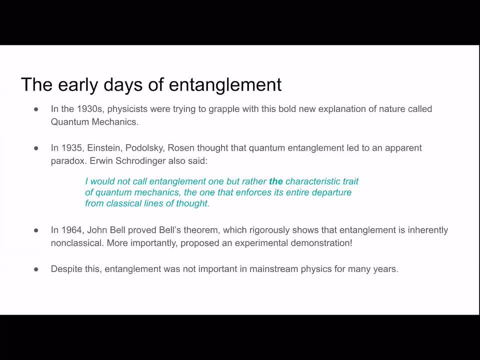 entanglement. this phenomenon is inherently non-classical. Okay, And more importantly, John Bell came up with an experimental, a proposal for an experiment, that would show this And to sort of get a sense of, like, how radical this is. you know. basically, his theorem is saying: 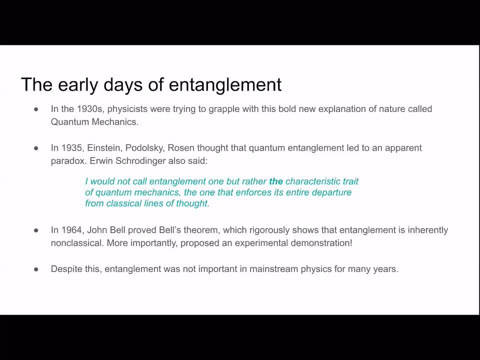 that this: there's a prediction that quantum mechanics can make about entanglement. that no classical typical theory. you know they're not. he's not even talking about just one specific classical theory. is saying all possible classical theories that you can come up with, as long as they're reasonable and 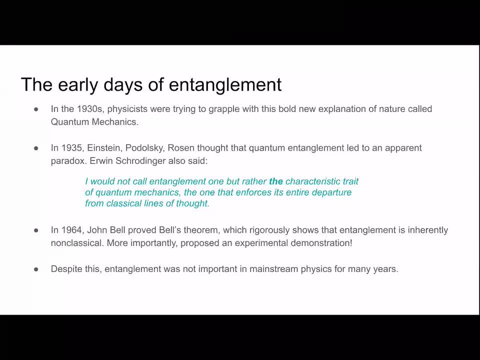 the end of the day, reasonable things like you knows light can travel faster. you know things can't travel faster than the speed of light, and so on. all such theories, no matter how you like try to work it, it cannot reproduce the same predictions as quantum physics. 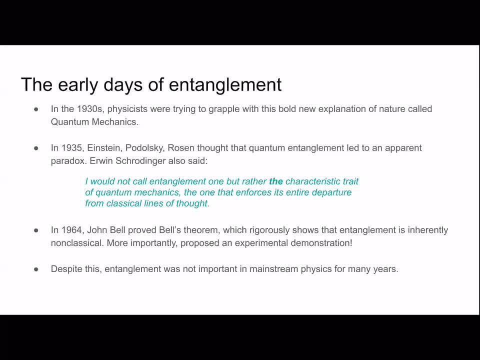 So And um, And you can run this experiment and you can see that what comes out in the real world is something that matches what quantum physics proposes and that tells you that nature cannot behave according to a classical theory that you know people like Einstein would have wanted. 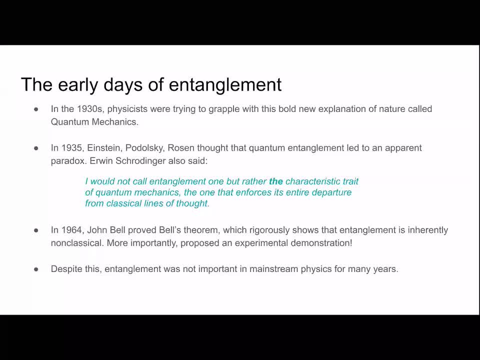 So you know we'll talk about this later today, but this is, you know, sort of how entanglement played a central role in these. you know these early days of quantum mechanics when people were trying to figure out. you know what it all means. 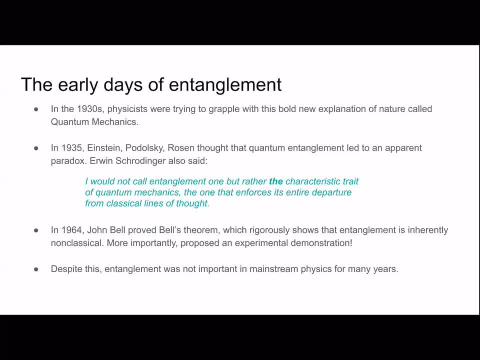 You know. but despite all of this, you know people figured this out- John Bell figured this out- but entanglement still didn't really play a very important role in physics For many years. For most of you know physics in the 20th century, you know people were focused on things like: you know, finding exotic new particles and you know figuring out like the standard model of particle physics and so on. 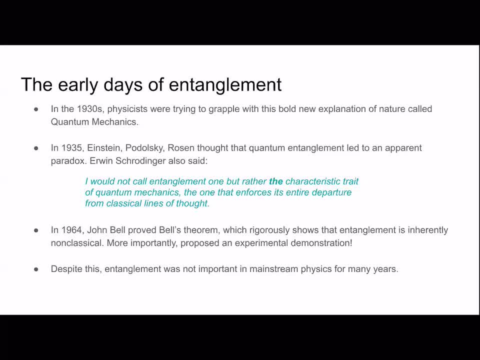 And all those things didn't really involve so much thinking about this entanglement phenomenon And actually I think you know, as far as I understand, even today, like if you're a physics major And I think a lot of you have a physics background- 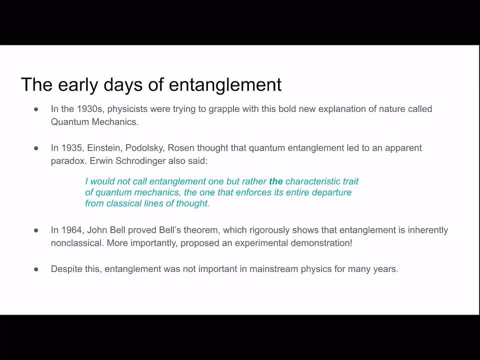 I believe that when you take classes, intro classes- to quantum mechanics, people barely mentioned quantum entanglement, if at all. Right, Although I'd be interested to hear if anyone has a different experience. So you know, this was the early days of physics. 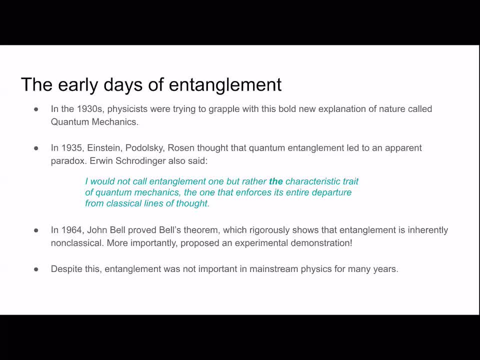 But let's fast forward to starting in the 1980s, When people started thinking about Something called quantum information. And this is where, you know, information theory, computer science and quantum physics start colliding, And now entanglement starts to take more of a center stage in people's thinking about quantum physics. 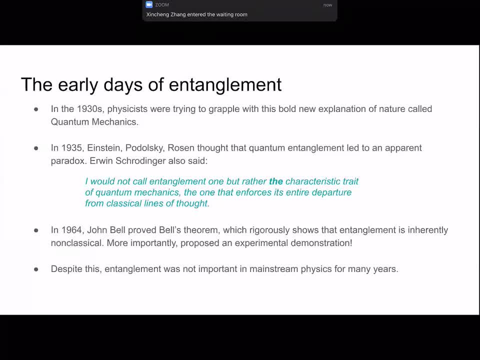 And the reason for this Is that people started realizing a bunch of things. Number one: Entanglement in quantum physical systems is a barrier to efficient simulation. So entanglement is the reason that if you have n particles, To describe them classically would require at least two to the n parameters to fully describe the state right, an exponential number of parameters. and for you know, 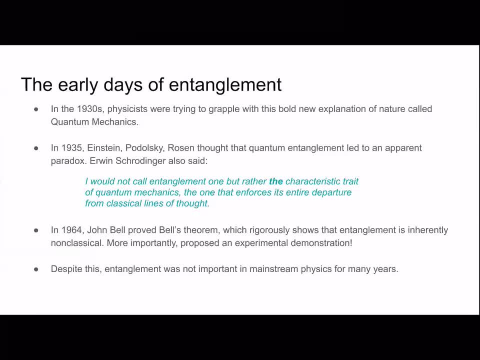 For not, you know, and that's not small. This is just way too large right to describe, And this is a reason why trying to simulate quantum physics On a scale Right On a classical computer, on the computers that were used to today, is really an intractable tasks like. we don't know how to do this efficiently and it makes understanding quantum physics very difficult if we want to try to simulate. 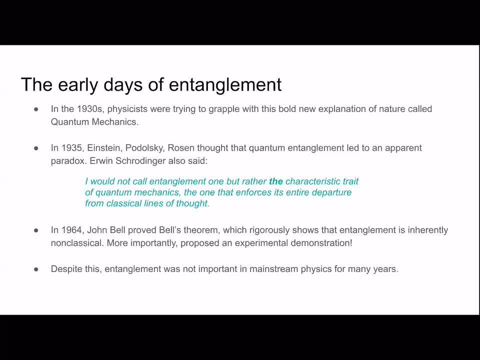 But on the flip side, people also started realizing that entanglement is like a really useful information processing resource. So it's entanglement is not just this weird thing out of nature where you have these like linked particles and and so on, but you can actually use it. 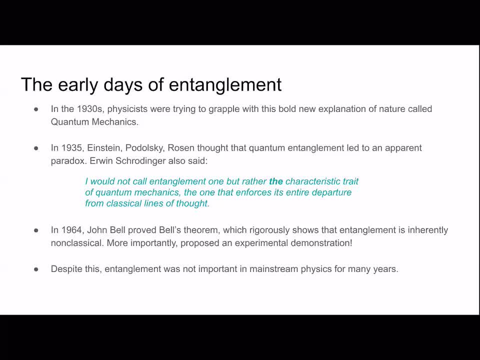 To perform interesting communication or information processing tasks. like you can use quantum entanglement to generate perfectly secure secret keys between two distant parties that they might want to use for a cryptographic tasks, You can also use entanglement for teleporting quantum states between one place and another. 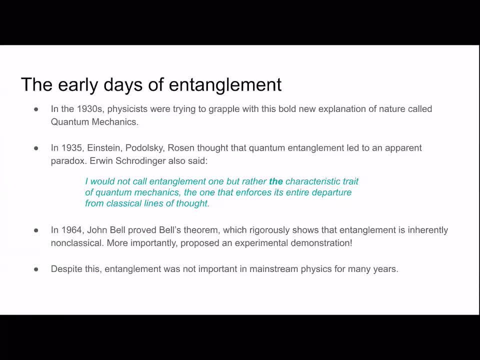 And so on, Right. So Once people wanted to do something with This quantum entanglement, then they started realizing what we have to understand it better. And also from just a fundamental physics point of view, people are starting to realize that entanglement. 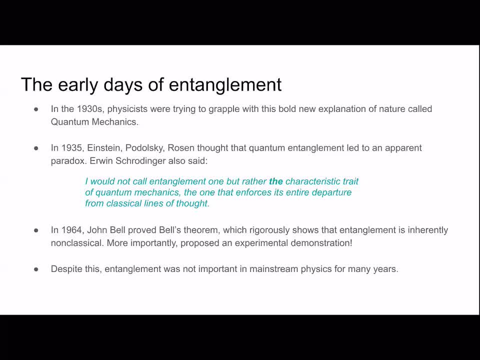 is behind some really exotic quantum phenomenon that you see in nature- things like superconductors. So this thing on the left-hand side is a picture of a superconductor. It's this little puck at the bottom and cool to some really low temperatures. 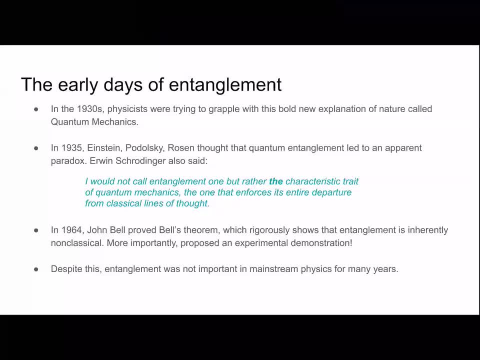 And it generates things like this levitating cube. And really the reason that superconductivity is possible is people believe it's because of very large-scale quantum entanglements between many particles. Things like the Bose-Einstein condensates are due to entanglement. 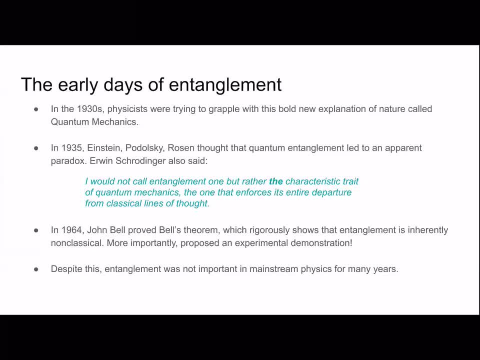 And even things that are super large and cosmic in nature: black holes. black hole evaporation: people believe it's due to quantum entanglement And it's already the most complex of all, And the more complex it is, I think. 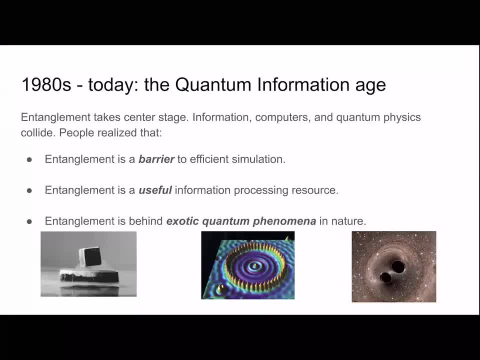 the better you can get. at the end of the day, that the more complex it is, the better it is. So there's a duality and there's a counter-interferencing that we call this campsite entanglement but a claim between two superconductors. 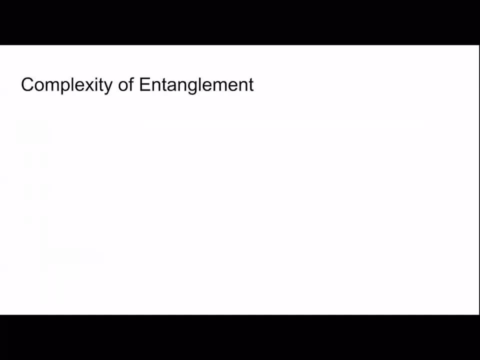 is, there are two types of entanglements. One is that there's a thermo-physical element, that the temperature is higher than the temperature, that the temperature is lower than the temperature, that the temperature is high, And the other thing that's really additional. Well, what do I mean by this? It's a computer science and information processing perspective. 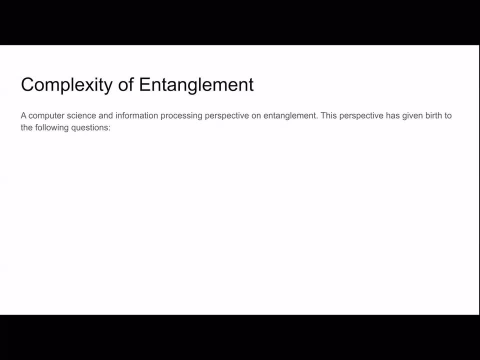 on this phenomenon, And this perspective has given birth to a bunch of really interesting questions that on the surface just seem completely unrelated. So here's some examples of these questions. Number one: can quantum systems that you find in nature? can you describe them using? 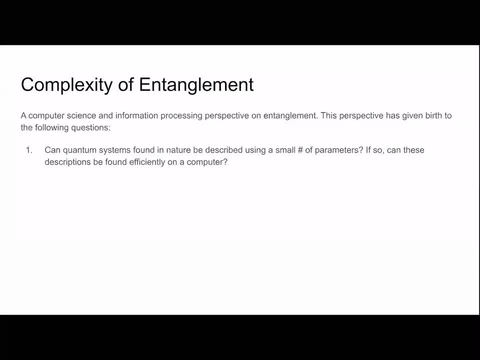 a small number of parameters, And if so, can these descriptions be efficiently found on a computer, classical or quantum? I just mentioned that entanglement is useful for information processing, but can unentanglement be useful? You know what does that mean? We'll talk about that. 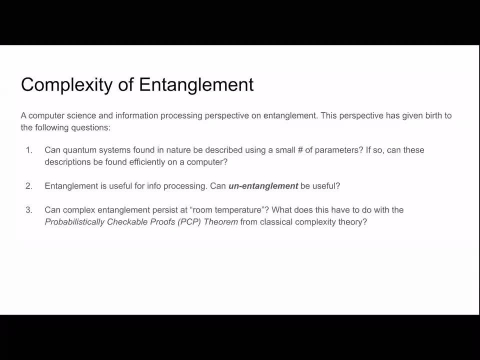 later. Can complex entanglement, like the types that you've just described, be useful for information processing? Can complex entanglement be useful for information processing? Can complex entanglement be useful for information processing That you find in superconductors? can they persist at room temperature? So this is one of the 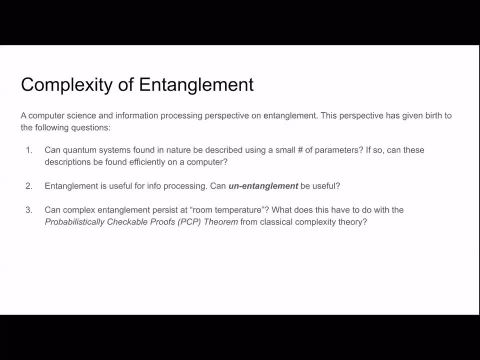 holy grails of engineering physics. Can you design a superconductor that has its superconducting properties happen not at, you know, near absolute zero, but, say, closer to room temperature? Okay, this is a big open question And apparently one can frame this in such a way that it can be. 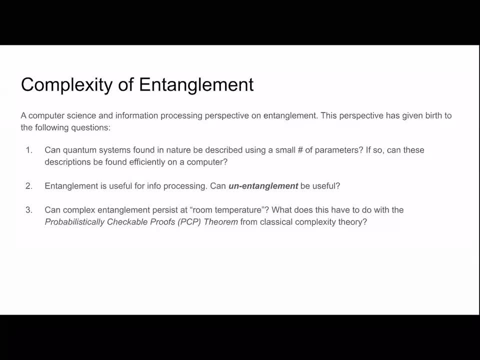 connected to something that's called the probabilistically checkable proofs or PCP theorem. that comes from classical complexity theory, So that's something that's just pure computer science. There's like, actually, it turns out, a deep connection between that and the notions of 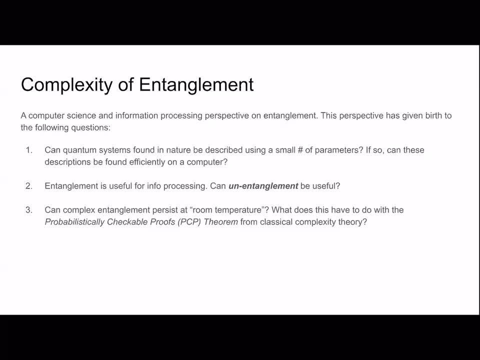 whether complex entanglement can persist at high temperatures or high energies. Here's something pretty different. Is it possible to verify a quantum computation using only classical complexity theory? Is it possible to verify a quantum computation using only classical resources? And here's another one: What is the complexity of something called quantum? 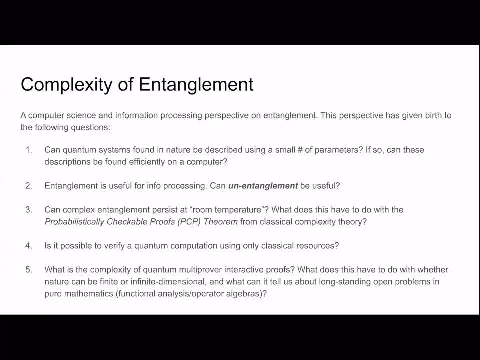 multi-prover interactive proofs. It's kind of a mouthful, And whatever that thing is, what does it have to do with whether nature can be finite or infinite dimensional? And furthermore, what can this tell us about long standing open problems in pure mathematics? 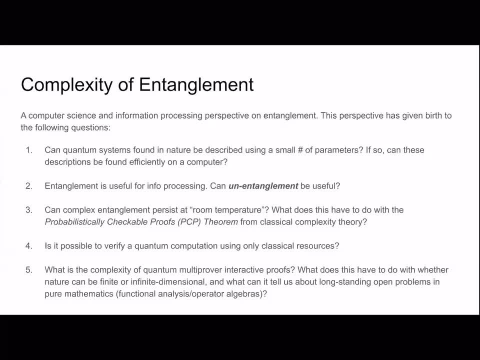 Specifically functional analysis and operator algebras. So this is like a wild collection of different questions And in this class we'll see how all of these questions relate to each other And a lot of them are active areas of research. We don't have the answers. 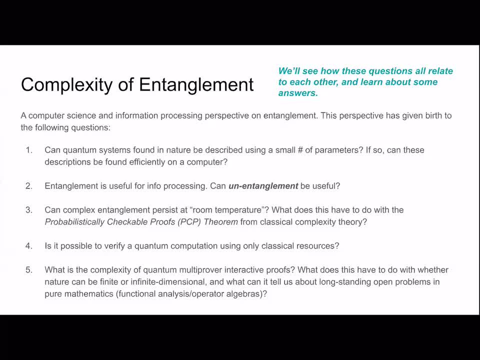 but for some of them we do have answers and we'll learn about that, So you know. so this is like a brief introduction to to what this class is going to cover, at least thematically. Any questions so far before I jump into things like the class mechanics. 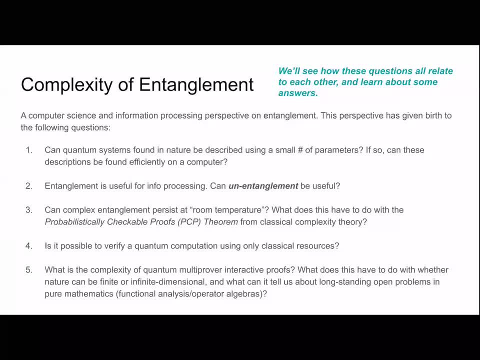 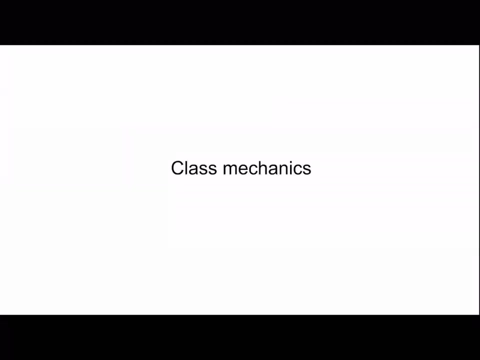 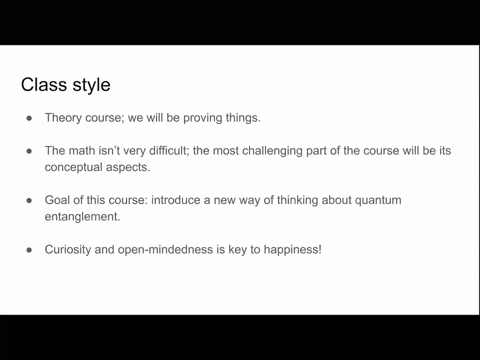 Oh, sorry, I just saw everyone's message about the picture. Yeah, great thanks, No problem, OK. so let's go on to administrative things about how this class is going to be run and what's its style. So this class is going to be a theory course, So you know we'll be. 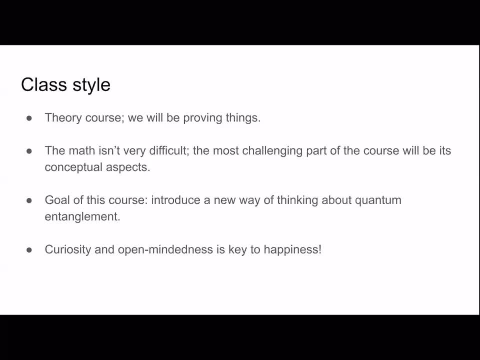 proving things. But the math is not going to be very difficult, I don't think. But really I would say that the most challenging part of this course will be its conceptual aspects. aspects, I mean, we're going to talk about all sorts of different topics, you know. 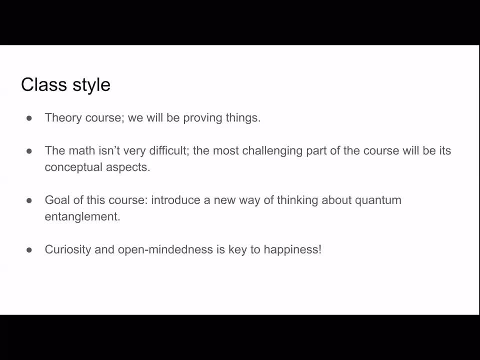 from physics, from complexity theory, from, you know, from cryptography and so on, And we're going to mash all of these concepts together And so really trying to wrap our heads around it. that's going to be the most interesting, and you know. 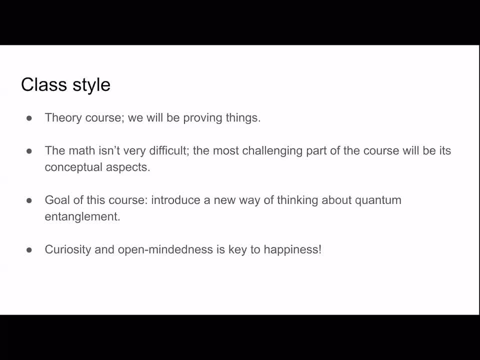 mentally challenging part And really the goal of this course is going to be introducing a new way of thinking about quantum entanglement and how can we use it. you know, how can we think about it, how can we analyze it, And in this course and 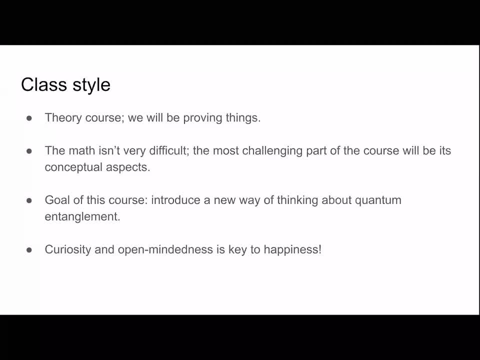 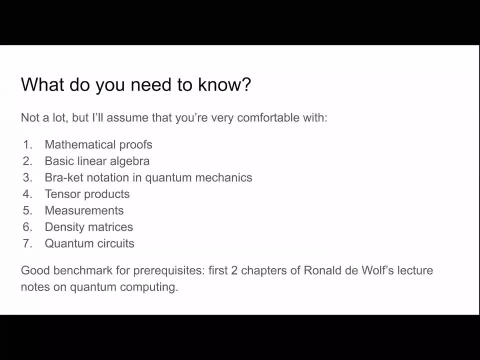 also, you know, in life in general, curiosity and open-mindedness is going to be the key to happiness. Okay, so what do you need to know for this course? What are the prerequisites? Not a lot, Okay. so what do you need to know for this course? What are the prerequisites? 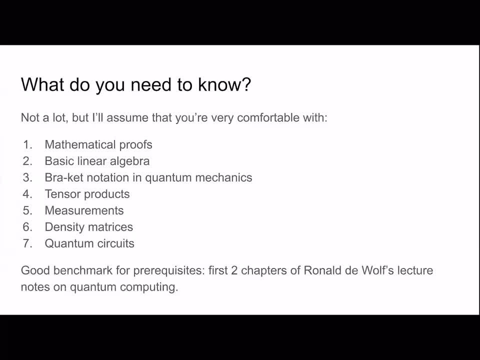 Not a lot, But I'm going to assume that you're very comfortable with some basic things, Things like you know: mathematical proofs. You should be comfortable with seeing a mathematical proof and understanding it how it works, Basic linear algebra. okay, I won't use anything more than you know first-year. 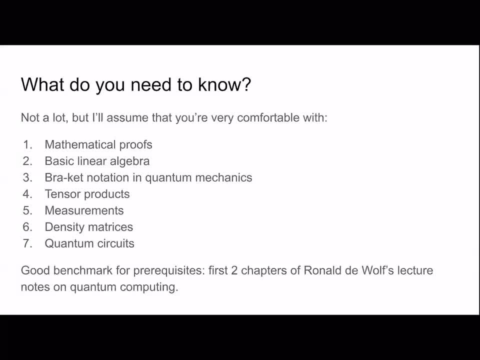 linear algebra. But it's basically I'm going to assume that you're very comfortable and you know you've seen it a lot. In terms of notation, I'm going to assume that you're familiar with this Braquette notation that's used in 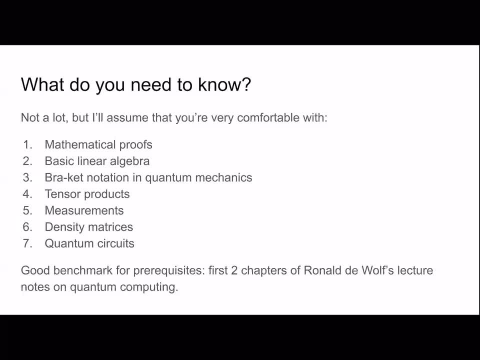 quantum mechanics and quantum information. You know concepts like tensor products, measurements, density, matrices. You know, basically, I'm going to assume And we're going to see a little bit of quantum circuits, but you don't. you won't need to. 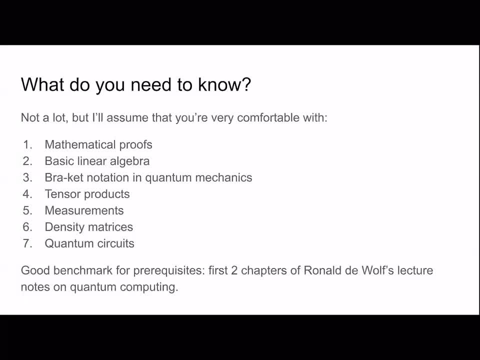 know any specific quantum algorithms or anything like that. A good benchmark for seeing if you are comfortable with these prerequisites are the first two chapters of Ronald DeWolf's lecture notes on quantum computing. There's a link to it in the class syllabus so you can take a look at that. 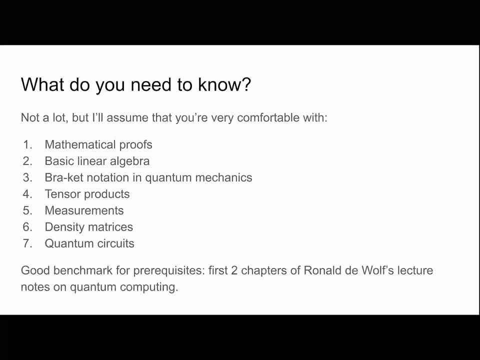 Even if you feel like you're a little rusty on this or you might have not even seen some of this, it's okay as long as you're willing and motivated to learn these things on your own and on the fly, And if you're not sure, just feel free to. 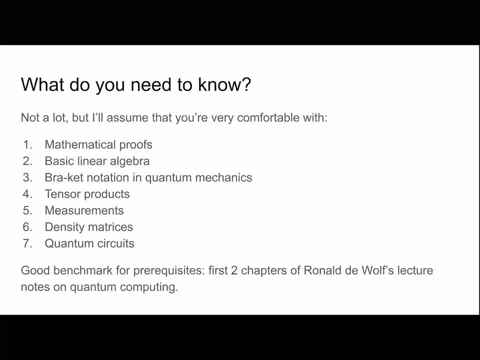 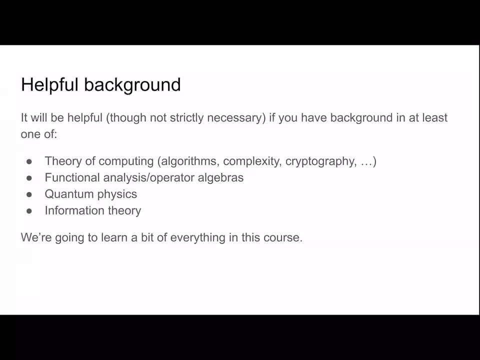 send me a message and ask me and talk to me about it. I'd be more than happy to help you figure out whether you could use it. You have the appropriate background And it'll be really helpful, but not necessary. but if you have background, at least one of 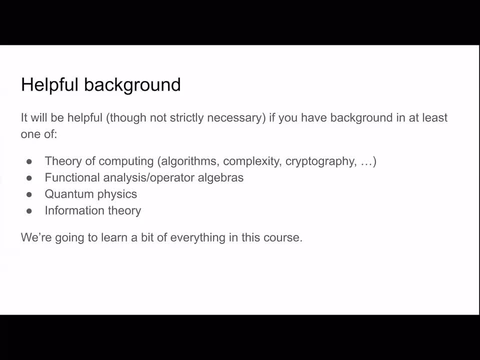 these topics you know, say like theory of computing, like you've taken an algorithms or complexity class before. or you know, maybe you come from a math background and you have some functional analysis class that you've taken, or you're, maybe you're, you're, you're. 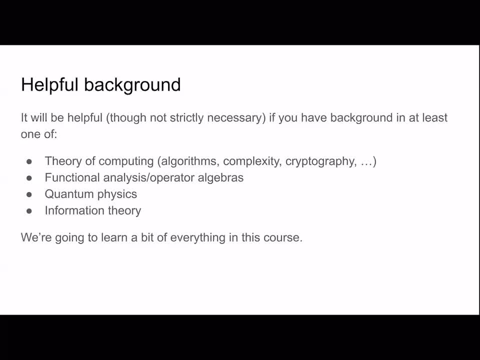 you're a physics major, that'll be really helpful because it'll give you a way to, it'll sort of give you an anchor to- to understand certain parts of the course and from which you can, you know, understand the other. you know the other parts. 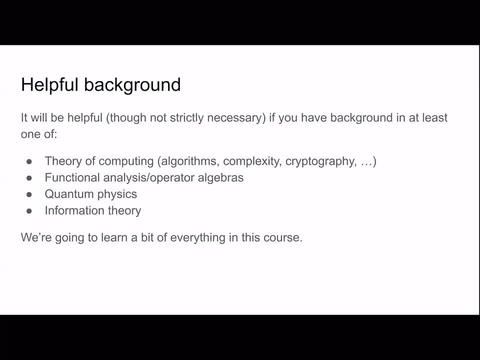 But really we're going to, like I said, we're going to learn a bit of everything. right, We're going to cover some physics, some, you know, pure mathematics, some complexity theory. So you know, if you're a physicist, get prepared to learn about some theoretical computer science. 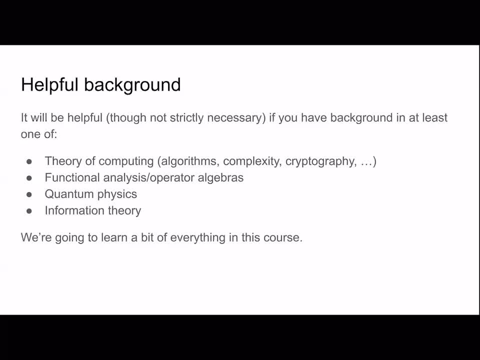 If you're a computer scientist. maybe you know you're a computer scientist, maybe you're a computer scientist, maybe you're a computer scientist. maybe you're a computer scientist, but you'll learn about some functional analysis for the first time. 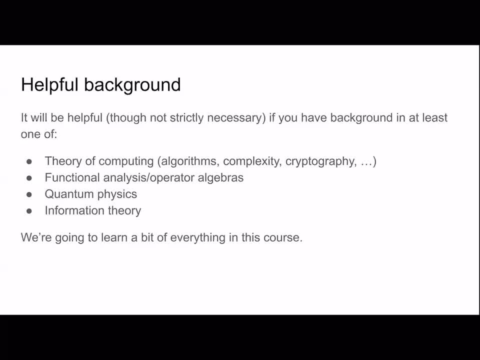 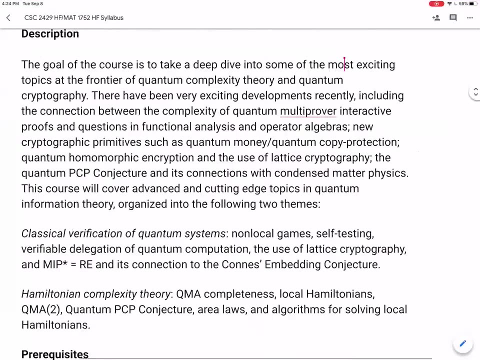 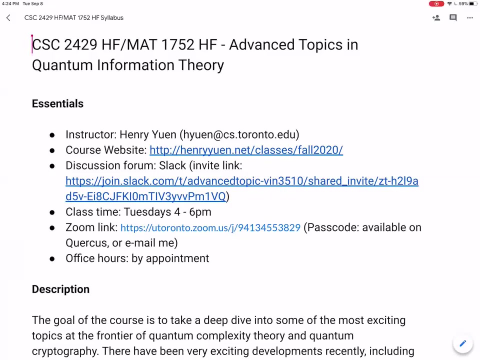 Good Okay, Now let me turn to the syllabus and continue with that. Good Okay, So so this is like the, the class information, The course website. This is where I'm going to post things like The lecture notes, links to recordings of the lectures and also the problem sets. 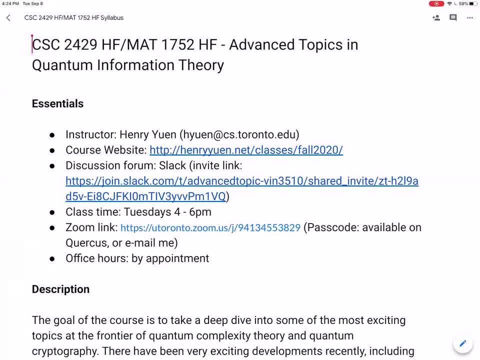 Okay, So, so all, almost all of the things will be posted up there. We're going to use Slack as a way to just discuss and, you know, ask questions in this course like, or ask questions about like the problem sets, or the lectures, or, or just 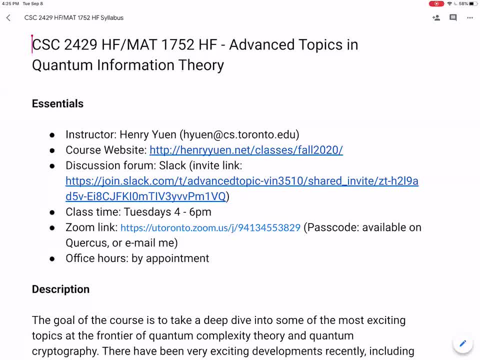 talk about things related to the course in general. So I highly recommend that you join the Slack and it'll be a way for us to keep in touch with each other throughout this course. We're going to use the Zoom link. Hopefully the Zoom link won't change. 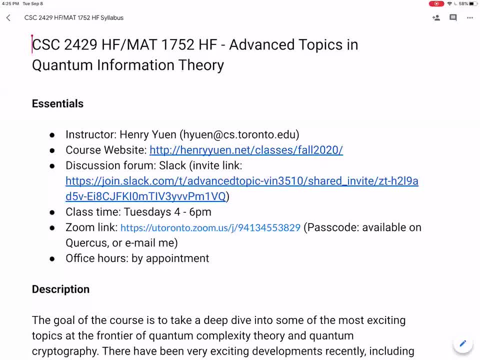 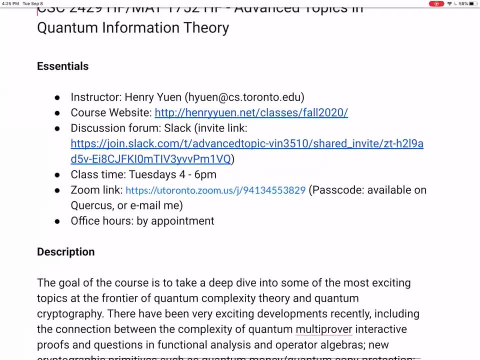 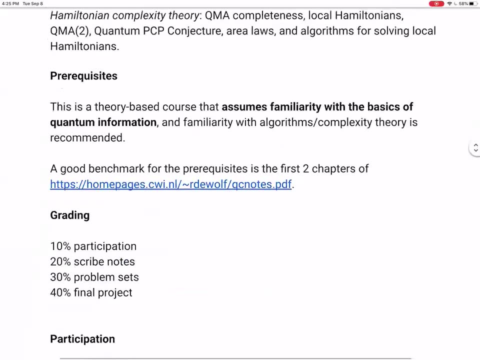 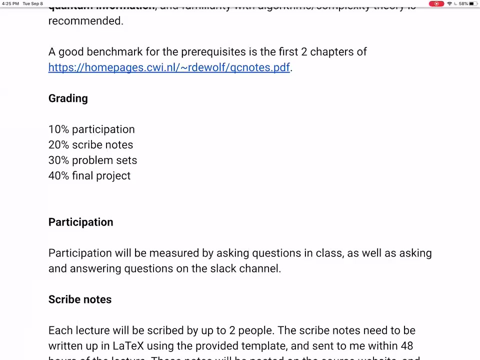 And you know you, since you're in this lecture, you have this passcode, but if you lose it for any reason, you can just email me. Let's see, We talked about the prerequisites, Okay, So in terms of coursework, the grading consists of a bunch of things. 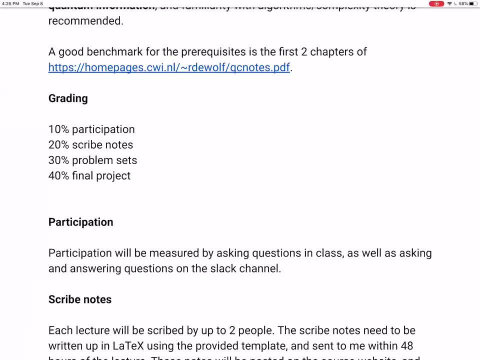 One is: you know there's 10% participation. That's pretty easy. All you know you have to do is just be engaged in class. you know ask questions as well as you know asking and answering questions on the Slack channel. 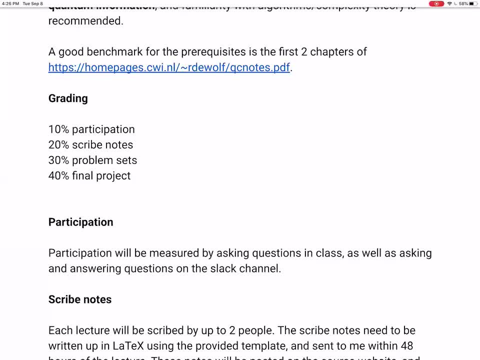 And for those who are in Like a very weird time zone- you know who can't make the class- then that will be counted in terms of like participation in the Slack channel. So hopefully we get some lively discussions up, especially once we start getting the problem. 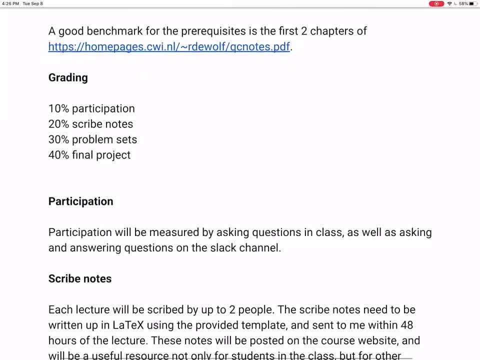 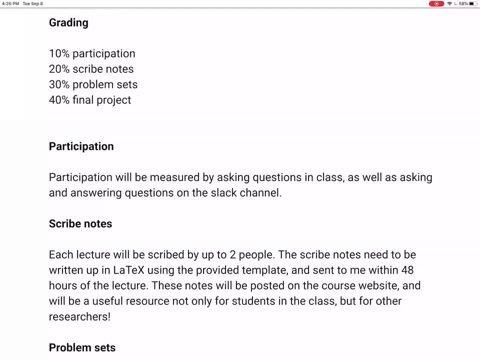 sets out, 20% of the class will be scribe notes And Each lecture will be scribed by. I think, based on the course, enrollment will be by two people And you know so, so I'll set up a sign up sheet where people can volunteer for sign. 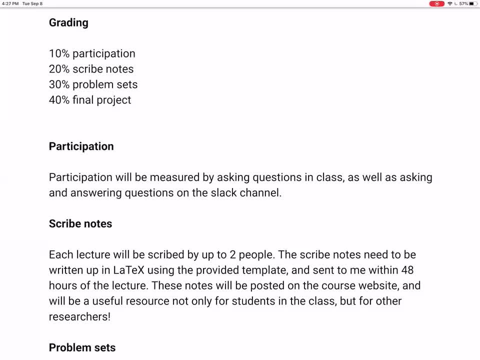 up for for different lectures that they want to scribe. for I'm going to provide a latex template pre-filled with some of my rough notes that I've written for myself, And then what you and your partner will do when, when scribing a lecture. 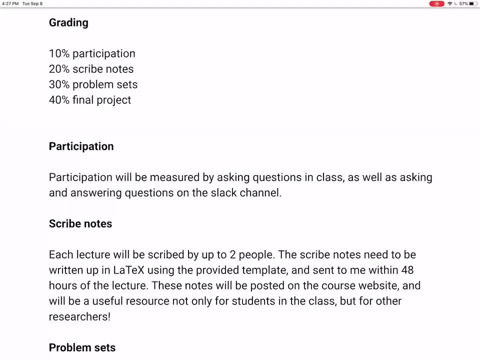 Is you'll just sort of fill in the details and make it nice And you know, ultimately these scribe notes will be posted online, Not just for this class but also for other people outside who are interested in this material, And you know they can read it and use it for for themselves. 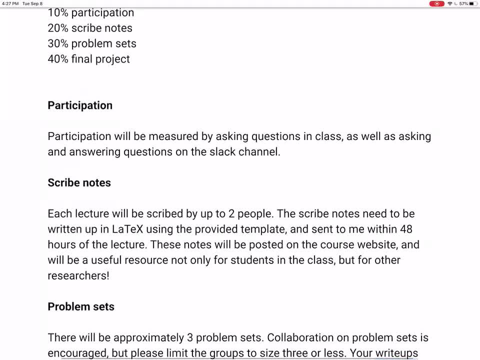 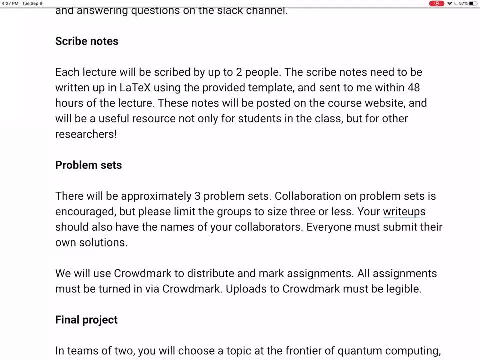 Okay, good So. so the next part is problem sets. I think there's going to be three problem sets in this course. Collaboration on problem sets is encouraged, highly, highly encouraged, but please keep your group sizes to three or less. 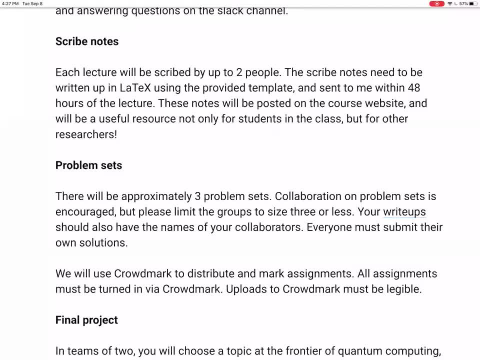 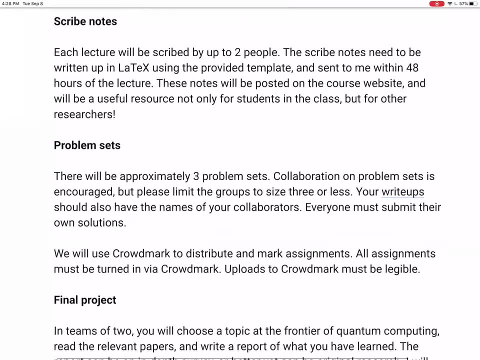 And when you write up your problem solutions, your write-ups should also have the name of your collaborators, And everyone has to submit their own solutions, And we're going to use something called Crowdmark. Maybe some of you have seen this before. It's just an online submission website where you can just upload your your homework. 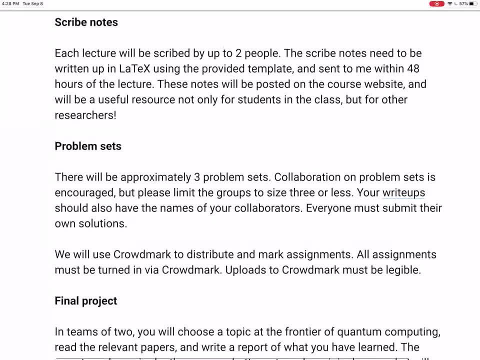 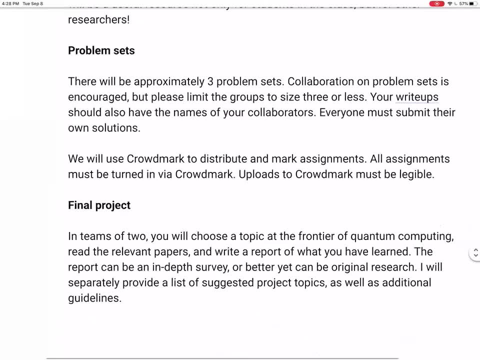 Okay, And finally, outside of the problem sets, there's going to be a final project in this course And in PEARS. basically, it's just a chance for you to explore a topic of your interest a little more deeply. So you're going to pick some topics. 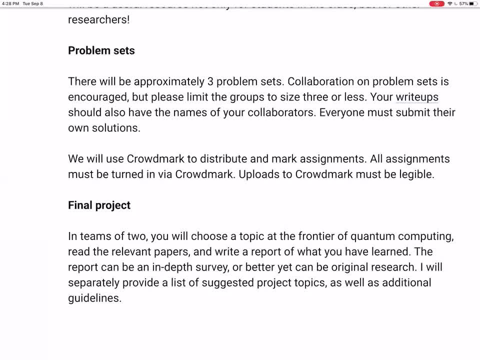 I'll have a list of suggested topics that you can read. You can read the relevant papers and write a short report of what you learned. If you want to do original research, That'd be awesome, Super great, But you don't have to. you can do. at the very least, you should do like an in-depth survey. 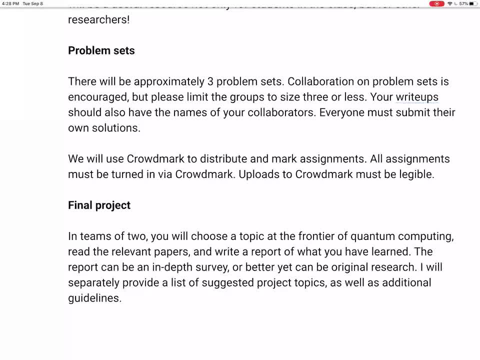 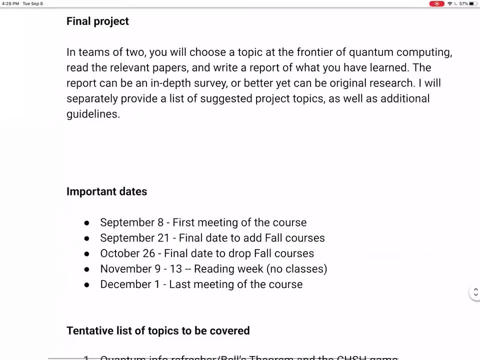 of the particular topic And later in the, in a couple of weeks, I'll post a project guideline. Okay, Let's see What else. Some important dates. In the syllabus I've written a list of topics, Topics that we'll cover. 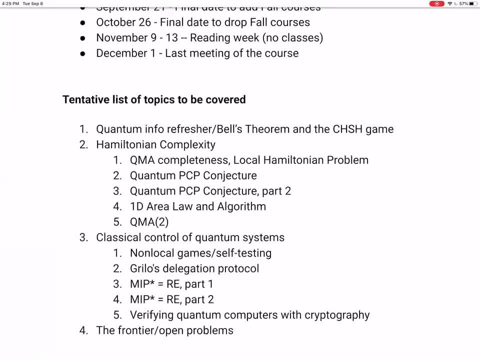 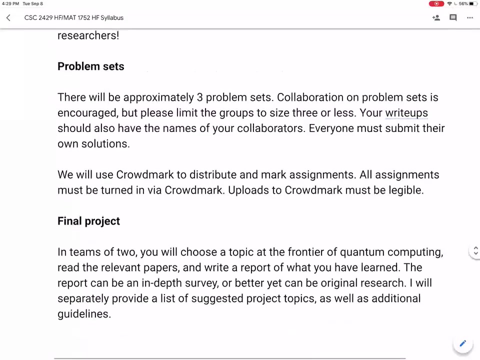 There's there's 12 meetings of this class And so there's there's 12 topics. Yeah, So that's the the course mechanics. Any questions so far? May I ask? if Yeah, Yeah, Are we going to get to a point where we'll be able to have an overview of the of the? 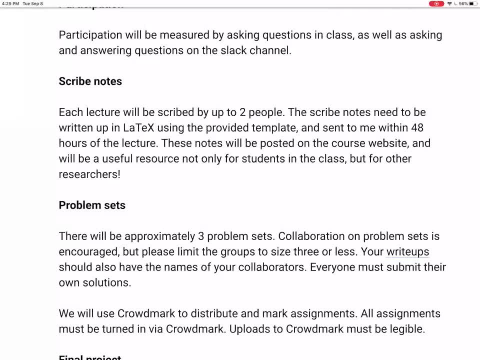 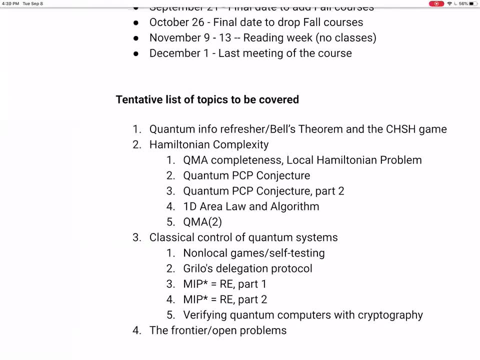 proof of the cons embedding problem. Hopefully, Yeah, So this will come a little later in the course. So in this section where it talks about MIP star equals RE, those two lectures will be devoted to covering the connection between this con embedding problem that you mentioned. 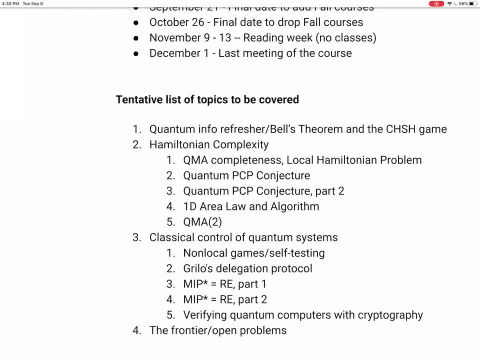 and and MIP star equals RE- Show the connection And also talk about. I mean, we won't be able to see all parts of the proof because it's quite long, but at least the the basic concepts and the outline of what's going on. 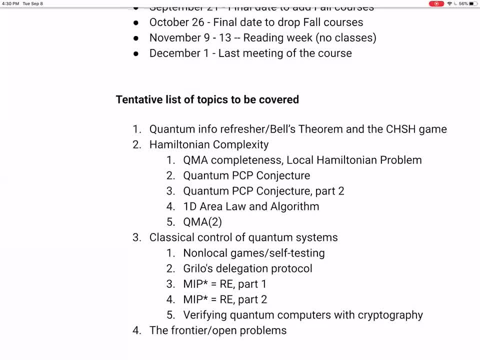 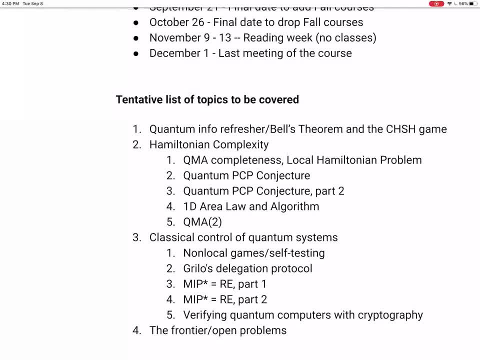 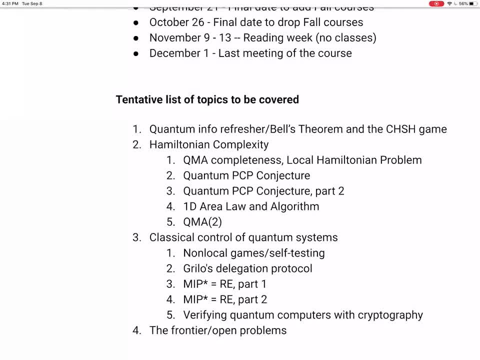 but it's always helpful to just get a very quick refresher and in particular, we're going to talk about Bell's theorem, the thing that I mentioned earlier and talk about, in particular, this thing called the CHSH game. So I'll start that for the next talk about that. for the next 30 minutes We'll 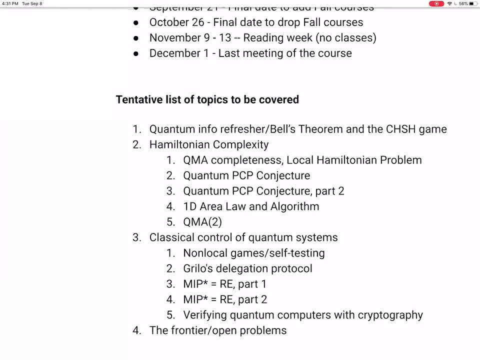 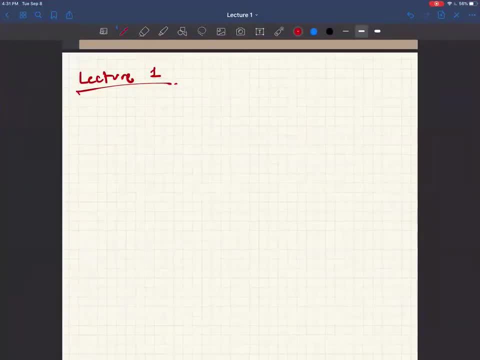 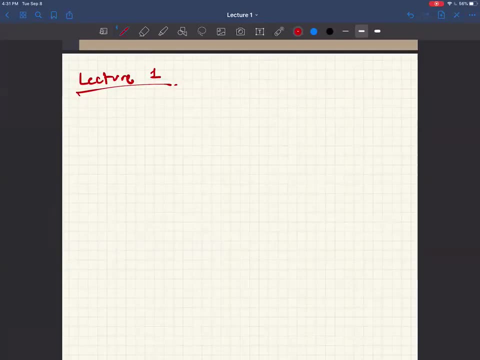 take a five-minute break and then continue on. So let me now turn to Snopad. Hopefully everyone can see it, Okay, Oh, actually, speaking of which, so I need two scribes for today. Would anyone like to volunteer for scribing today's lecture? And it's pretty simple, because 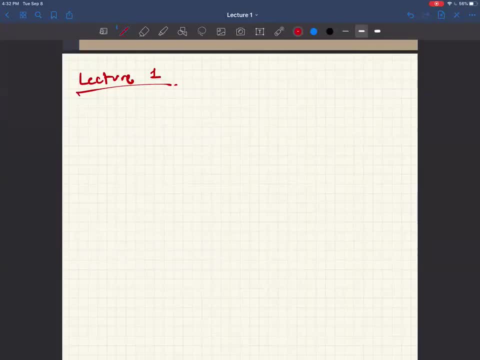 you know, actually most of the notes are done. You just have to, like, turn them into complete sentences and so forth. Okay, Abhinav, great, And Dipanshu, Okay, cool. So we have our first two volunteers. Let's get into it. So brief, quantum info refresher. 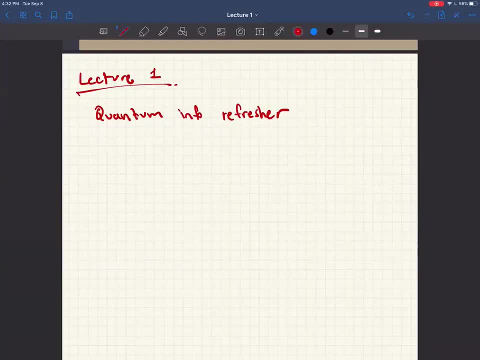 All right, So let's talk about what a d-dimensional quantum state is. All right, So this is going to be represented by ket, psi And it's a some linear combination. It's a superposition of d classical states. So i is an index that runs from 1 through d. 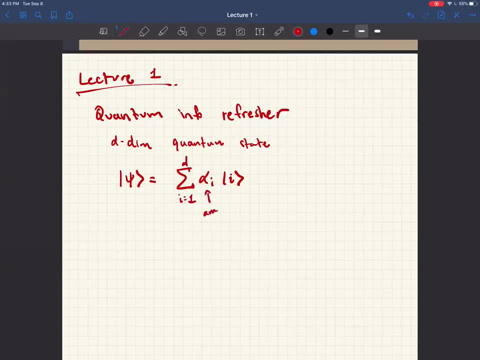 It has some amplitude, alpha sub i. Okay, And this is a d-dimensional unit vector in complex space, right? So you should be very familiar with this. And if you take this quantum state, this d-dimensional system, and you measured it in the standard basis, 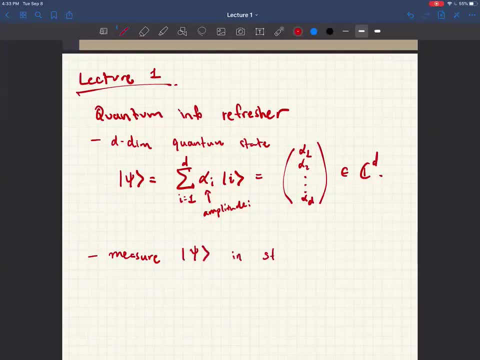 if you measure psi. so what does this mean? The standard basis is just the basis that's spanned by each of these elementary vectors: ket 1, ket 2, up to ket d. You're going to obtain an outcome. You're going to obtain one of these d classical states with probability. 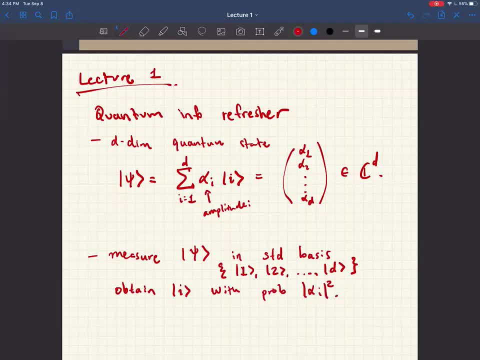 the norm of alpha, i squared Okay. And furthermore, your state psi: it collapses, It gets changed, So state psi collapses to the state i. So if you measure it again, you're just going to get the outcome i again, with 100% probability. 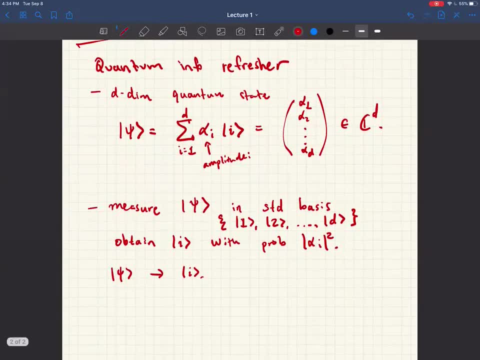 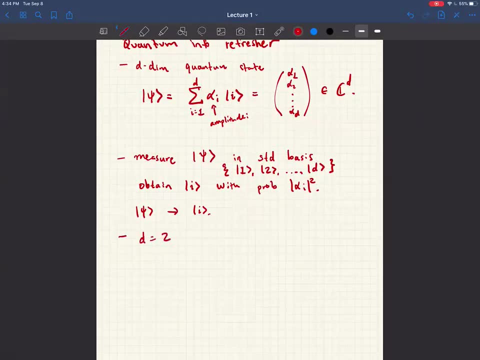 Okay. So you know, in particular, when d is equal to 2, when the dimension of the system is 2, we call this a qubit, Okay, And you know one way to visualize it is, it's just, you know, some vector in the. 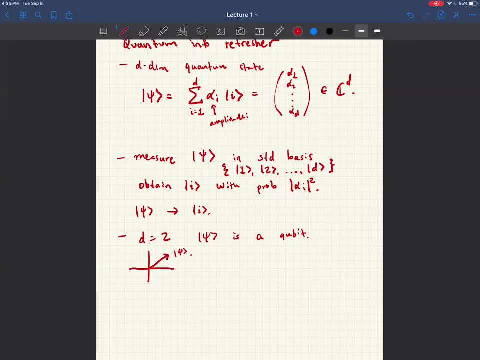 you know two dimensions. So this is our state psi. It's a unit vector And when you measure you're just projecting it onto one of the vertical or the horizontal axis. Okay, Of course we can. we don't have to measure in just the standard basis. 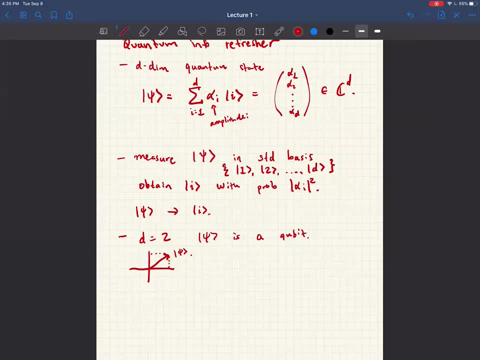 We can measure in different bases, And that corresponds to picking a different pair of orthogonal axes to project upon Right. So say you want to measure in different bases. And so in the two dimensional case, that would correspond to say measuring not along the horizontal and vertical axes but say on along this diagonal. 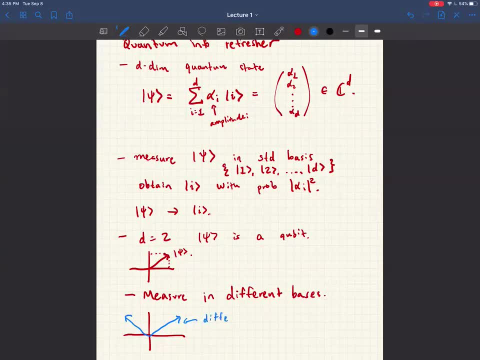 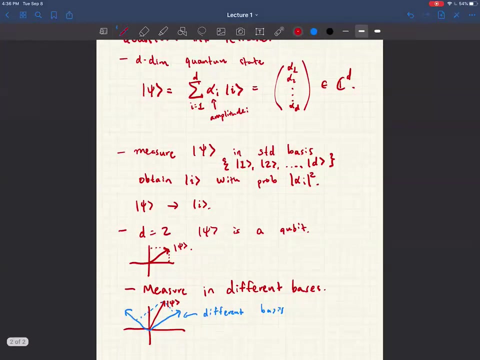 basis, Okay. And again, if you have some quantum state psi, this qubit psi, you're going to project it on the blue lines rather than cap simultaneously, So you're going than the red lines Okay, and the probability of getting a particular 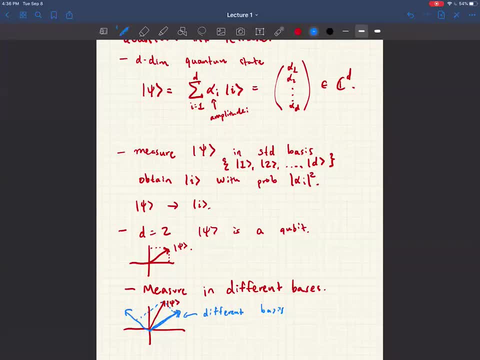 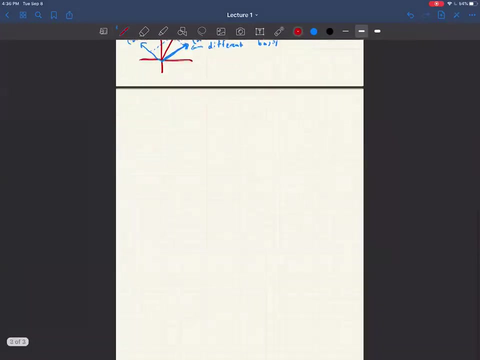 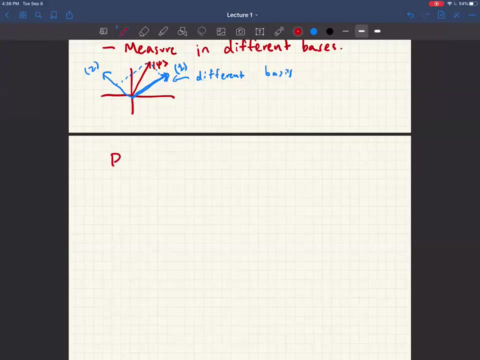 outcome, whether you get, you know this outcome. you know, let's call this outcome one or this outcome two. whether you get outcome one or two just depends on the, the length of the projection of your state psi on those, those vectors. So you know more generally. so more generally, like in higher dimensions, if suppose that you have an 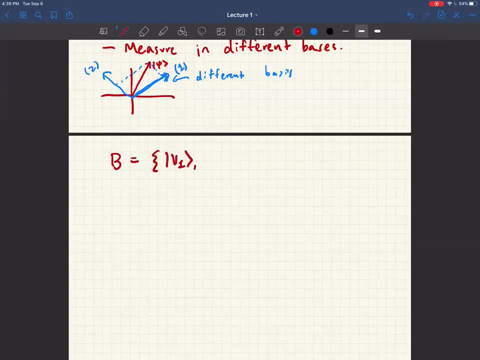 orthonormal basis of vectors. so v1, v2, up to vd. so this is an orthonormal basis for the space cd. Orthonormal meaning that all of these vectors are unit vectors. they're all orthogonal to each other. If you want to measure a d-dimensional 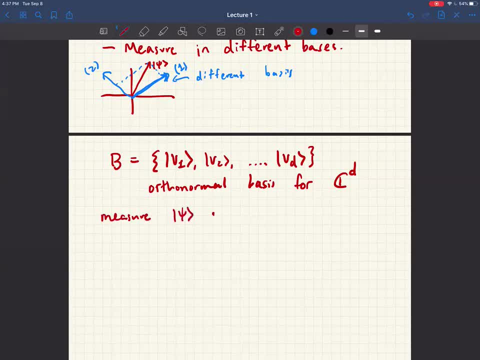 state according to this basis b, then you get outcome i. with probability, it's going to be the square of the overlap between the i-th vector and your state, Right, and here we're implicitly associating each, you know, v1 with outcome 1, v2 with outcome 2, and so on. 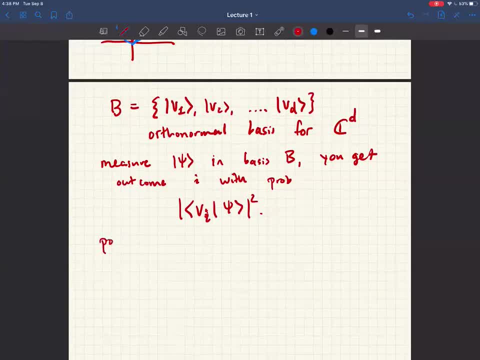 And then the what's called the post-measurement state, and here we have the same outcome. You know, the state psi will collapse to something. it's going to collapse to one of these, you know, whichever vector vi you got the outcome for. So the post-measurement state is going to be ket vi, and if you measure again in the 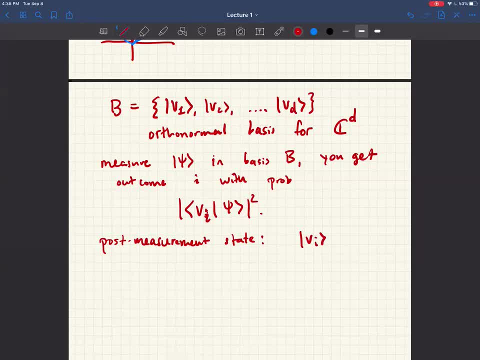 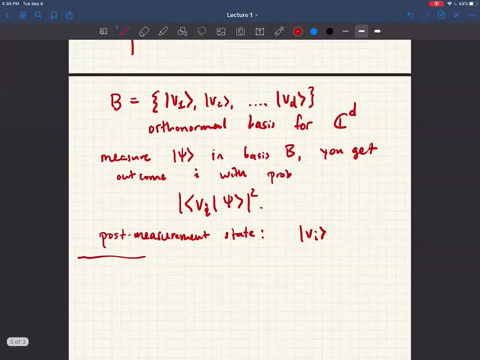 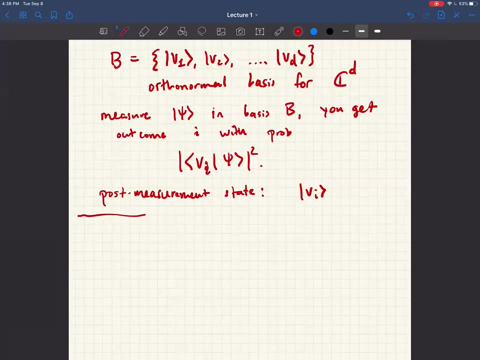 same basis, it's going to produce the same outcome with certainty. If you change the basis, though, then then again you'll you'll have another probability outcome. So that's, this is how you measure in a different basis. Let me generalize this just a little bit. You don't have to project onto single basis. 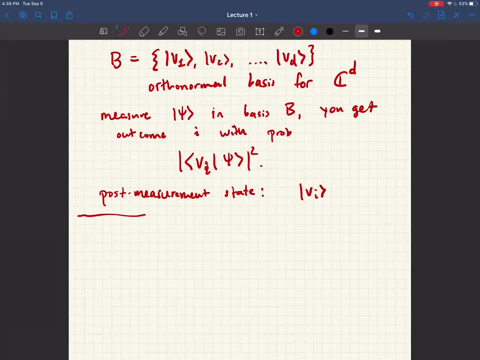 vectors. Sometimes you know you're working in d-dimensional space, but you want to make a measurement where you have fewer than d outcomes- Maybe you just have two outcomes- and the way to do this is you can group different basis vectors together into a single outcome and this gives rise to a projective. 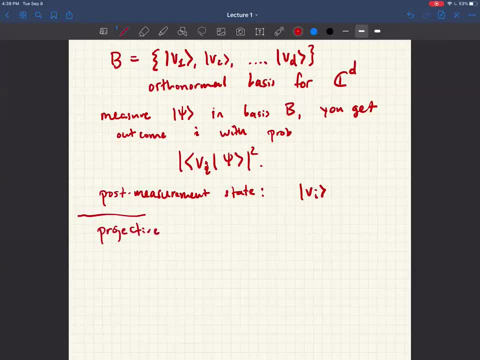 measurement, So a projective measurement, and if you know, if you're confused about anything, just feel free to unmute yourself and just ask. Sometimes I don't see the chat so I might miss something. Okay, so what do I mean by this? Well, I'm going to say a k-outcome projective. 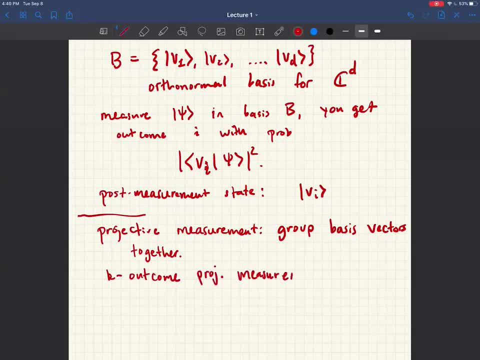 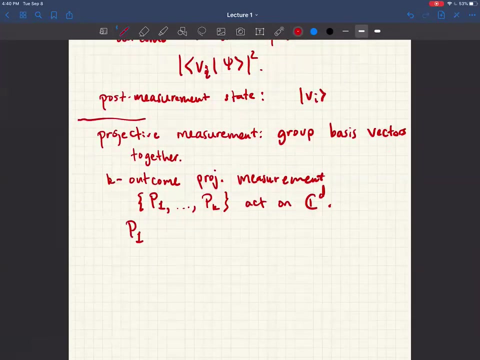 measurement. It's going to be a sequence of projectors, Projection matrices, Okay, p₁ up to p, Youtube, K. so these are matrices that act on C, D, So they're d by d matrices, they're projection matrices, They sum to the identity, okay So, and they're orthogonal. so if you take a, say, % of p₁ in thearden super种 database- And I'll come back to that in a moment, It's not or something un Gambin slightly created, Not going toorsa-s Crow, Okay, are sees only if the machine needs a TheraI 효ga loop, pain-yes. The projection matrices, they sum to the identity, okay so, and they're orthogonal. So if you take a, 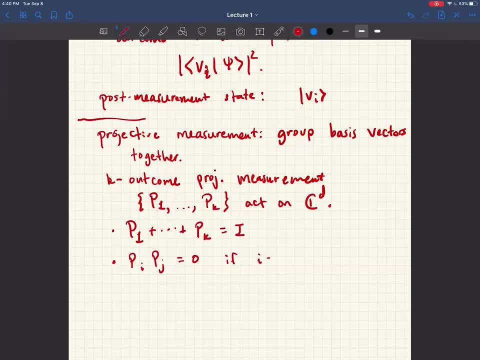 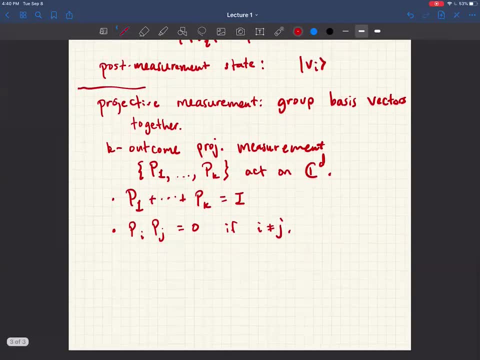 pi times pj, you're going to get zero if i is different from j. Otherwise, if you take pi times pi, you get pi Again. that's what it means for it to be a projection. So I walk up to you with: 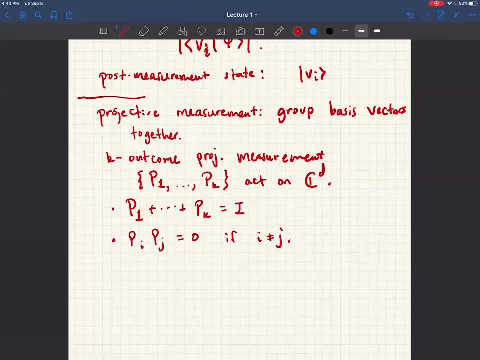 this set of projectors. there's k of them and it forms a measurement. If I want to do the measurement on a state psi, you're going to obtain an outcome. you're going to get outcome i. with probability It's going to be the norm of the projection. 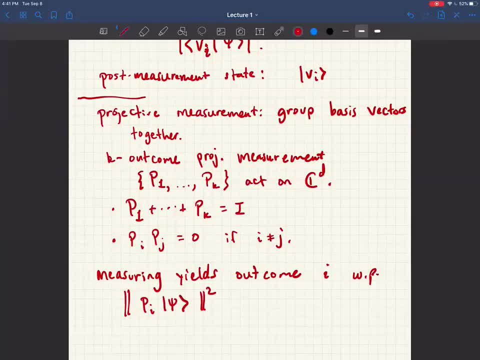 applied to your vector the squared norm. So you take your projection, you apply it to your state, you get a number, you get a. you know a shrunken vector. How long that shrunken vector is? that's going to be the probability. Another way of writing it is this is: 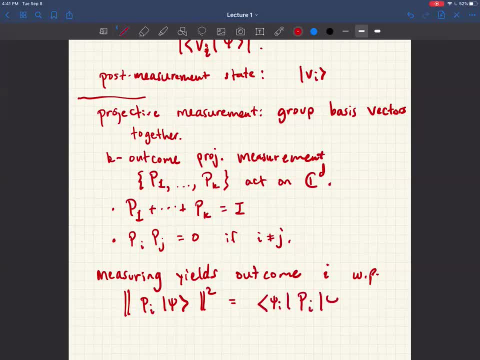 the projection matrix, pi sandwiched by- oh whoops, there's no, it's going to be pi sandwiched by the state psi. Okay, so this is a number right, because you have the transpose of psi, the matrix and the vector psi And the post-measurement state. 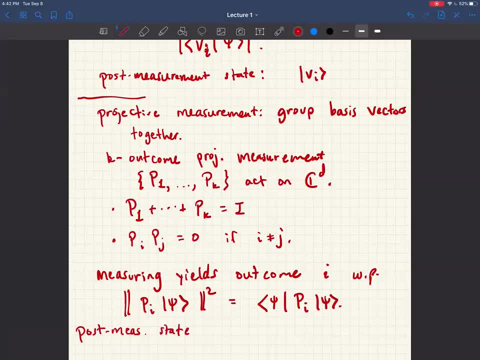 must be the same. So what does this mean? Well, you're going to take the projection and then you're going to divide by whatever this probability was. So this is. you know, this is a vector Right. so hopefully this should be a refresher of things you've seen before. 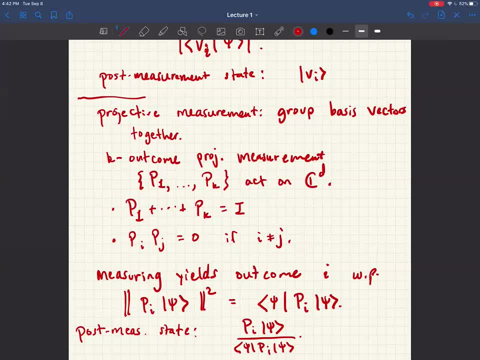 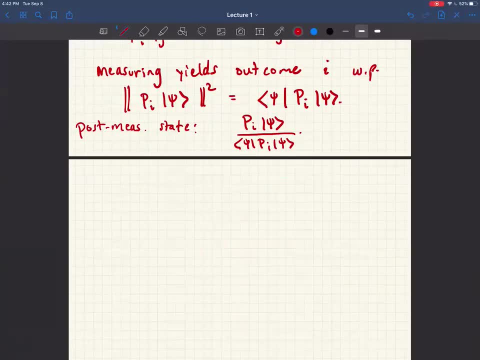 Okay. so now we come to something that will come up again and again in this class, which is describing measurements using observables. Okay, what are observables? Well, it's a convenient way of describing measurements. An observable is basically, it's just a Hermitian matrix. Okay, 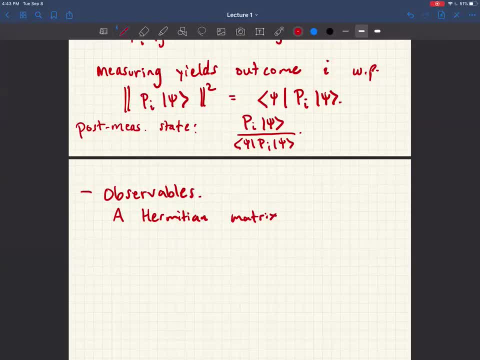 Hermitian means that the matrix is the same as its conjugate transpose. A is equal to a dagger, So how does it encode a measurement? Well, suppose you had such a Hermitian matrix, right, Observable, let me call it. let me call it M, So an observable M, Since it's Hermitian. 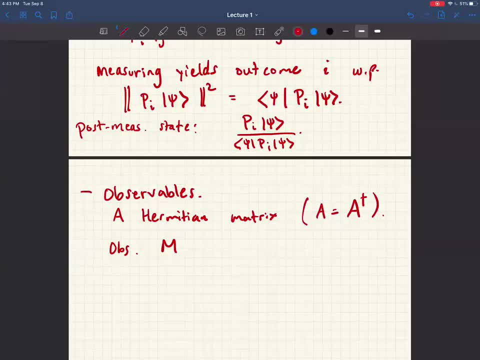 you know that you can diagonalize this, this matrix, right, So diagonalizable meaning that you can write it as the sum of 1 through k of some real numbers. lambda k times a projection- I guess it's lambda sub i times a projection: p sub i. 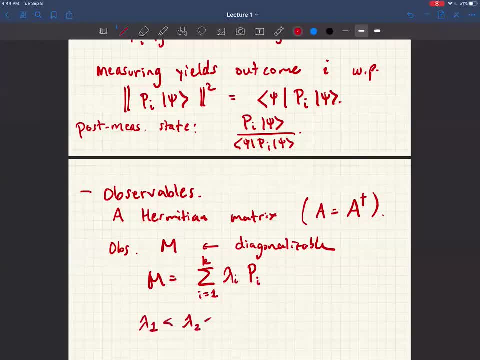 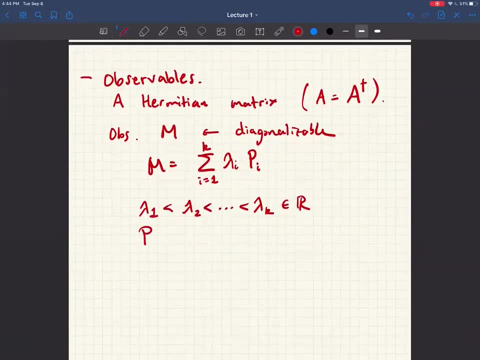 So the lambdas are all going to be distinct real numbers And the pis are projections, right, And the- you know, the lambda i is going to be the eigenvalue of this matrix M corresponding to the PI. so clearly, once you've diagonalized it and you've found all these, 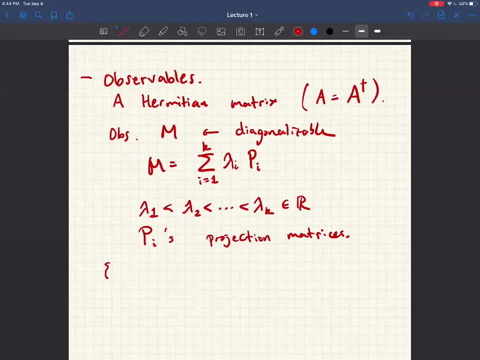 projections. they're all orthogonal. they sum to the identity, so it specifies a projective measurement, right? okay, what about these lambdas? what? what is their role? well, there there's some extra piece of information that's in addition to the, the measurement that you're talking about, and I think of them as weights. so 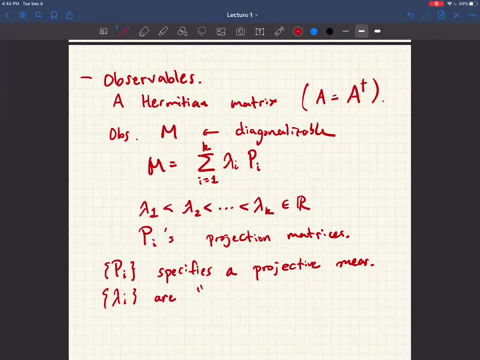 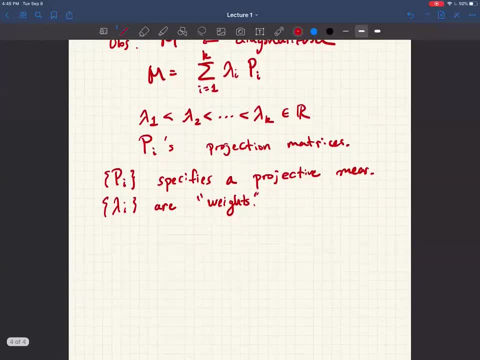 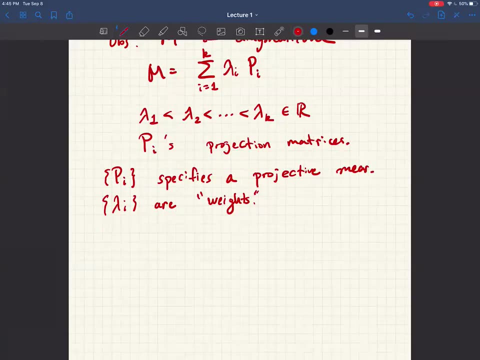 the, the lambda I's, are weights, and the way they they play a role is you can use them to calculate what are called expectation values of an observable with respect to a state. so if someone walks up to you with an observable M and a quantum state psi, then you can compute this number, which is the. 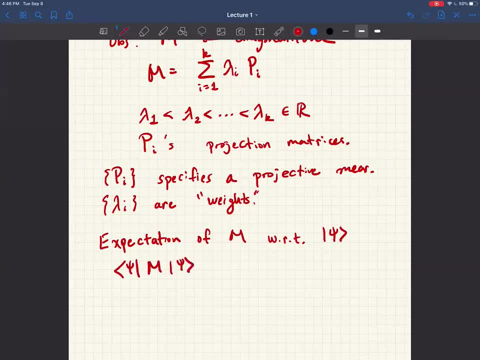 observable M sandwiched by psi. so this is going to give you a real number, right? and what does it correspond to? well, if you open it up according to its spectral decomposition, right, you're gonna have these lambda I's and then you're gonna have the PI's. 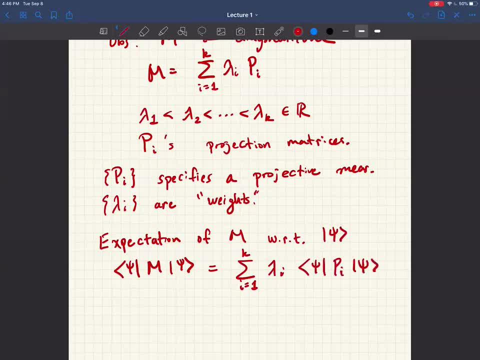 sandwiched by your state. Now we know what this number is right. This is the. this is the probability of getting outcome i. if you did this measurement corresponding to p, i. So it's like saying you measured the, the state psi, with respect to p, and then you, once you get an outcome i, you're going to output the. 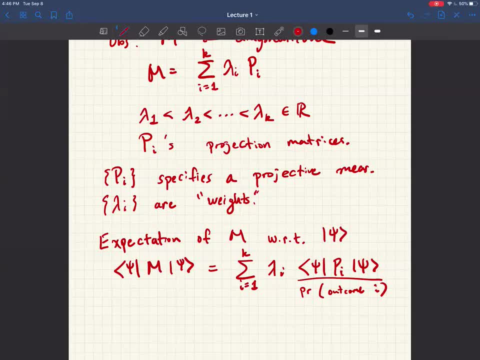 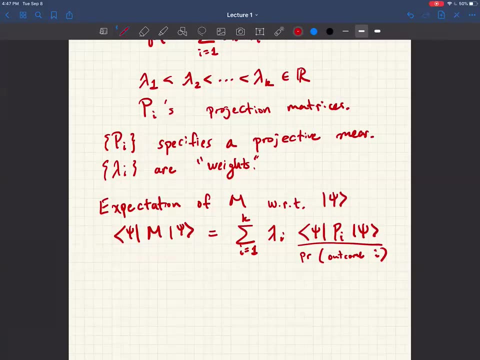 i-th weight, this lambda i. So this expectation value is going to be the expected weight that you output. Hopefully that should make sense. Now, why is this useful? Well, let's let's think about the, the qubit scenario. So let's go back to. D equals to 2.. 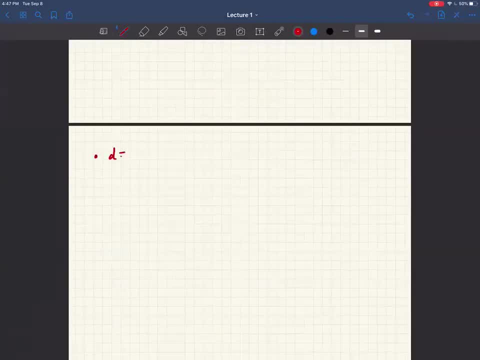 So let's say, you walked up to me with an orthonormal basis for two-dimensional space. So you had two vectors. I'm going to call them v0 and v1.. It's a basis for c2.. However, you're going to get a value of v1. 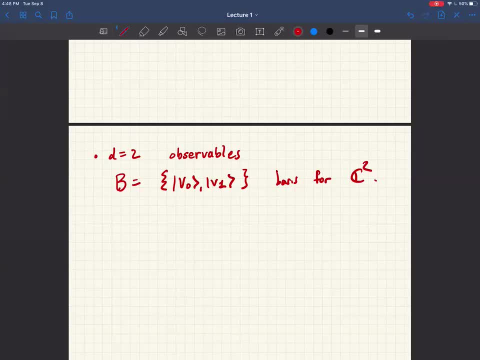 rather than carrying around this. you know these two vectors all. whenever I want to talk about this particular authors basis, I can instead package it into a single matrix. So I'm going to package it into this 2x2 matrix. Let's observe, We will call it m and it's going to be the 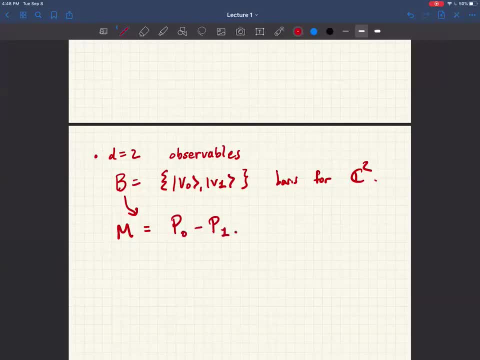 difference of two projectors. It's going to be p0 minus p1, right, And what's p0? is going to be the projector onto the basis element v0, and p1 is going to be the projector onto basis element v1.. Or another way of writing: it is you. 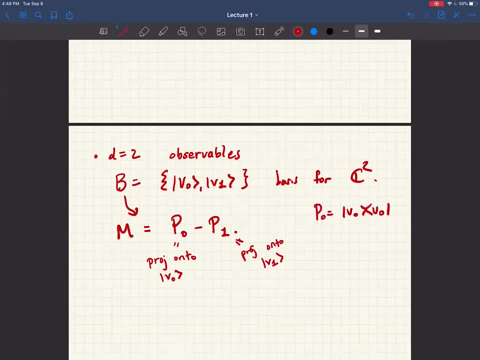 can write p0 as the outer product between v0 and itself. p1 is going to be the outer product of v1 and itself. You can see that the way I've defined m. it's a Hermitian matrix, so definitely corresponds to an observable and in fact, 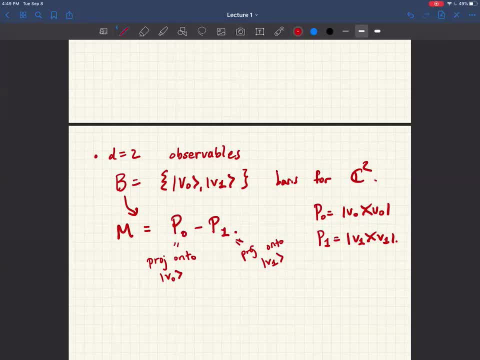 I've just written down its spectral decomposition, because p0 and p1 are orthogonal projectors and they sum to the identity. so that's something you can verify. Another thing to say about this, and this is kind of trivial, but the first basis, vector v0,. 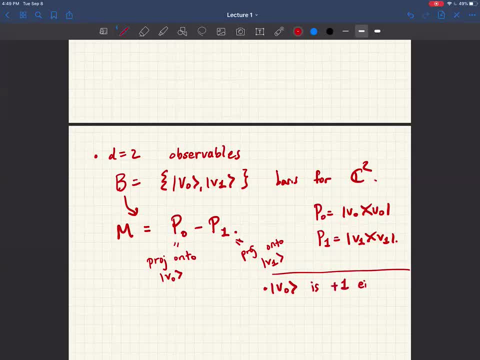 this is the plus one eigenvector of m, right, Like, if you take m, you multiply by v0, you're going to get v0 itself. v1 is going to be the minus one eigenvector of m, So v1 is going to be v0, and that's going to be the remaining one of the. 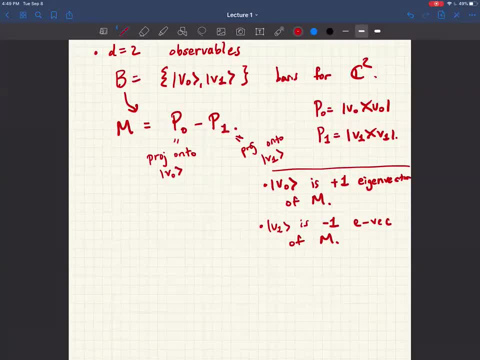 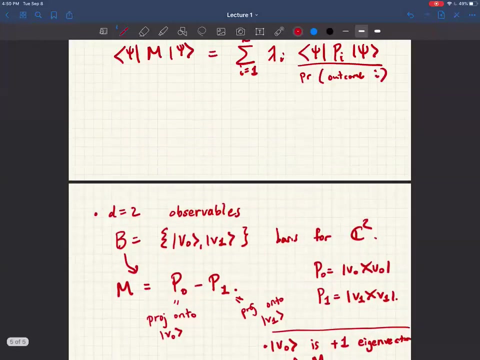 vector v0.. So to sum that up: m. And then let's go back to some other linear functions. So if you just write down that del-1, and you do that, you get a little bit of a clue here that if you do that, also gives you a little bit of a. 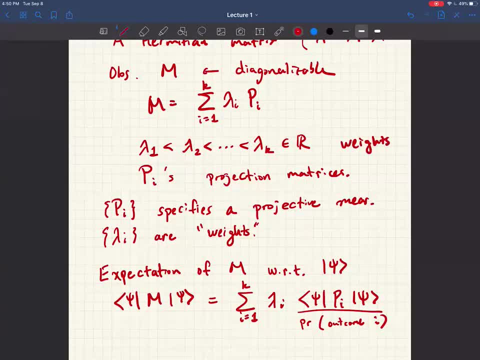 way to help you write down these measurements. Right? so the weights? I mean these lambdas. So here, M is a matrix, right? So M is the thing, that sort of talks. it encodes. this measurement has nothing to do with a state. 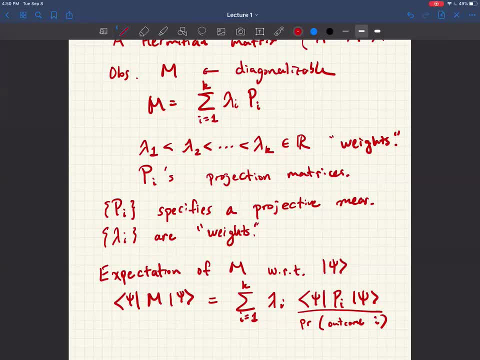 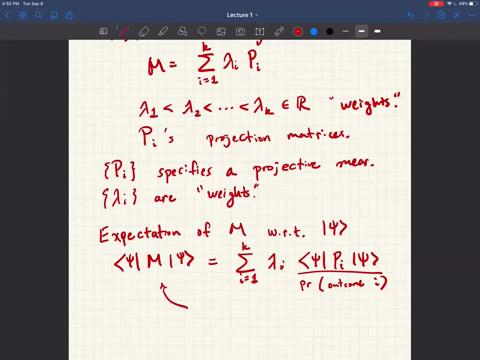 doesn't talk about a state yet. But you take this observable M and you diagonalize it, you get all these eigenvalues, these lambdas. those are the weights. Does that make sense? And what this expectation value is? it's average weight if you measure according to. 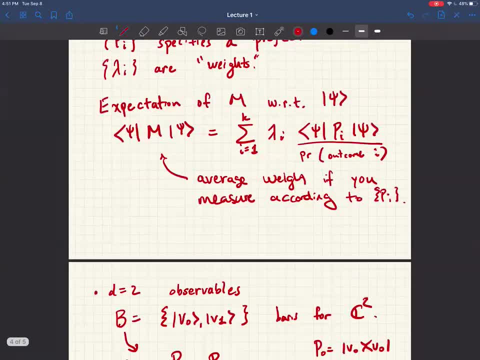 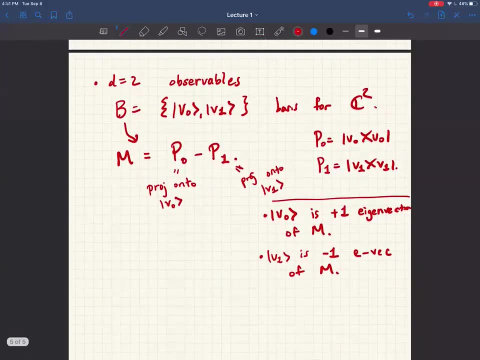 So, just to be pedantic, expectation values are a function of both observable and a state. okay, If you don't talk about a state, then it doesn't make sense to talk about an expectation value. Good question, Okay. so yeah, I've taken this basis B. 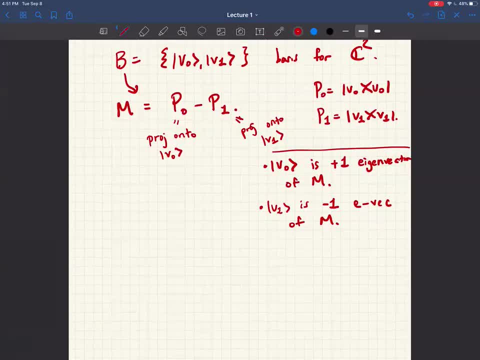 and I've neatly packaged it into one object, this two by two matrix, M. So M is a two by two matrix And let's say I walk up with a qubit. So Psi is some arbitrary qubit And I want to know what is its expectation value. 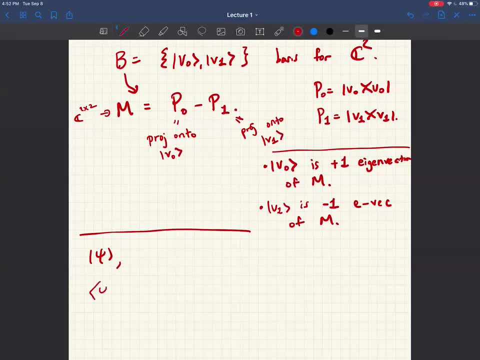 with respect to this measurement M in the way that I've defined it here. So Psi is a qubit. its expectation value? well, just expand it out. Well, it's going to be P0 sandwiched by the state minus P1 sandwiched by the state. 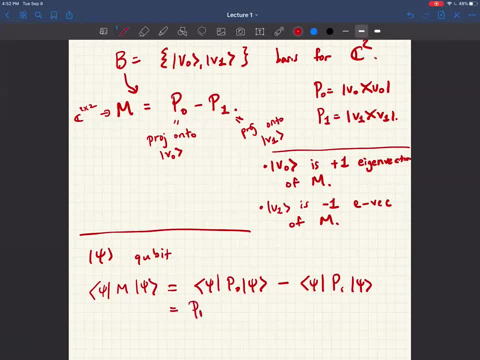 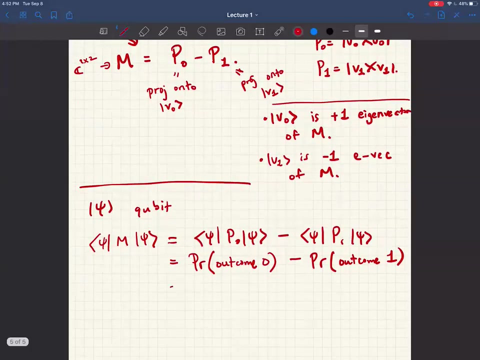 Well, we know what P0 is. This is the probability of obtaining outcome zero if you measured in this basis, minus the probability that you get outcome one. But we also know something else about these probabilities. Does anyone know like? what's the relationship? 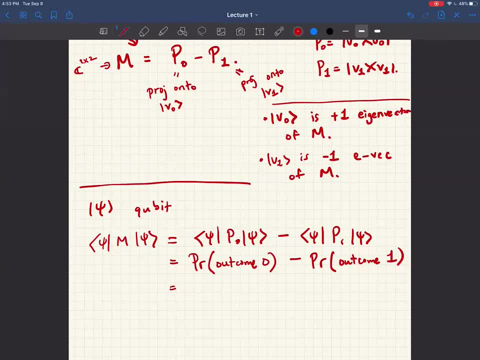 between these two probabilities, They sum up to one. They sum up to one, exactly right, Because you either have outcome- oh great. They either have outcome zero or outcome one. So if you use this relation, then you get you know. 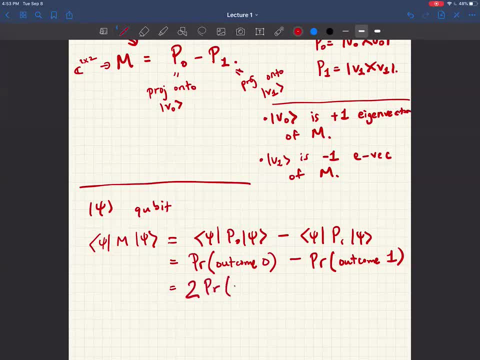 that this is also equal to twice the probability of outcome zero minus one, or equivalently, it's one minus twice the probability of outcome one. So for qubit observables, this is like a really nifty formula to have like to relate expectation values of this observable. 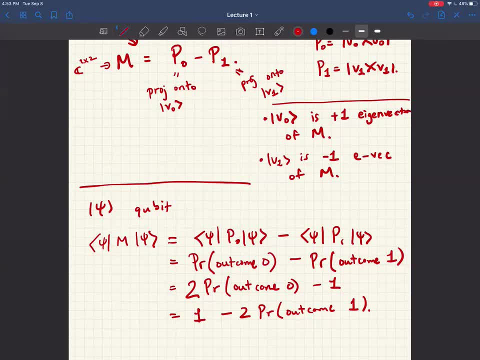 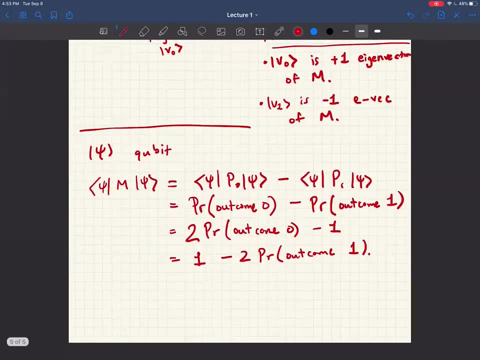 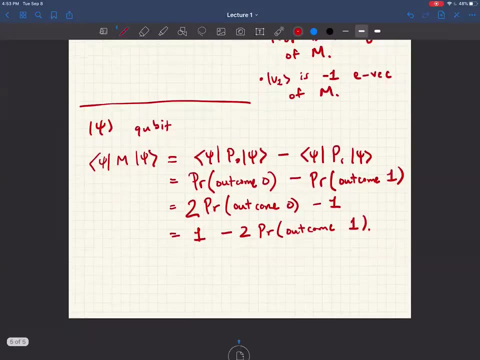 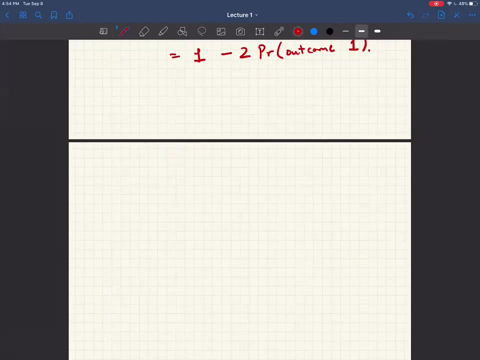 with probabilities of getting outcome zero or one, And we're going to see really quickly why you know this is a nifty tool to use. This brings me to an important class of qubit observables, the most important class of qubit observables. 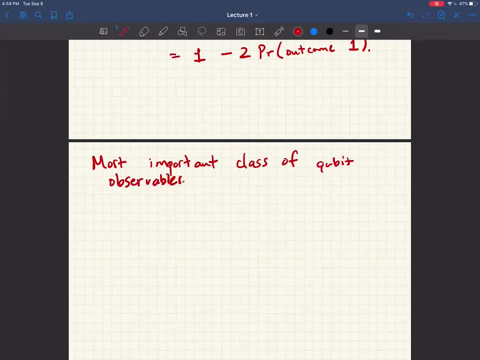 Okay, This one's going to be the identity matrix. There are these four matrixes. Probably a lot of you have seen these before. The first one's going to be identity matrix, You know the identity matrix is. And finally, the one that we'll rarely ever talk about, if at all. I mean, this might be the last time you see the Y matrix. 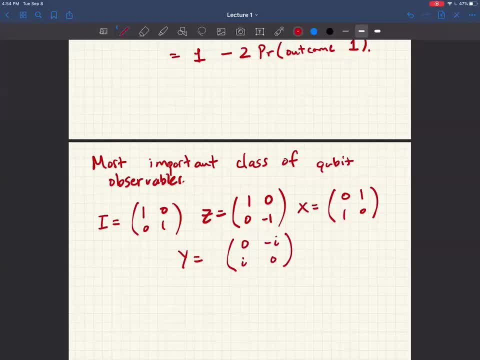 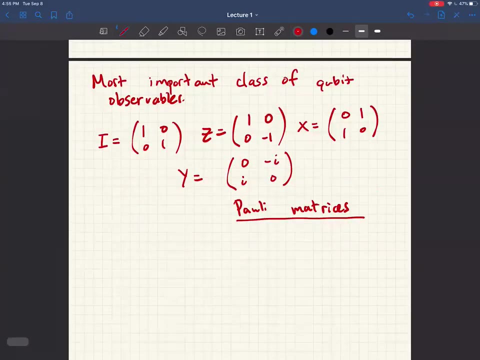 It's, It's this matrix here. Okay, so these are called the Pauli matrices, Named after the physicist Wolfgang Pauli. And why are they so important? Well, they have a lot of really nice properties. You know they're the nicest two by two matrices you'll ever see. One is they form a? 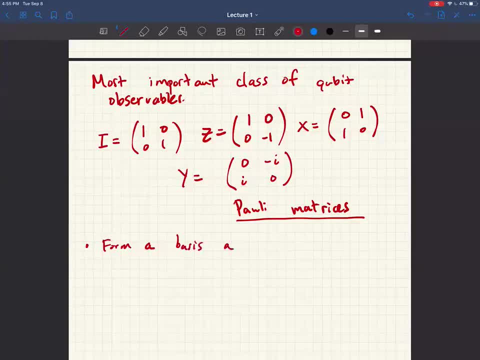 basis for all, two by two. matrices. Basis for: Okay, they are unitary, meaning that if you take their conjugate transpose that's the inverse of these matrices: They're Hermitian. Okay, They have. they each have. well. 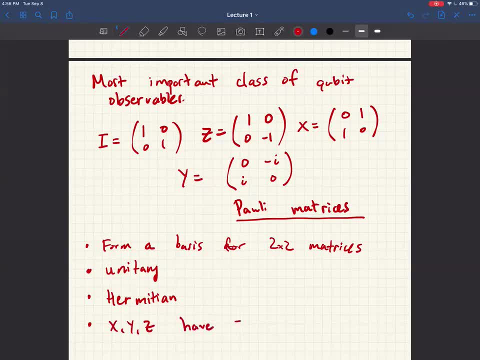 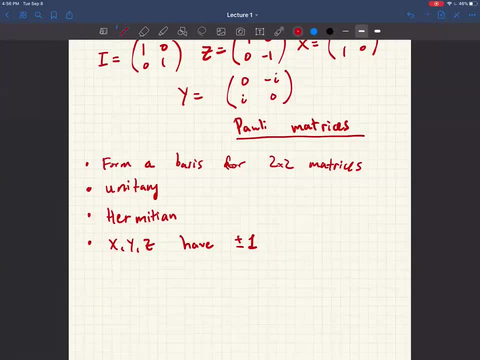 X, Y and Z have eigenvalues plus and minus one, Right? so they have one plus one eigenvalue and one minus one eigenvalue. They square to the identity, Like if you multiply them by themselves. Right, I mean, these are simple properties, but they're important. 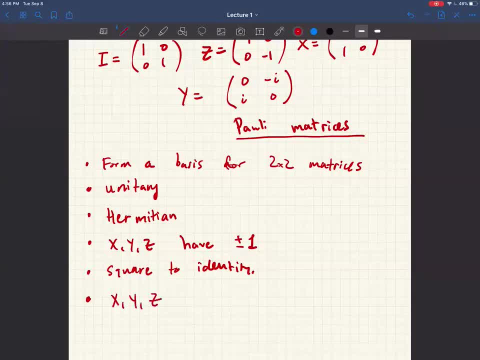 And importantly, X, Y and Z, all pairwise anti-commute. Okay, so a question: Shang-Yan asks for two by two matrices. are you referring to real matrices? No, I'm referring to complex ones, Yeah. 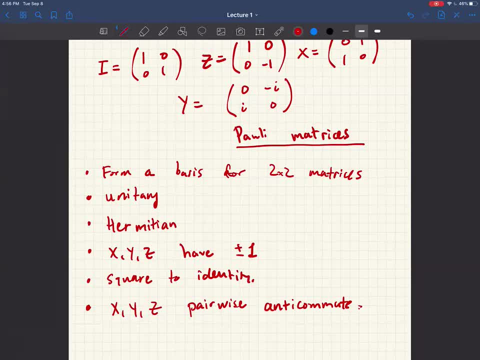 Any questions Waleed is asking. do I mean the basis of Hermitian matrices? No, not necessarily. If we take allow complex linear combinations, Then it doesn't need to be Hermitian. Yeah, I believe there's quero. 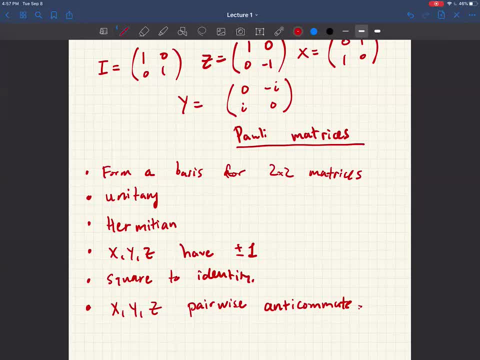 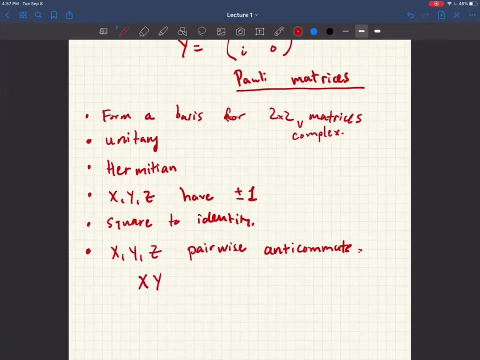 nothing else. Right, they're the. yeah, they should be a basis for all complex two-by-two matrices. Yeah, Okay, hopefully that makes sense. So what I mean by parallelized anti-commute? I mean that if you multiply, say x times y as matrices. 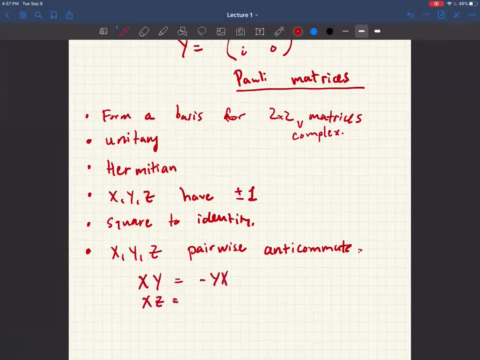 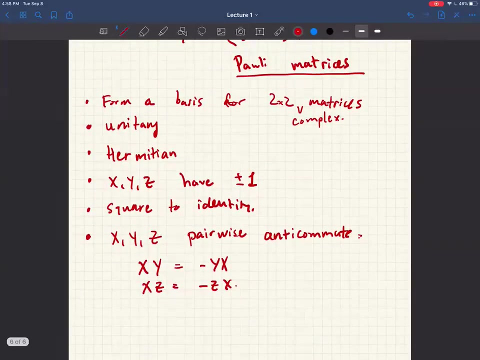 you get minus yx or x times z equals minus zx, and so on. This anti-commutation is super important. We'll see it come up again multiple times throughout this course. Okay, so maybe let's do a quick pop quiz. 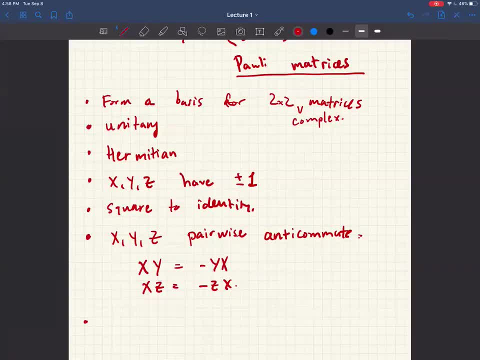 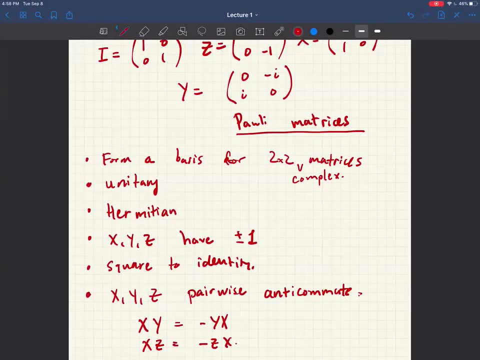 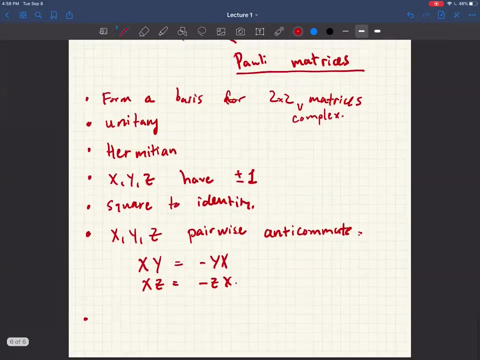 So I've described these really nice two-by-two matrices. They're Hermitian right, So in particular they're observables, And I've just told you how observables are packagings of projective measurements. So what measurement does the observable identity? 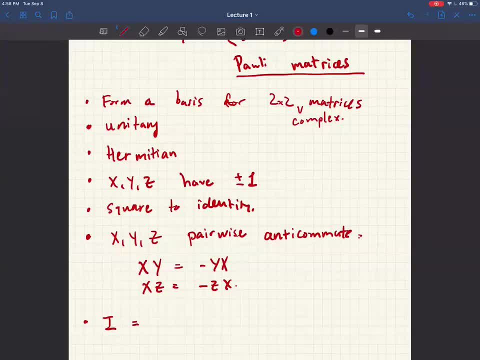 correspond to Like: yeah, what are the projections? So this one's the easiest, Same as the original ones. I guess what I'm asking is like what's? yeah, it corresponds to some measurement, right? So if you diagonalize it it's like: well, maybe if you add: 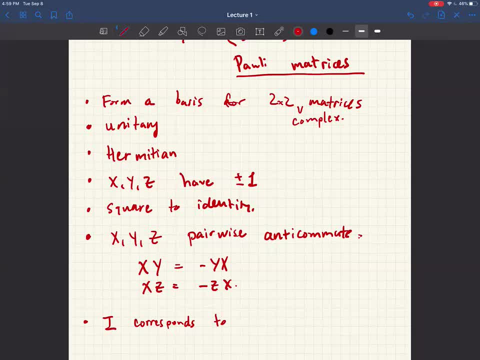 it. you're going to get projections onto what basis? Okay, Hao, I think, almost has the right answer. Great, So Waleed says it's projections onto x-axis, projections onto y-axis. That's absolutely correct, So we can write it as projections onto this. 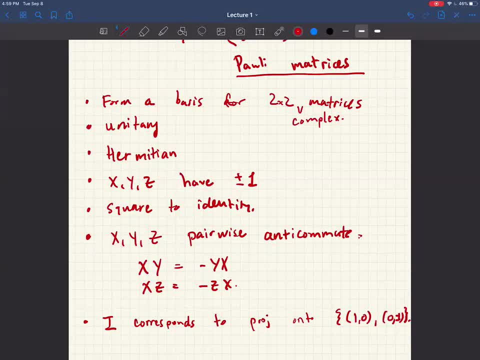 particular basis, but of course identity is diagonal in every basis, So you could have written any, you could have written any orthonormal basis here, right So? but it's, but it only has one plus one eigenvalue, so it only has one outcome: that. 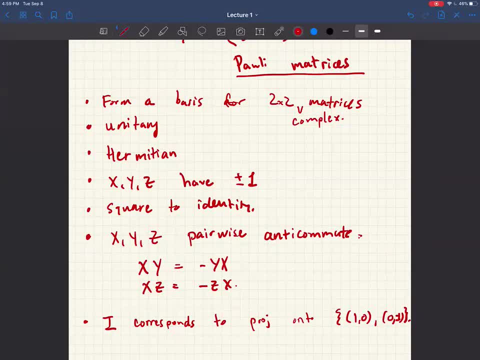 ever occurs Like. if you measure the observable correspondent identity, you're always going to get one outcome right. That kind of makes sense. Identity shouldn't do anything And it's not going to change your state. The post measurement state of the. 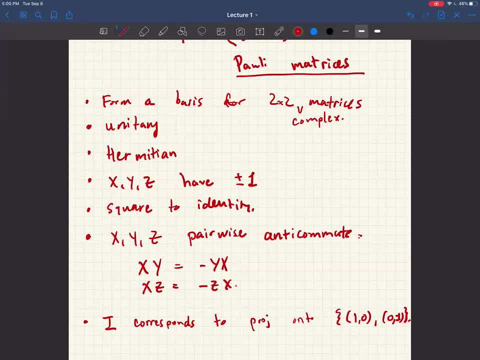 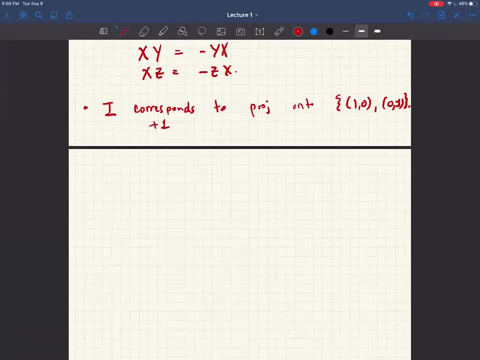 identity measurement is just the state itself, So that's maybe a bit trivial, but that's that's what it is. It only has one plus one. We call it the plus one eigenspace. All right, Let's see the more interesting. 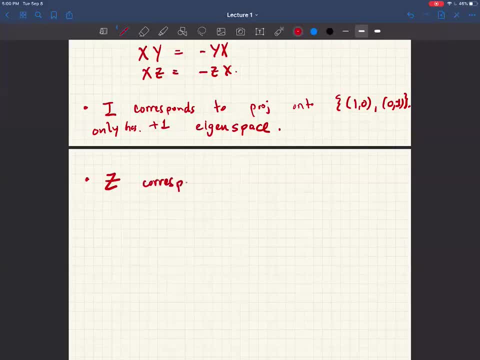 of the three. let's see Observable. so the, the Z observable corresponds to what? measurement? X and negative y-axis? It's a Hold on. I want to make sure that I say the right thing here. The answer is yes and no like okay. so here's a. I guess one thing I should mention is that 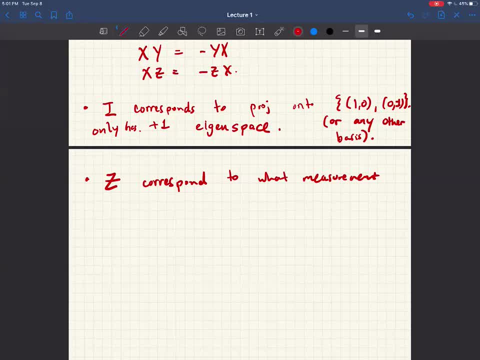 When you talk about the negative y-axis, you mean, like the, the vector 0 minus 1, right, You Actually get who is who asked this question? I did Yeah, Yeah, so. so one thing about quantum states is that you know they're their unit vectors. 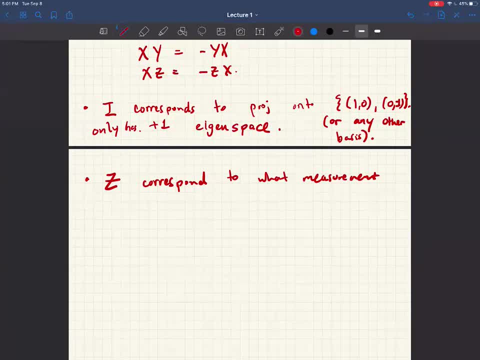 You can multiply these unit vectors by any like say plus minus one or any complex Phase, and that technically doesn't change the state. So we actually kind of consider all of those vectors the same. So it's- it's going to be-. so Abhinav writes it's. 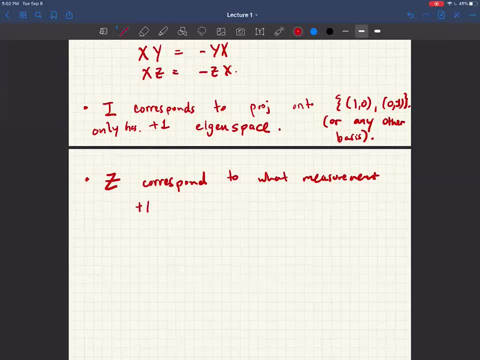 plus one- so the- the plus one eigenspace is the projection onto the x-axis and sort of alluding, like to tie in what Kyle was asking earlier. this also could have been projection onto the- the minus x-axis, It's actually all the same It. 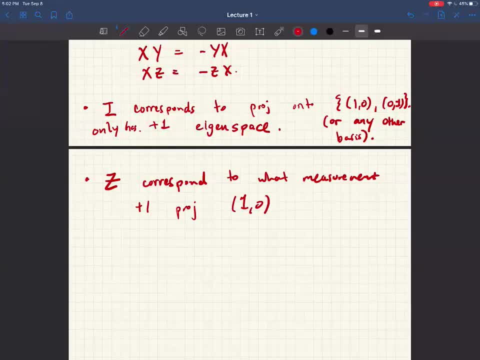 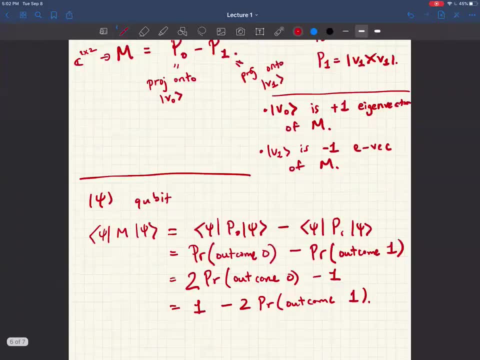 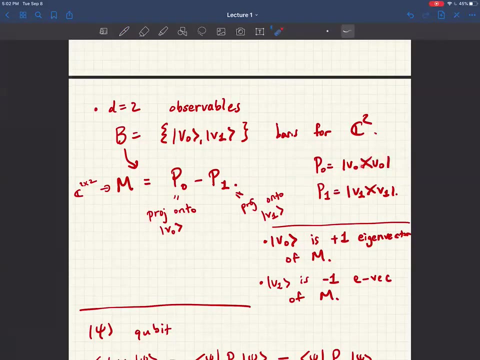 doesn't- mathematically, it doesn't change the operator, because when you multiply- and when you're taking these outer products- this is kind of an aside, but you know these outer products here- if you put a minus sign on this vector, it gets cancelled out by a minus sign here, So- so. 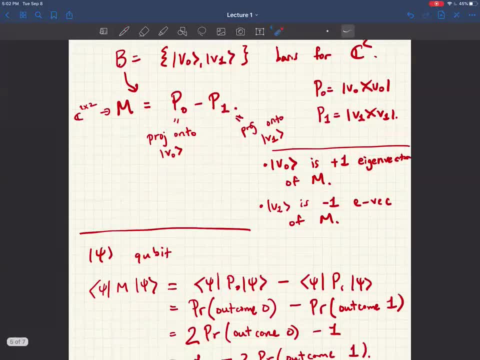 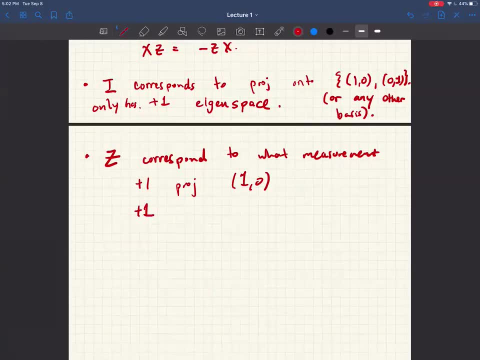 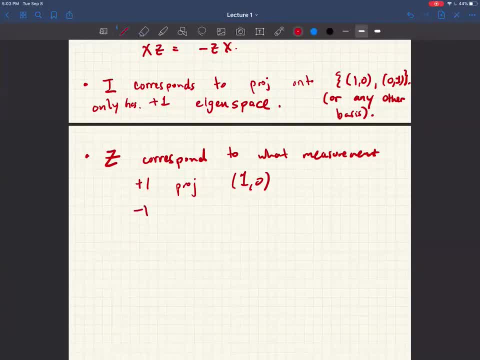 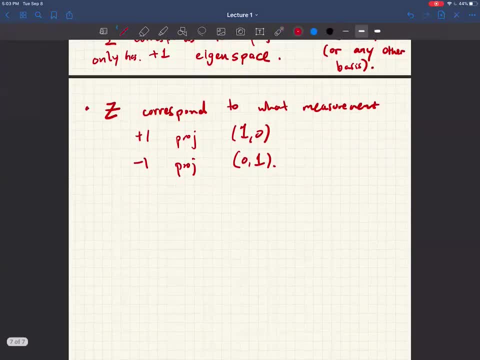 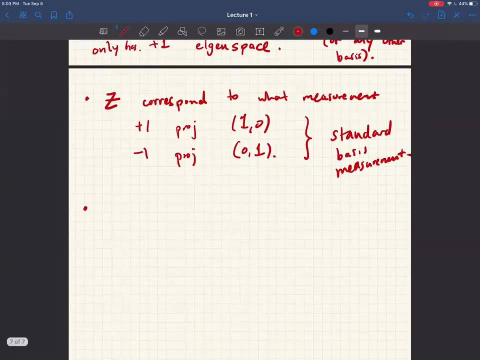 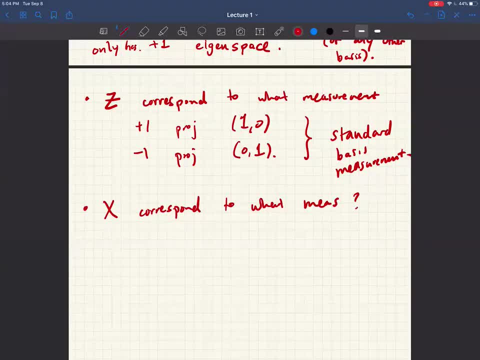 So remember, x is this anti-diagonal matrix and we- we want to uh, diagonalize it. Okay, uh. Sajjad says it is plus one eigenvector onto the plus state, so projection onto the plus state. Well, what's the plus state? It's the equal superposition between zero and one, exactly, and it has the minus one. 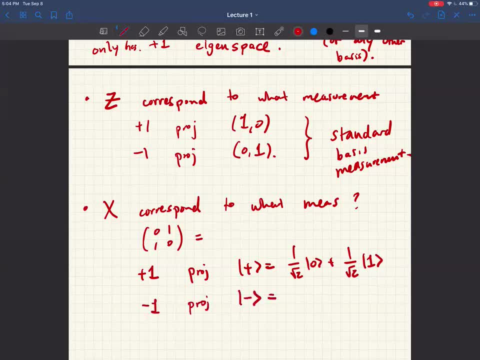 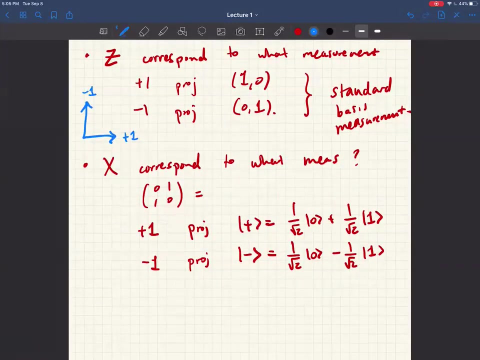 eigenspace, which is the projector, onto the minus state, which is the same thing, except you have a minus between these two states. So just to draw out, this is this basis, this is plus one and minus one outcomes, and here, for the x, we have a project. 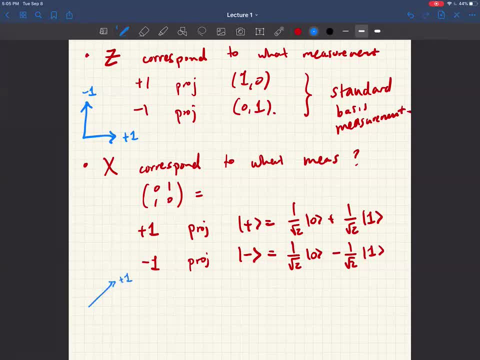 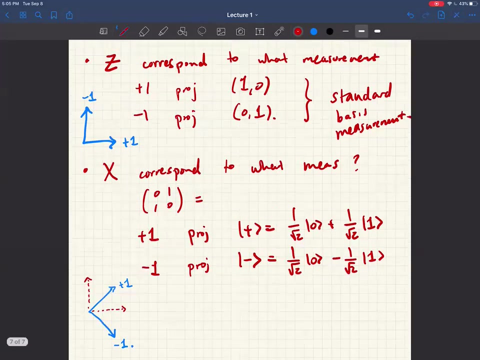 let me make sure I get my drawings right. this is the plus one axis and this is the minus one axis, And we won't talk about why because it's not not important. Really, the most important poly matrices we'll ever talk about are z and x Standard basis and this diagonal basis. 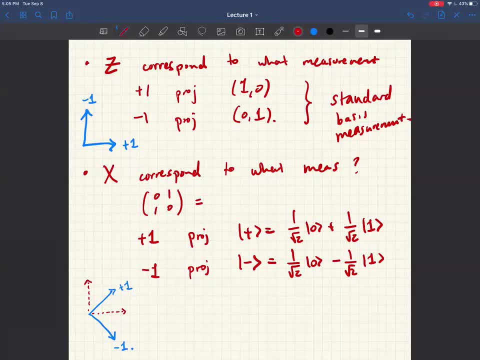 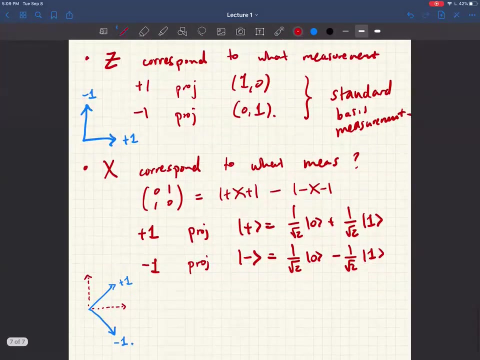 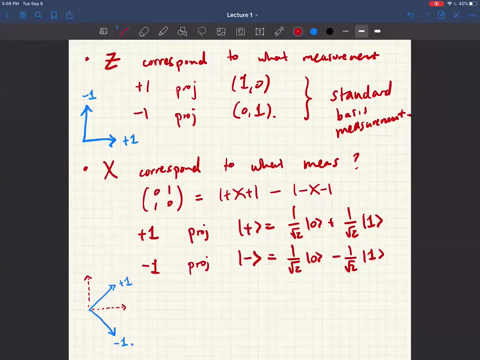 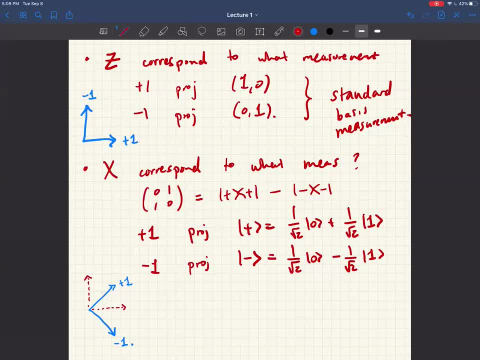 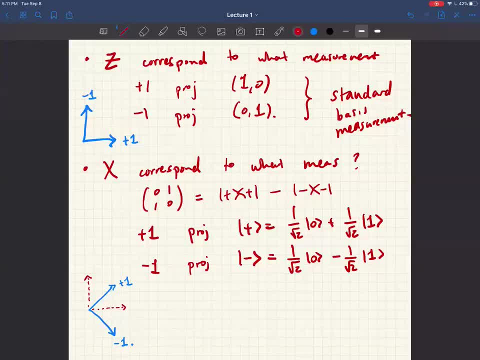 Oh, so yeah, plus and minus, the plus and minus states are different. So the 0, 1, 1, 0 are the. I'm going to write it here. So 0 is this. You can see what I'm writing, right. 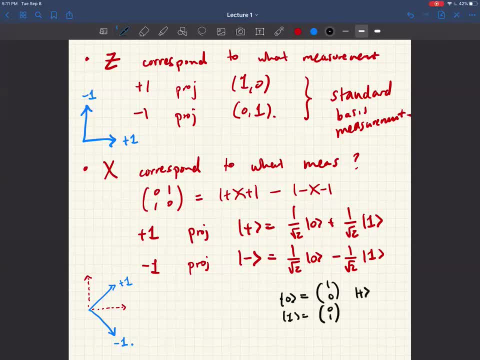 Yeah, And the plus states and minus states are the diagonal ones, So it's going to be like these ones. Oh, So that's how they're defined. Okay, Got it. Thank you, Yeah, Cool, So let's come back. 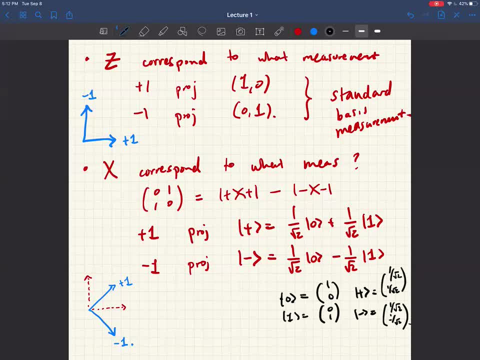 All righty. So we talked about. what did we talk about? We talked about measurements, talked about observables. We saw the most important qubit, observables X and Z, Identity Y- I don't think we'll ever talk about. 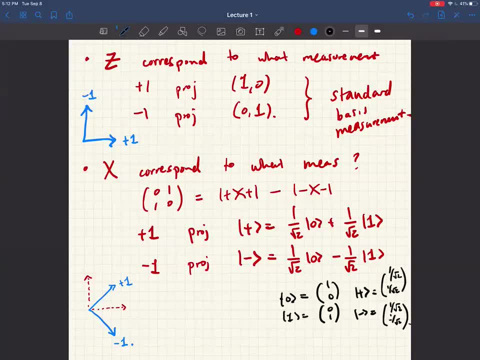 So we talked about. what do we talk about? I can't remember. And you're right. the last one. Is there anything else I need to mention about those? Okay, Yeah, So if this is going a little fast for you, then you can take a look at say: 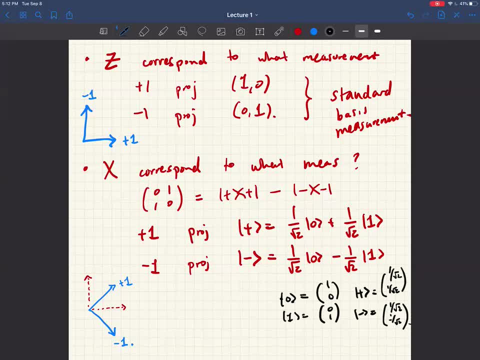 Ronald Bolt's lecture notes, or actually there's lots of different resources. You can go to my website. I have a page that's called resources and it has links to different lecture notes. So different ones appeal to different people and hopefully one works for you. 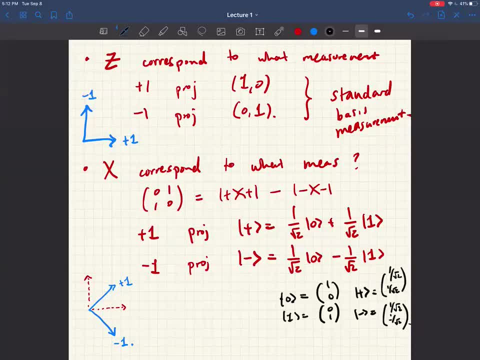 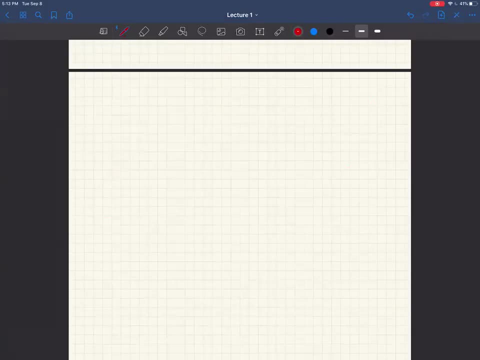 You can use that as a way to Refresh yourself or get caught up on some of this. Alrighty, Let's talk about The Heisenberg. uncertainty principle Is a good place to for it to come in. Oh sorry. And then she had a question: Is it projection operator linear? 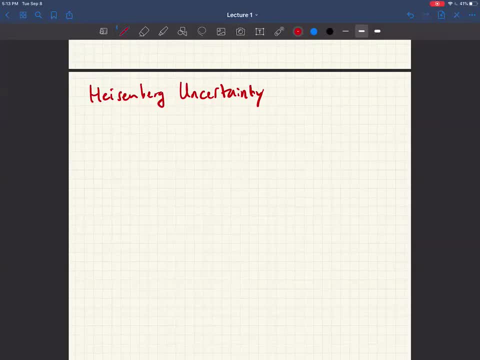 It is linear. It seems linear from Phi, P Phi, but not from the norm of P Phi. Oh right, So the projection operator has the property that if you multiply it by itself, So P squared is equal to P. So does that answer your? So maybe that is that answer your question. 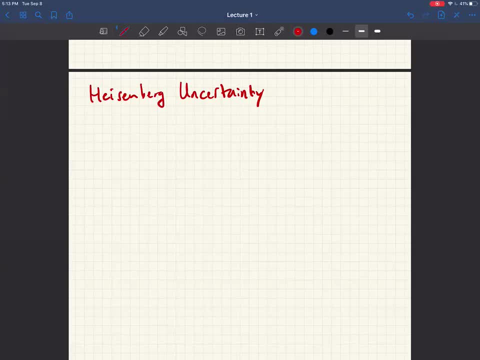 You know, also free. Yeah, feel free to unmute yourself. It's sometimes easier to just chat over voice If it's convenient for you. Okay. so if that makes sense, then we'll continue on. Okay, Heisenberg uncertainty principle. 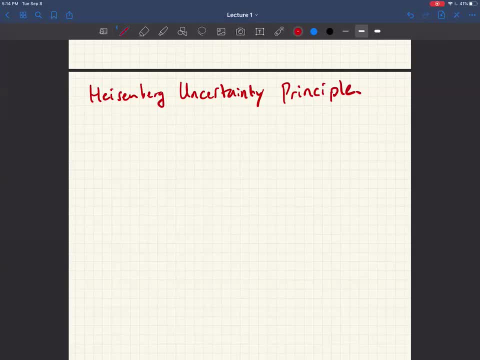 You know. it's this. this thing Maybe a lot of us have heard of, comes from quantum physics. It says that you know At a high level. You can't know the position and momentum of an object simultaneously, right, And you know. in quantum information theory terms, This boils down to the following statement is that if you take a quantum state, 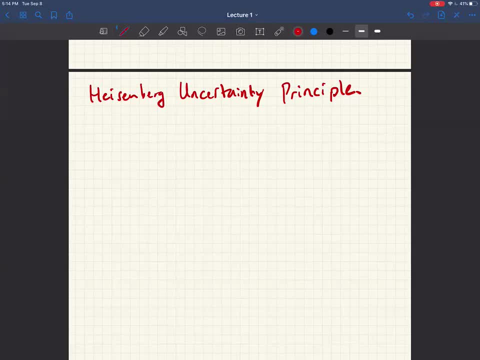 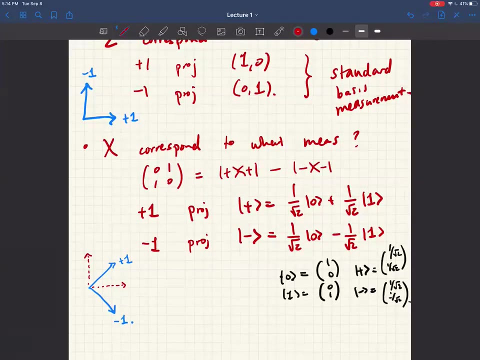 And You can't. you know this quantum state cannot be simultaneously determined in two different bases that are incompatible. So, for example, two bases that we've just seen is one, is this: the standard basis, the 01 basis and the plus minus basis. These are incompatible bases because you know they're they're like, not aligned with each other. 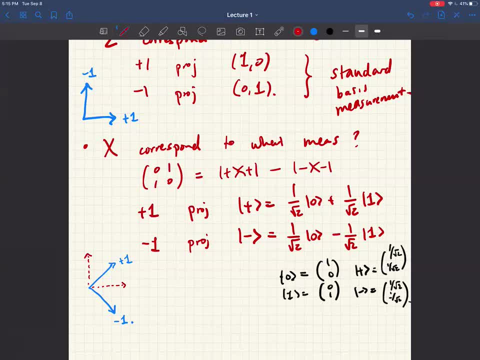 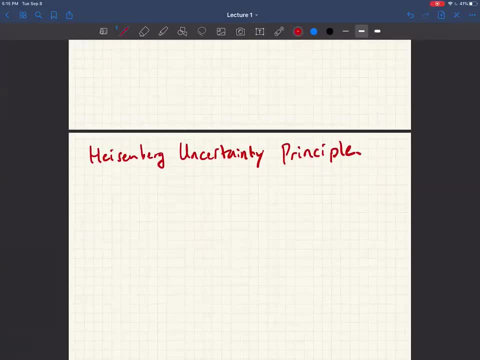 And what does it mean for a state? you know, the Heisenberg uncertainty principle says that if you have a, Let's say, a qubit size, So let me, let me draw the, So you know here, Here's our, our state side. 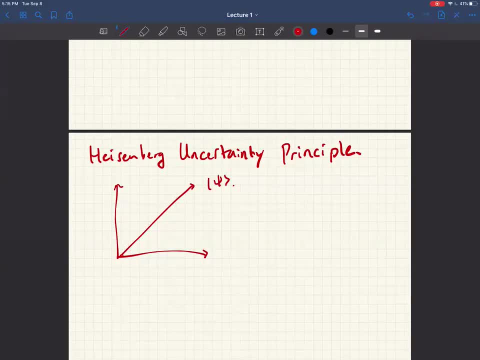 Suppose that it were determined in the The X basis, Right. So that means it's perfectly aligned with, You know, With this X basis. So this is the plus state, This is the minus state. So if you measured in the X basis, you're going to get the plus outcome. 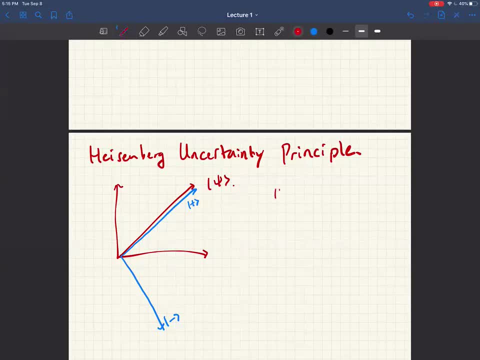 100% of the time, Right So? So si would be Determined According to the plus minus basis measurement. But now imagine you took si and instead of measuring in the plus minus basis, you measured in the standard basis. Well, what would be the outcome? 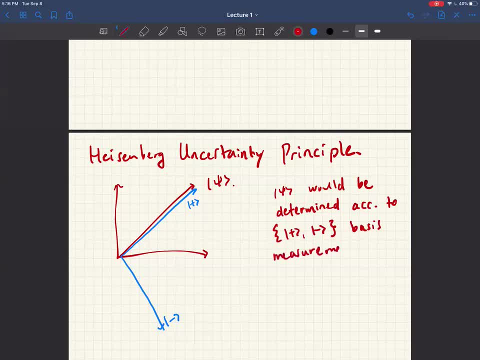 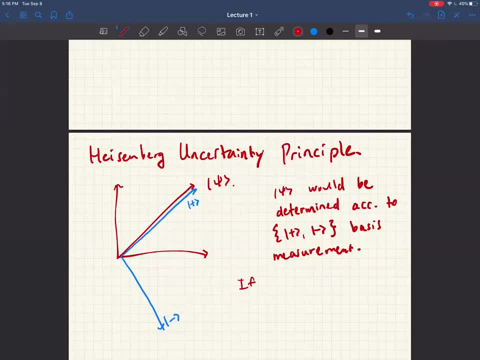 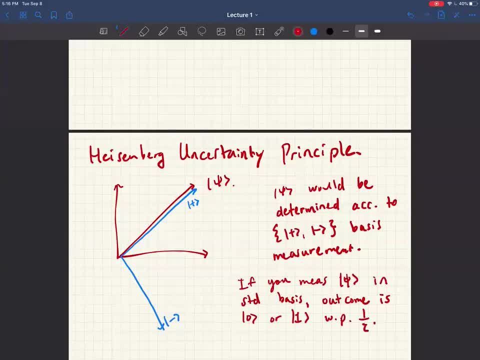 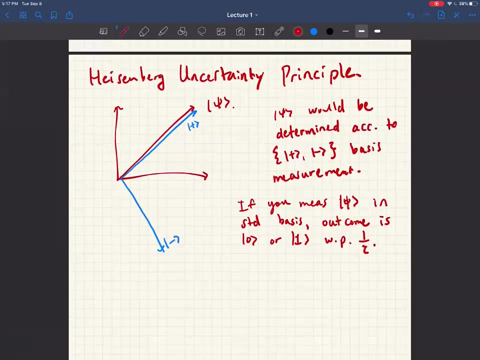 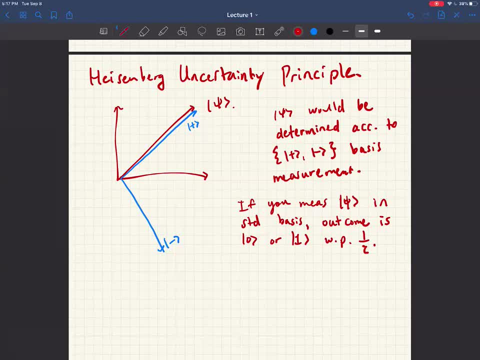 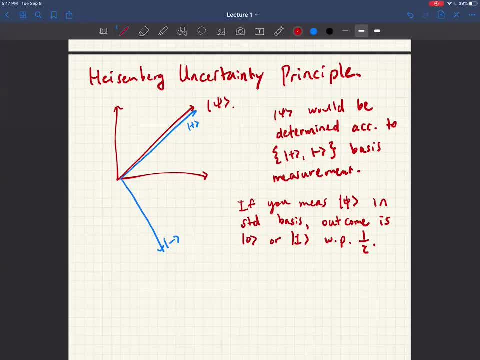 principle is saying that you know there's going. you know, when you combine the two uncertainties it's always going to be at least something. It's always going to be, at least you know, pretty uncertain. at least one of the bases, Another way of 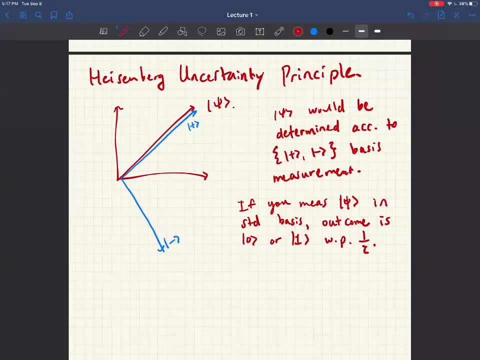 you know, seeing why this is true. this comes about from the fact that the observables- the z and x observables- don't commute, So it's a consequence. I mean, you can see, it's a consequence of the picture I just drew, right, It's like very. 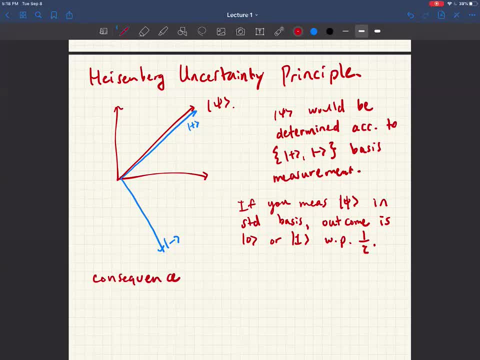 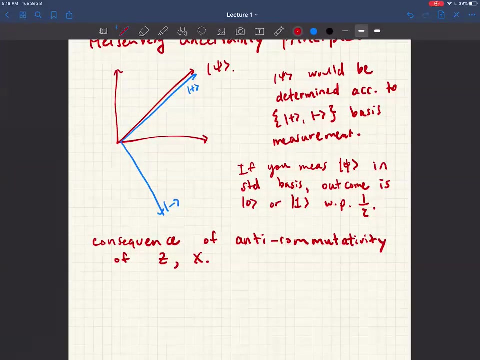 intuitive. But algebraically you can see it from the fact that z and x don't commute Anticommutativity, right. That's kind of a mouthful of z and x, right? So why is that the case? You know? suppose for contradiction that there was some qubit. 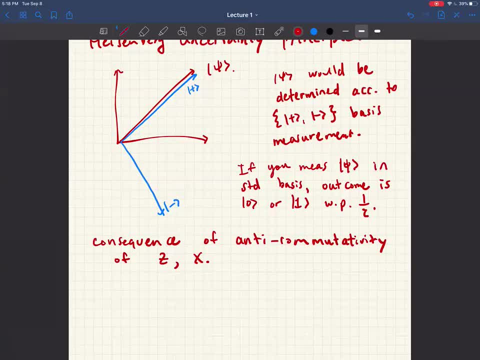 psi that was determined in both the z and x bases right. So if psi is determined, meaning that if you measure it in either basis you get the z and x basis right, You get one outcome all the time, like with probability one. What does this mean? 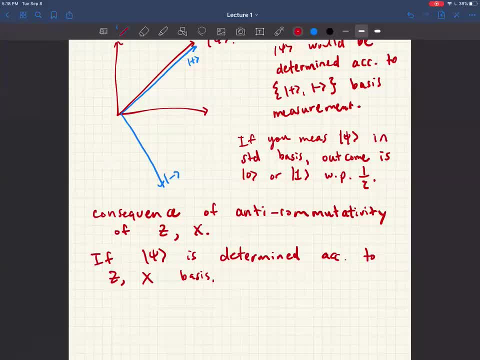 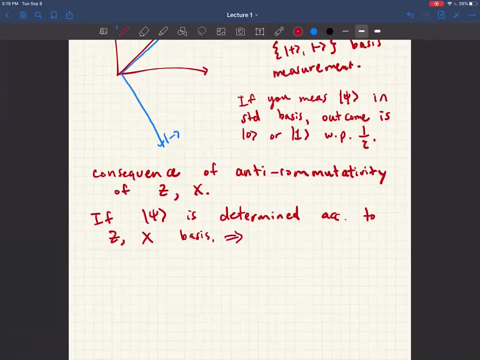 It means that the psi is going to be an eigenvector of these two observables simultaneously, Right? So, in particular, if you took z and applied it to psi, you're going to get some eigenvalue- alpha times, psi, you know- and this eigenvalue is not going to be zero, it's 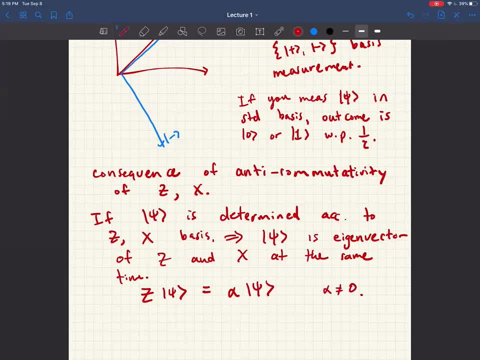 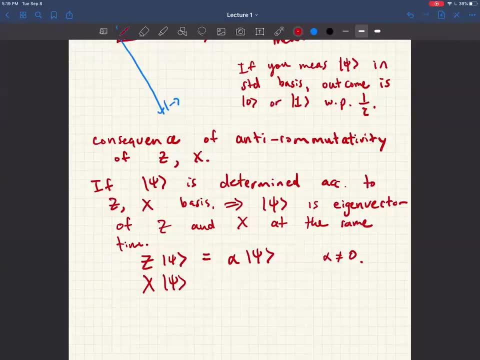 going to be plus or minus one. Oh, and then Juan, yeah, Juan had a, you know, guessed the answer: It's because they don't commute. If you had, you know, this eigenvector of x which was, say, eigenvalue, beta, beta is not all up to zero, but we quickly see this. 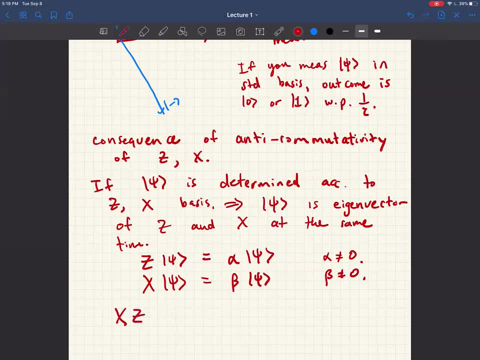 contradiction, right? So let's apply x times z to psi. Well, this is going to be alpha beta psi, right, Just from what I wrote above. But on the other hand, x times z as a matrix is equal to minus zx as a matrix, and this is equal to minus alpha beta times psi. But that would 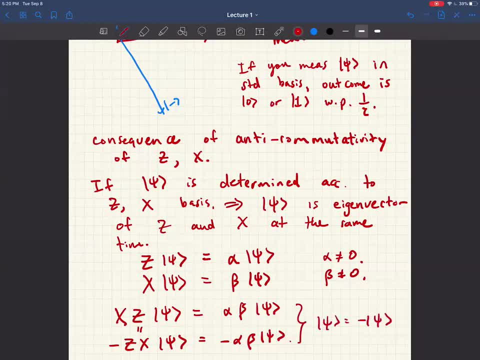 mean that psi is equal to minus psi, And that's only possible if, if psi is the zero vector, which we're assuming, it's not. So this is a contradiction, Sorry. so what is the precise definition of uncertainty? Good question. So here I'm using the most simplistic notion. I just mean that if you 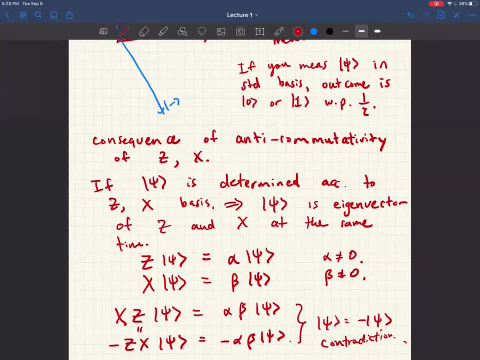 measure a state in some basis that there's some probability of getting both outcomes. Or to put it another way, if there's no uncertainty, it means if you measure in a certain basis, you're always going to get the same outcome with 100% certainty. 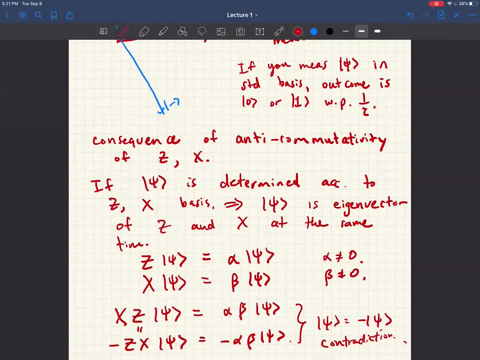 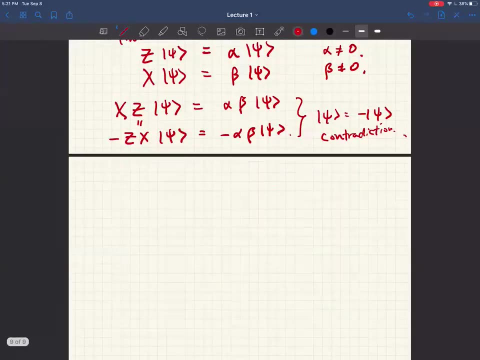 Okay, thanks. So you aren't making the technical right, Not a precise formula. let's say, for uncertainty, Yes, I, you know the more precise statement would be: you know that if you measured, let's say, in the X basis, 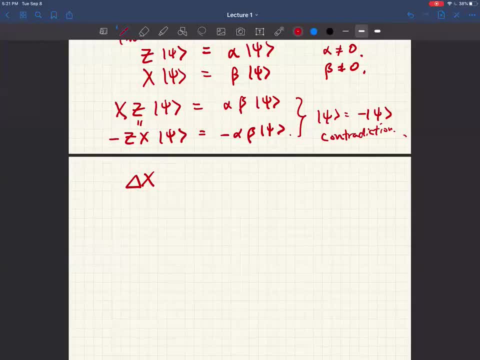 you get some, say, some variance or some standard deviation that's measured by Delta X and you multi or you compared it. if you measured in the, the Z basis, you get some deviation. then this deviation is lower, bounded by some constant that's greater than zero, and that's that's sort of the technical statement of the, the. 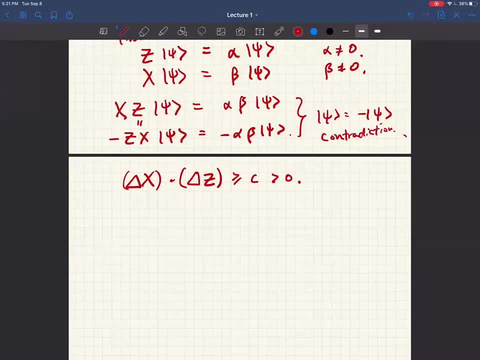 Heisenberg, uncertainty principle, thank you. so or you know the, rather the quantitative, quantitative, but that is conceptually. you know good, and but again, you know this: you can derive this from the fact that the Z X is equal to minus X Z, which comes from the same fact. cool, cool, cool. so this is Heisenberg. 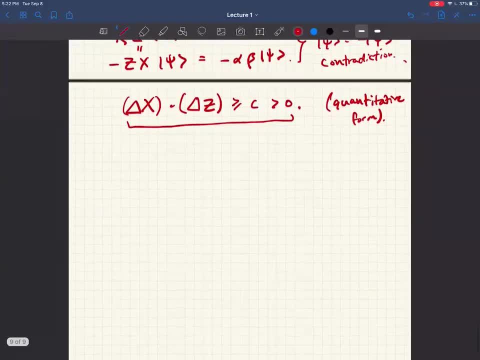 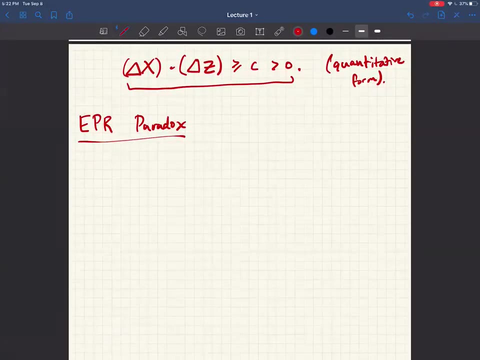 uncertainty. so this: now we can talk about the EPR paradox, another paradox I mentioned at the beginning of lecture. so what's the paradox? you know, Einstein and his friends were thinking about quantum mechanics and we thought about this particular state called the. well, today we called the EPR state. they didn't call it that. it's a. 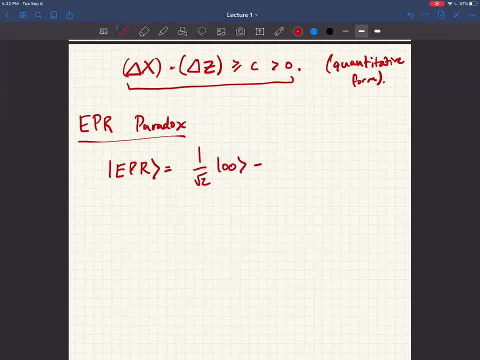 two qubit state and so it's going to be the equal superposition between 0, 0 and 1: 1. so it's, you know, graphically it's two particles, they're maximally entangled to the galactic and they imagine taking the you know two particles in this EPR. 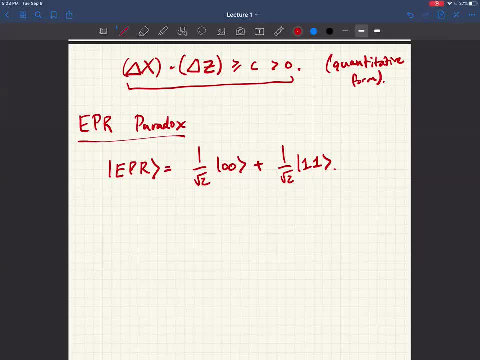 state and separating it by vast distances. you just move, you know, put one at one end of the galaxy and the other at the opposite end, right? so we have two particles here. their, their shared state is this EPR state, and they started just thinking about: well, what are different things you could do to it? well, you can. 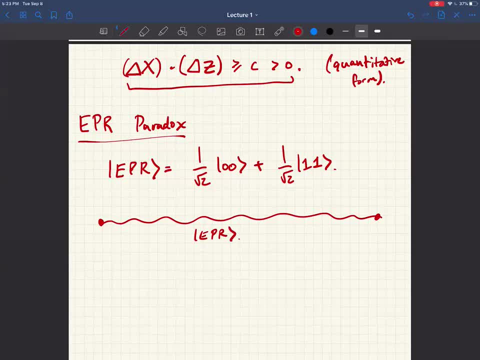 measure the, the two particles, and that's where we clearly 형овор 설치 the two particles. and there is a part where the stars stay at logarithm levels, only Kirkと the two particles. And so let's imagine that what you can only do, 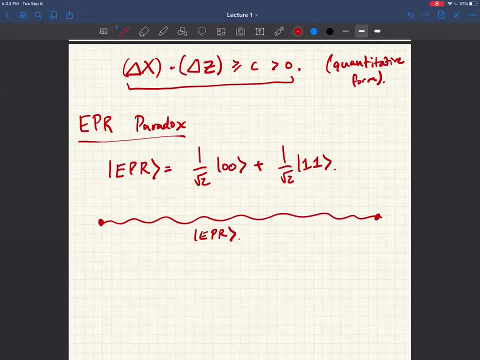 are local measurements. So one person has one particle and the other person has the other particle And we'll call one person Alice and the other person Bob. So let's think about different things they could do. Let's say they both decided to measure their particle. 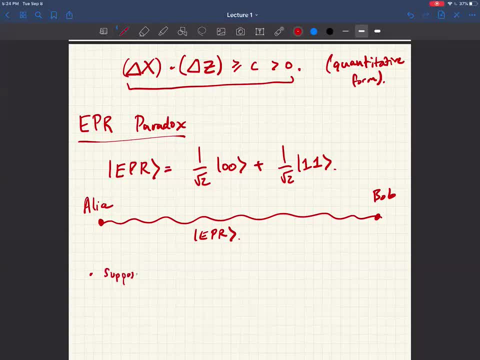 in the standard basis And this was a greater machine could measure Z observables. So they both measured the Z-observables And they both measured the Z-observables. Okay, so let's do the same thing: we measure the Z-observable as well. 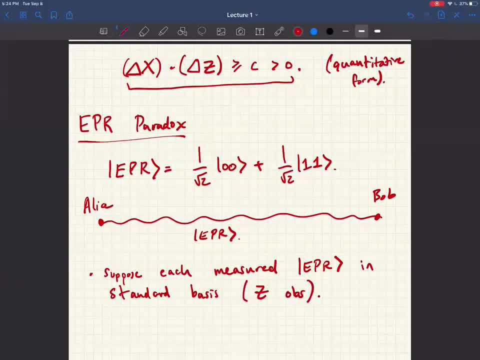 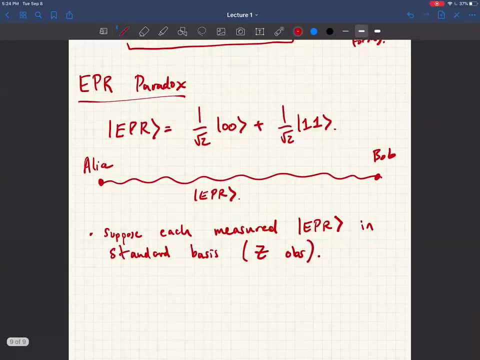 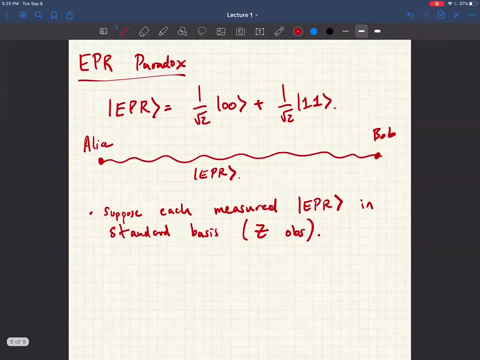 Okay, or in other words, they both measured the Z-observables. Okay, so what are the outcomes? What happens? So if Alice forget Bob? for now, if Alice decides to measure her qubit, the left half of the EPR pair, then what are theyou know she gets zero or one right. With what probabilities? 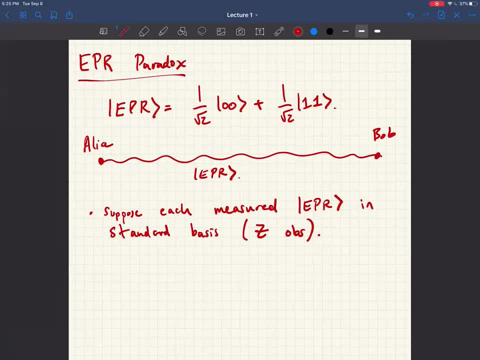 One half, One half Exactly. So Alice is going to see a uniformly random bit. What about Bob Forget whatever Alice didn't get? Or those are the same actually? Yeah, Exactly, Alice and Bob don't get the same thing, right, Alice and Bob don't get the same thing. Alice and Bob. 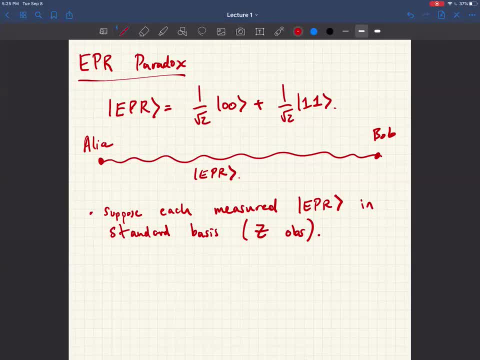 they measure the standard basis, they both get the same exact bit, with probability 1.5.. Because the state will collapse in either 0, 0 or 1, 1.. Okay, so you know, this EPR pair allows them to, you know, get totally synchronized coin flips. 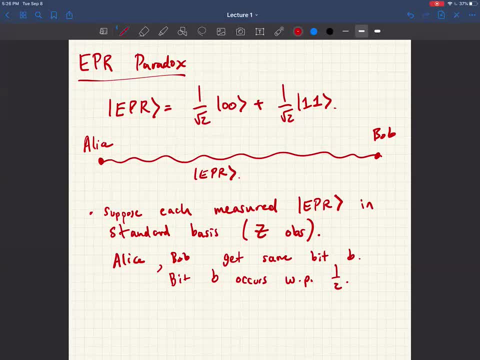 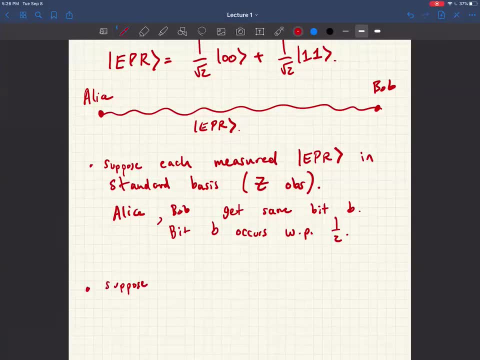 And the coin flips are unbiased. Okay, pretty easy. But suppose each you know, they decided, hey, let's not measure the standard basis, Let's measure it in the X basis, Right? So when you measure the X basis, you get one of two outcomes: either the plus state or the minus state. 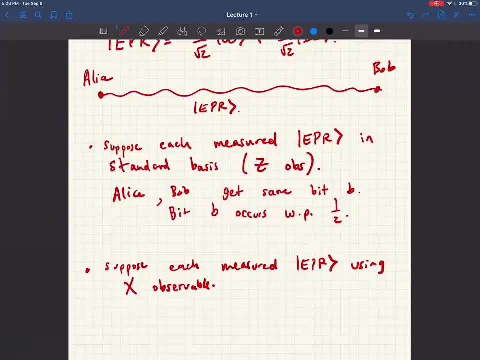 And What will the outcomes be? All right, Yeah, let's start again with Alice. So she's going to see this. you know plus and minus with what probabilities? Okay, Is it the plus one with a state with probability one? 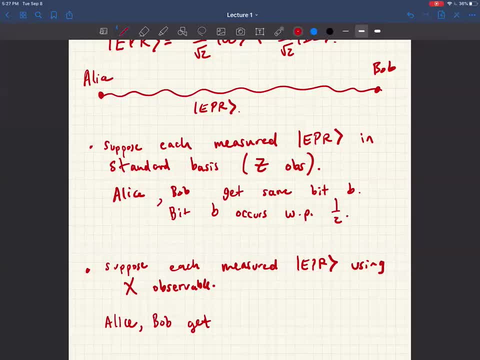 The plus you mean the plus state, right, Yeah, the plus state. sorry, It won't be with probability one, It'll be some other probability. Let's just try to balance, Okay, Well, maybe let's let's go through the calculation together, because I think actually this will be instructed. 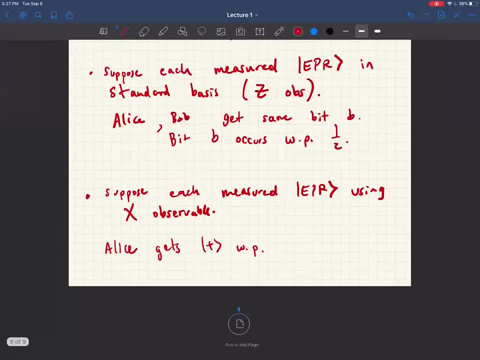 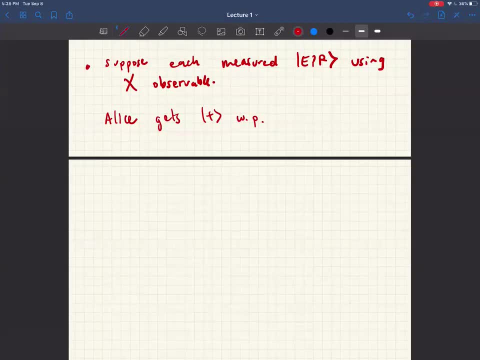 So let me, so you know how. how do we evaluate what the probability of getting a plus state? So we want to know what is the probability that when Alice measures she gets the plus state. Well, we can mechanically calculate. 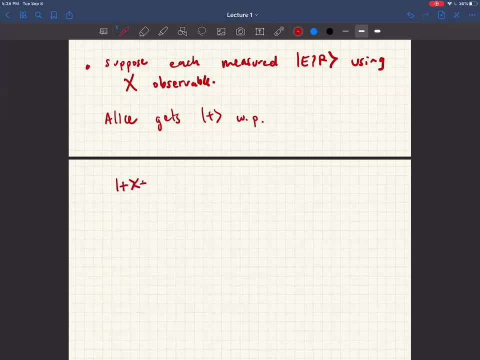 So we want to apply the projection onto the plus state. So this is the projection right And this tensor identity means that Bob isn't measuring anything yet. So this is a projection and we want to apply it to the EPR state, And then we want to take the norm squared. 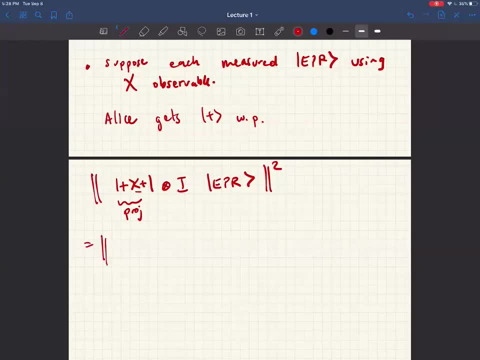 So this is the probability. Well, we can write expand this out, Right, So we get a one over root two, Zero zero, plus one over two, one one, Okay, And we can factor out this: one over root two. 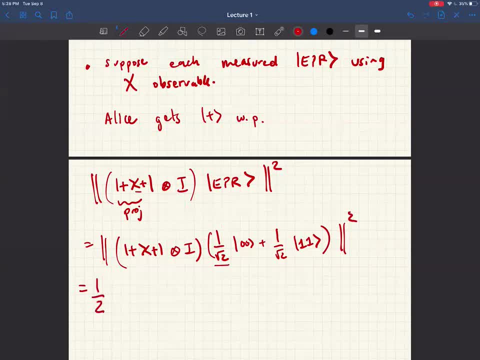 It's going to get square. So this pulls out a one half in front Right And We're going to move this projector. I mean it. it acts only on Alice's qubit right, So this projector is only going to act. 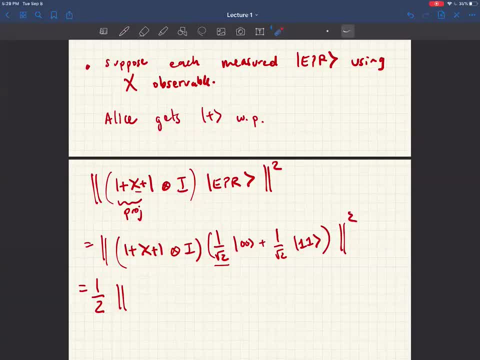 Right. So this projector is only going to act on Alice's qubit Right, Right. So this projector is only going to act on Alice's qubit Right, Right on those qubits. So what does that mean? We're going to do the plus. 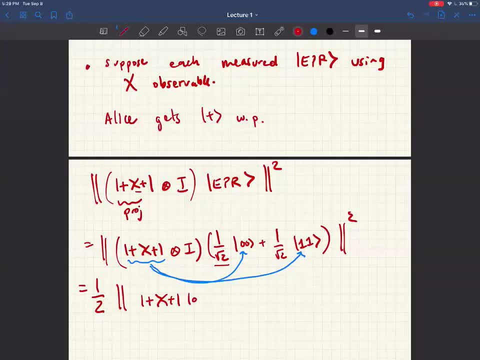 state. This is a projector applied to the first zero tensor Bob's state, which is zero plus. you know- and I'm just sort of writing this on in like a very pedantic way, but hopefully this will be helpful and this is going to be the. 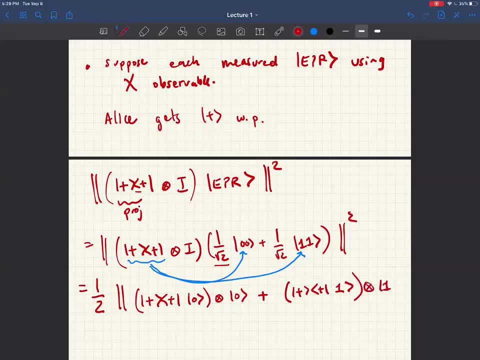 projector applied to Alice's qubit one, with Bob's qubit being one right. Well, this here is a number, because it's, you know, the. it's the inner product between two vectors. What is the overlap between? what is the inner product between the plus state and the zero state? 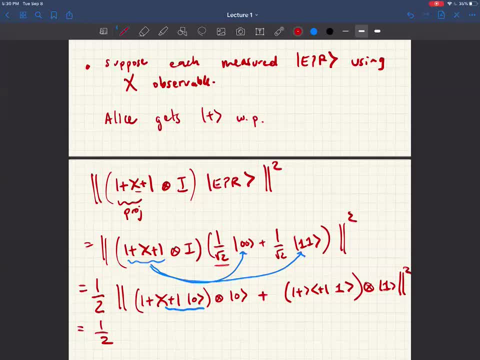 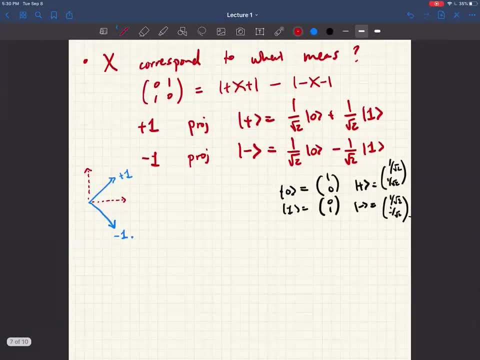 One over square root of two. right, You can see that from. well, you know wherever we wrote the the plus state. Yeah, so the the plus state, the contribution of the zero, is going to be one over square root of two, so we just plug that in. 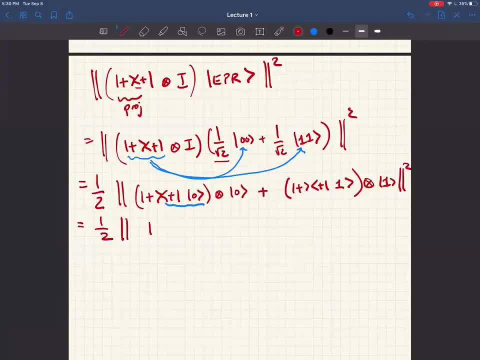 So, uh, you get plus. you get a one over square two. tensor zero plus again. the inner product between plus and one is going to be one over square root two as well. tensor one, right, But you can factor out this: one over square root two, we got. 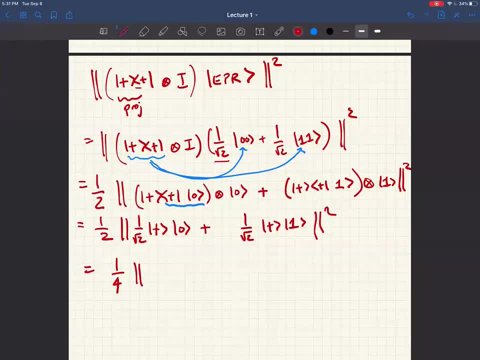 a one fourth. right, Actually, you know I don't want to do that. let's see, let's see here. Ah, or actually, you know, let's try this out, we'll do one over one. I kinda want to do one over one. 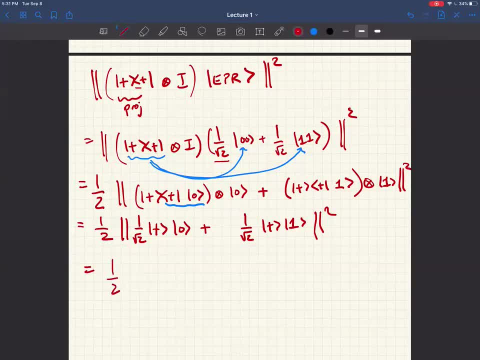 that. Let's keep it this way. It's 1 half. This is going to be plus tensor: 1 over square root, 0 plus 1 over square root, 1 squared. But just notice that this is nothing but another copy of the plus. 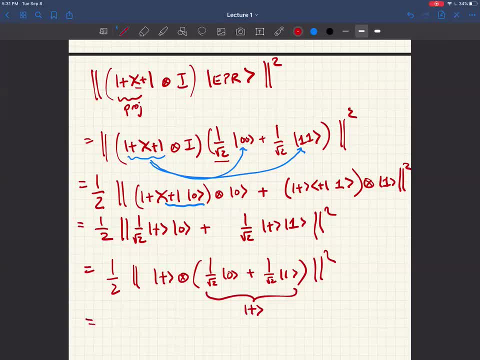 state right And plus tensor plus. this is a unit vector. The norm of this is 1.. So we're just going to get 1 half. So again, what we've just calculated is that Alice will get the plus state with. 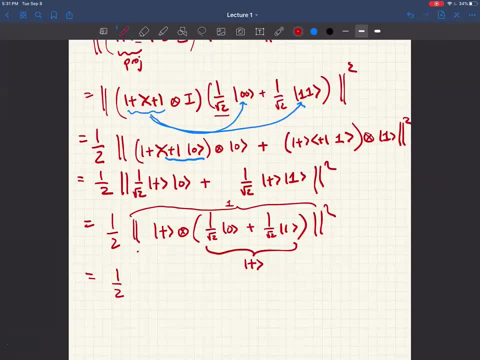 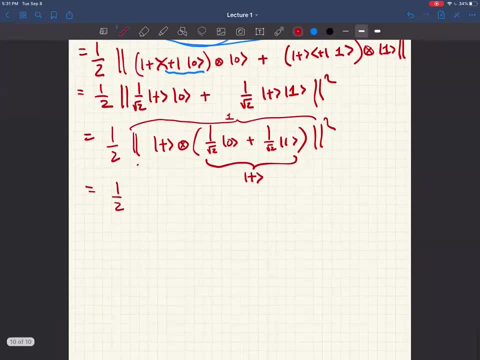 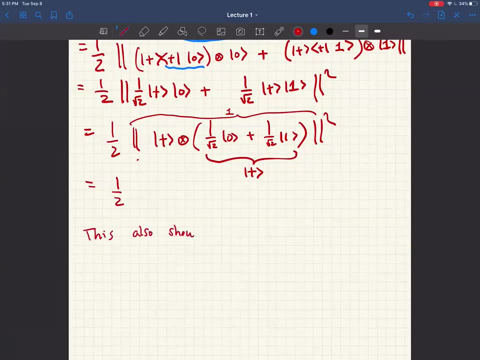 probability 1 half. And already in this calculation we've seen when this happens, what happens to Bob's side, like what happens to Bob's qubit. What is his state? now, Good, The plus state, right. You see here that you know when Alice does a measurement and she 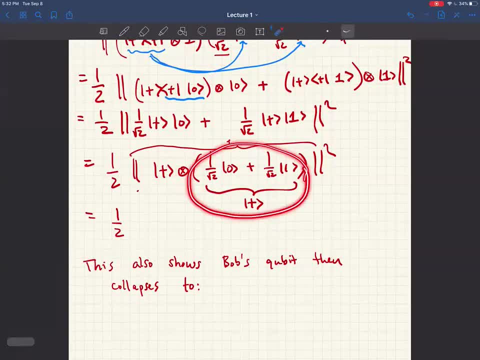 obtains a plus outcome, then this is what Bob's state turns into. It also turns into the plus state. So when Alice does a measurement and she obtains a plus outcome, then this is what Bob's state turns into. It also turns into the plus state. So when Bob simultaneously measures his 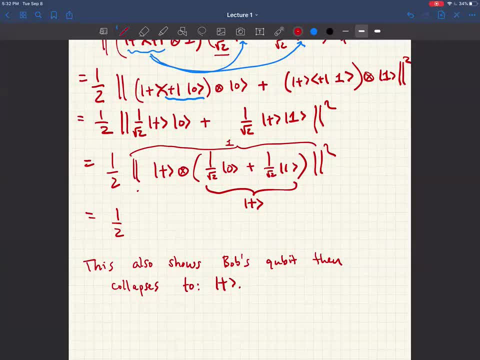 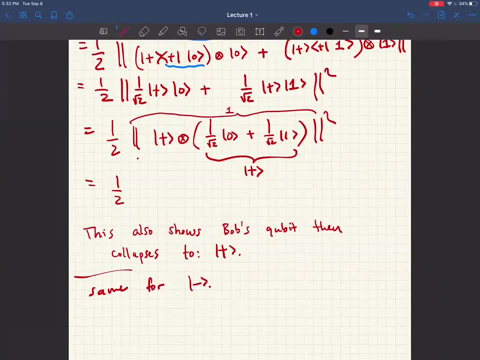 qubit in the plus minus basis, he's always going to get plus. Okay, So they both get Alice and Bob get plus plus with probability 1 half, minus, minus with probability 1, half right. So that's kind of funny. Even when they change their bases, as long as they use the same basis on both sides. 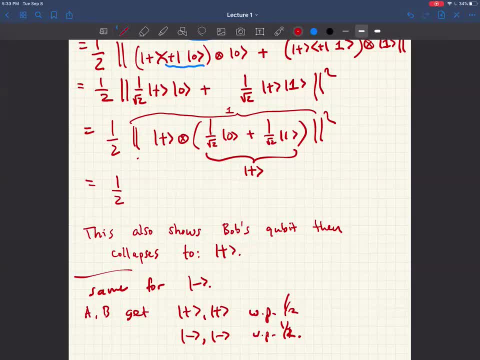 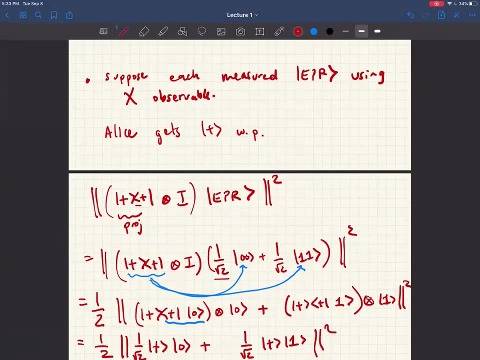 this EPR pair is always going to have them have matching answers. Why did you use the plus states when calculating the projection rather than minus? Well, because I wanted to know you know what's the probability that she gets the plus state. So that means I have to take the calculate. 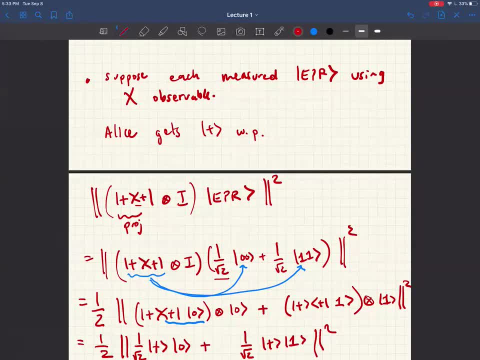 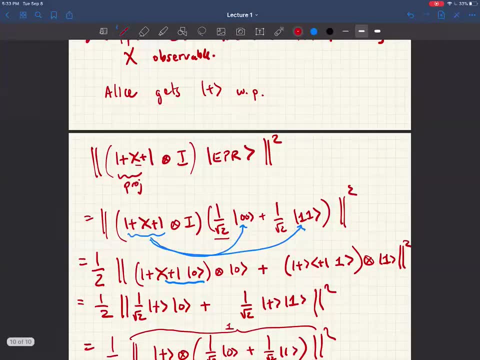 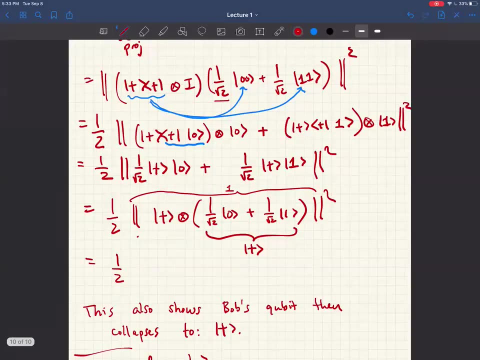 the projection onto the plus state. Does that make sense? Yeah, exactly. You just do the exact same calculation, but you replace with all minuses And you'll see that Bob's state will also collapse into a minus state. And and where did that minus come from? Well, it came from this term. You have a minus 1, right. 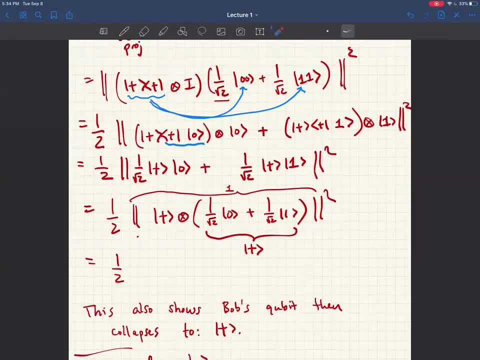 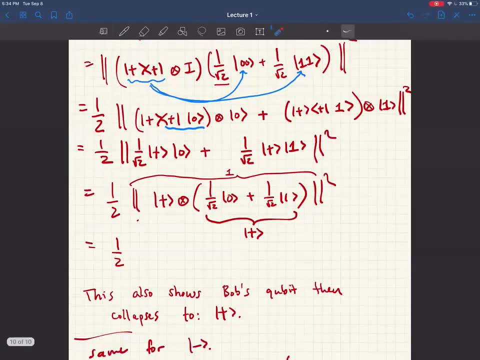 Okay, between the minus state and the one state is going to be minus one over square root two, So so that that's why it all works out Alrighty. Uh, okay, So hopefully that that makes sense. Um. 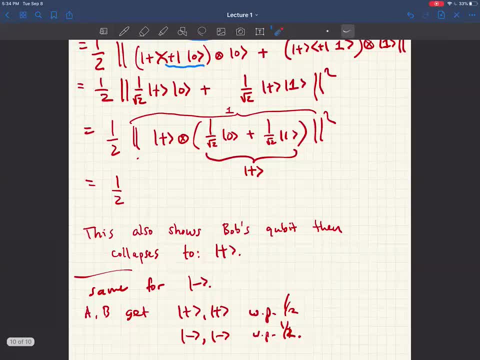 where were we going with this Good So? so we've considered these two scenarios. Measuring in the standard basis: they get matching answers. Measuring in the x basis: they they also get matching answers, and Einstein, Podolsky and Rosen thought this was really strange. 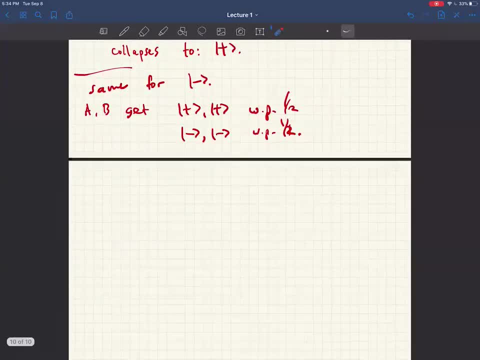 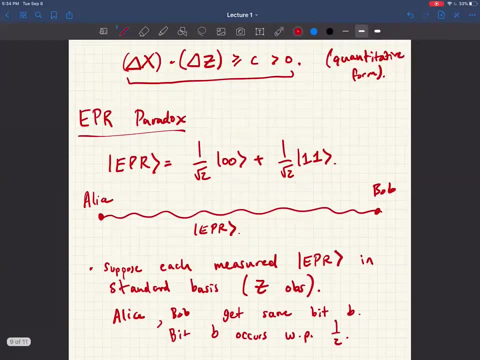 Something was really fishy with this. Why is did they think it was fishy? Well, you remember that Alice and Bob, you know they're on opposite sides of the galaxy, right? Um, and you know from Alice's point of view, you know. so let's say that she decides to, um, uh, flip a coin to decide. 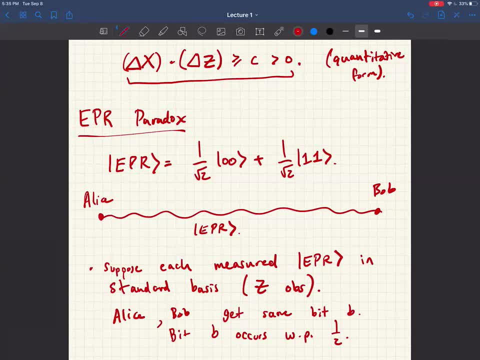 whether she wants to measure in the standard basis or in the X basis, right? So Bob has no idea which basis she's going to measure it? right? Because Bob's just way too far away. She flips a coin and she measures, but what does she know? She knows that no matter what basis she measured in. 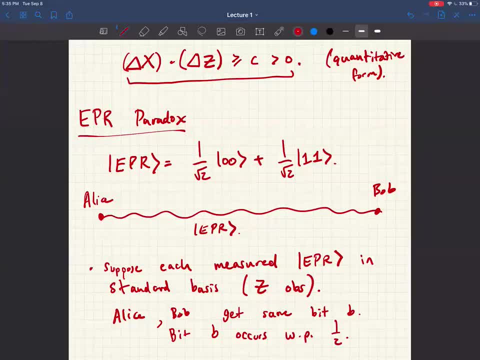 if Bob happened to be lucky and measured in that same exact basis, he would always get the same exact outcome, right? But that's kind of weird because it was sort of say that you know this particle on Bob's side. it couldn't have known what basis Alice chose, So this particle that 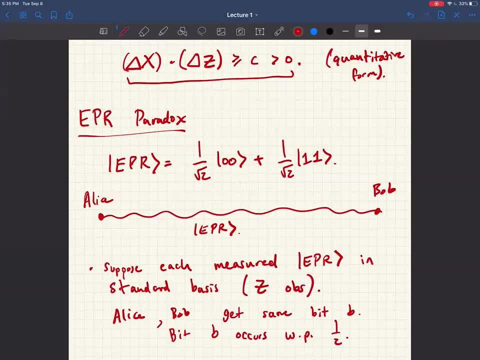 Bob's qubit must have known ahead of time. Okay, sorry, let me back up. So when Alice measures her particle in the standard basis, and let's say she gets a zero right, Then she knows Bob's qubit also. 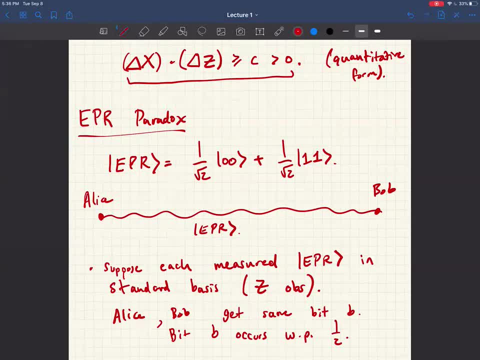 has to measure zero. So from Alice's point of view, this tells her that Bob's qubit maybe really wasn't the zero state the whole time. right, We just didn't know it like it's just due to our own ignorance or whatever, but really after the fact we learned that it was in the zero. 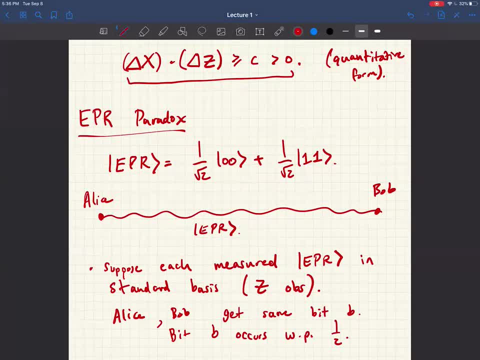 state okay. But if Alice, on the other hand, decided to measure in the- sorry, that's a short ingress cat- If Alice decides to measure in the x basis, then you know, let's say she gets the minus outcome, then she knows in her head that Bob's state must have also. 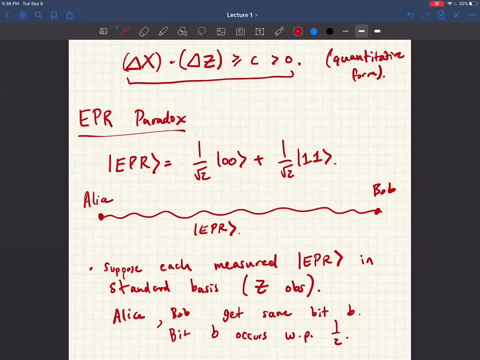 been in the minus outcome. So you know, putting all of this together, like Alice, would reasonably conclude that Bob's state was both determined as the zero state and the minus state at the same time. We know from Heisenberg's uncertainty principle that this is not allowed, Like Bob's qubit cannot. 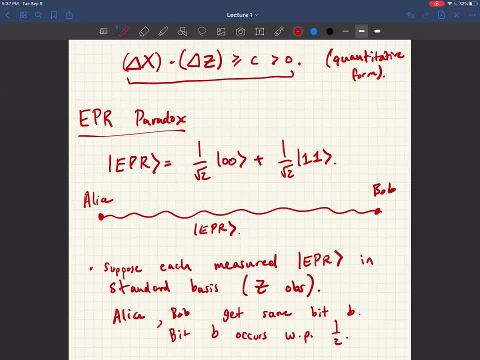 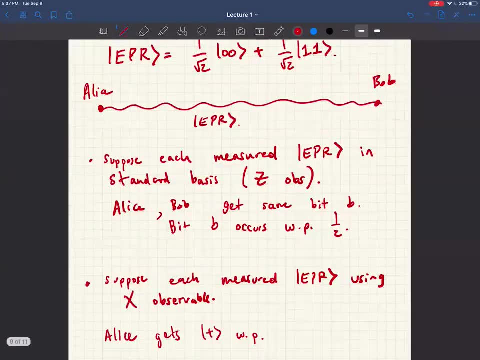 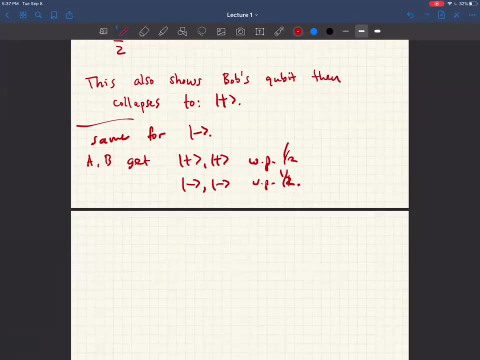 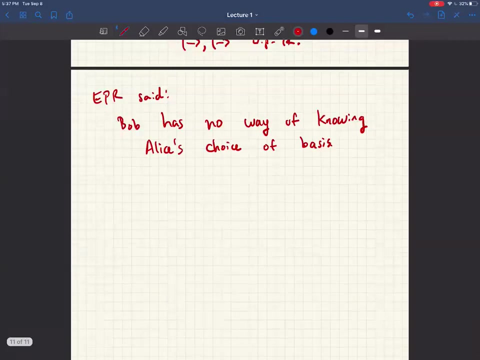 be determined in these two bases simultaneously? Does the reasoning make sense here? So let me just kind of sketch that down. EPR said that there's a negative gradient in diversity and so on. right, So like the candidate elements were called differently, So are you know. do have fewer Papa. 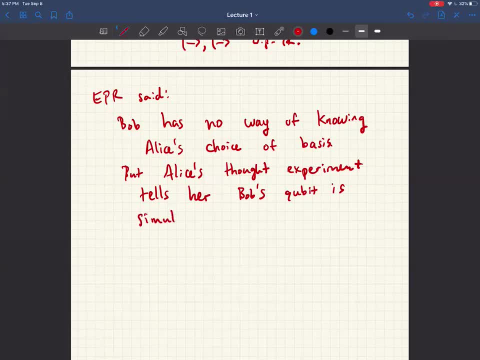 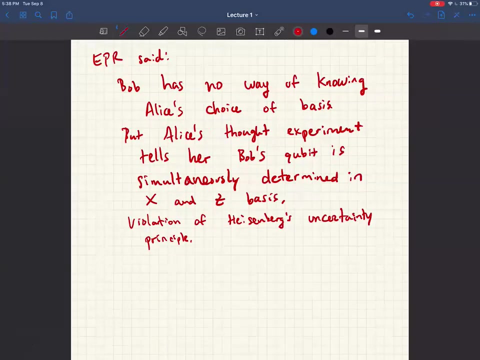 veterans. Yeah, Thank you. So, fundamentally, what you're saying is that being a subsystem of a two-particle system is distinct from being a one-particle system, because the Heisenberg's uncertainty principle doesn't apply in the same way to the one particle that Bob has here. 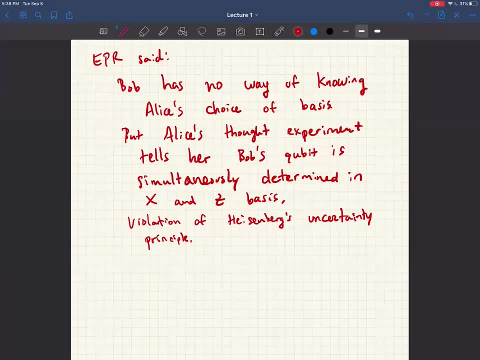 Well, This is sort of what they were confused about. They were trying to figure out exactly this. Like they know, for the one-particle system, Heisenberg's principle is definitely true. I mean, we just saw proof of it. 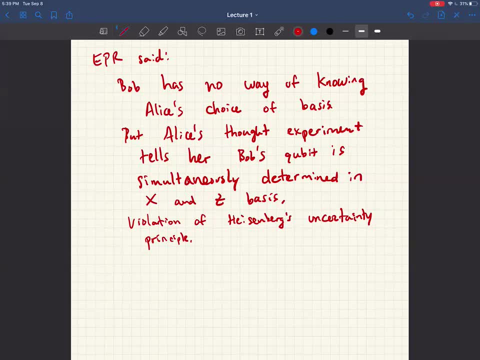 But you know they're trying to reconcile it with this same calculation that we did. And let me make it clear: like you know, oftentimes people say that Einstein didn't understand quantum mechanics or, you know, he didn't believe in it. 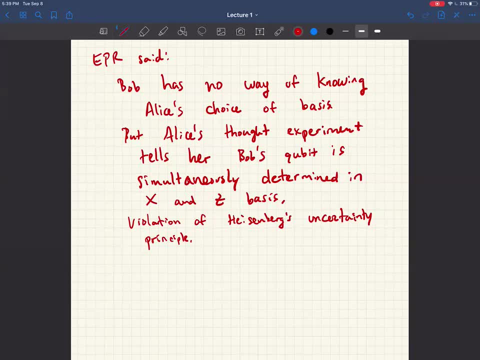 I mean he understood it extremely well. I mean, in fact, like he discovered a lot of the principles of quantum mechanics And he, you know, he trusts that the calculations are correct. But what is bothering him is the basically like the interpretation of what's going on. 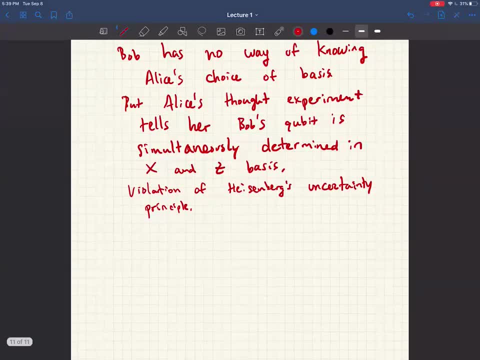 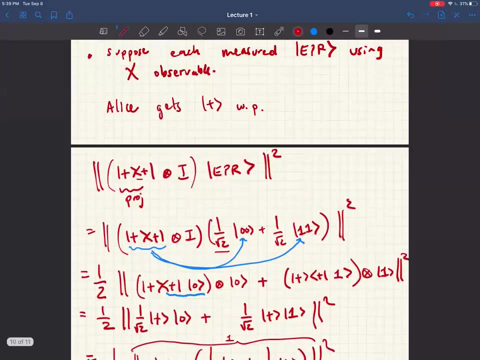 Right And basically what they had in mind, and they had an implicit assumption, which is that each of these particles have, like, a defined state, Like you know, Like basically you know, EPR is assuming that, because Bob is so far away, you know. 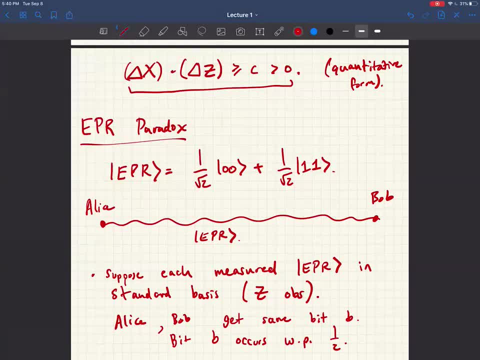 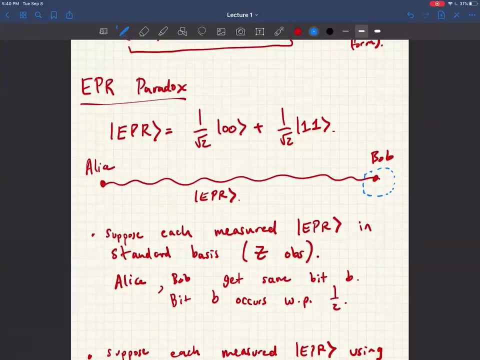 that you know this piece of space and time around Bob's particle is, you know, should in some sense have all information that you need to predict the outcome of Bob's measurements. Right, And Alice's reasoning is: well, If I did measurement A versus measurement Z versus measurement X, I would have gleaned: 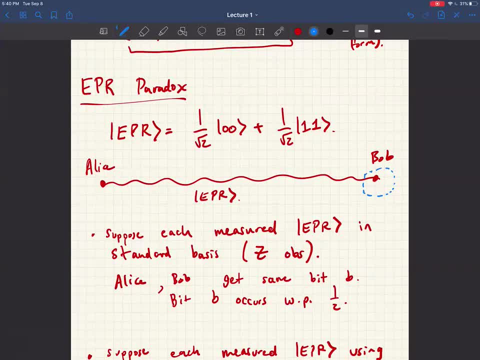 some knowledge about what Bob's bubble. would you know what information Bob's bubble has? And that shouldn't affect anything in his bubble because he's just so far away, Right, So this bubble must have contained information about the Z and X outcomes. 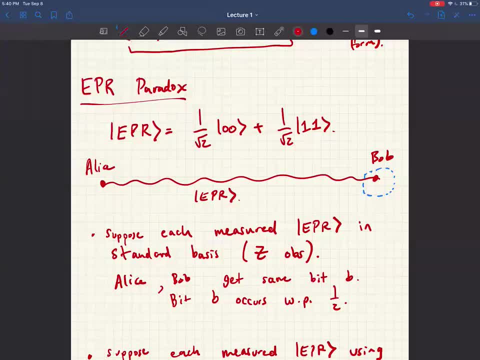 Right. So it must have had some You know little Like somewhere in, like the fabric of nature or something. there must have been like a little indicator that said, if I measured in the Z basis, what would have happened? 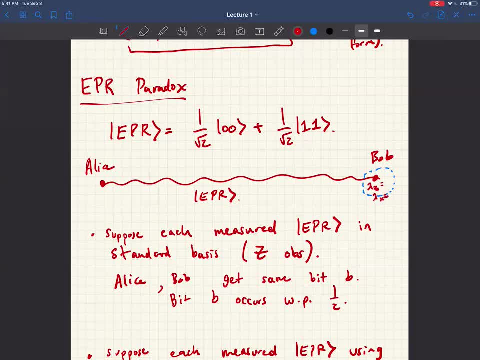 And if I measured in the X basis, what would have happened? Right, And you know, Alice's thought experiment is telling you that. you know, however I measure it, it's going to pin down what you know what's going to happen. 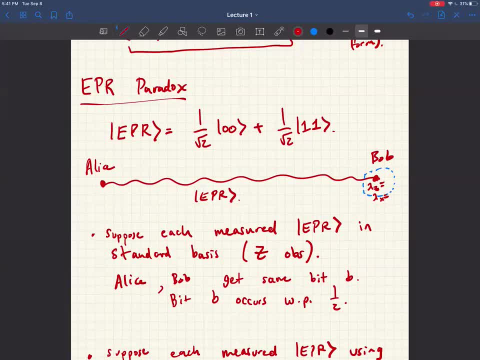 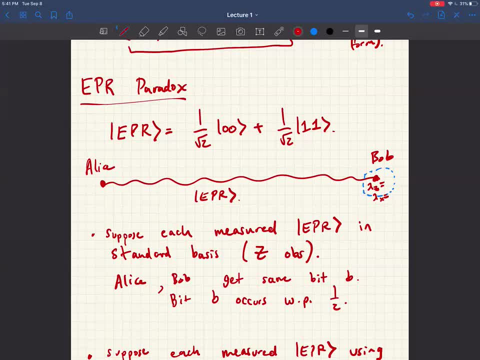 Okay. So Gary has a question. I don't understand how this violates Heisenberg uncertainty. If she hasn't made a measurement yet, then Bob's qubit hasn't been determined in any basis. So this is the thing that EPR didn't understand. 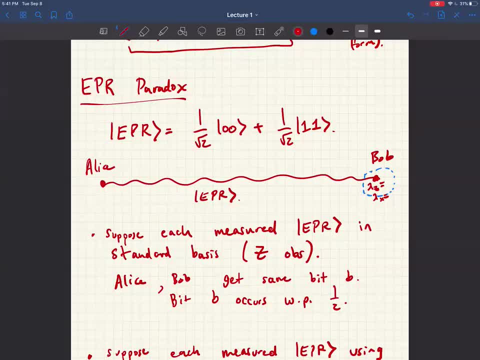 So, you know, they're thinking of like what's really going on behind the scenes, like what is mother nature doing, and i think what they intrinsically believed is that, uh, you know, mother nature is sort of like keeping track locally for every particle what measurements on it is supposed to produce. 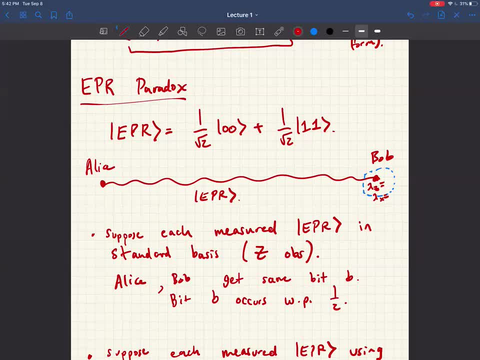 right, um, and you know, if you look at the mathematics of quantum information, you know you're right. like bob's, qubit isn't determined yet. uh, right, if alice hasn't made a measurement. but what einstein, podolsky and rosen are saying is that, well, the the mathematics of quantum. 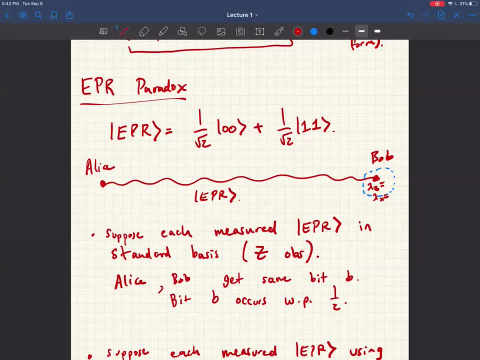 information doesn't say this, but, uh, it should, and so therefore it's incomplete, it's missing this: these extra pieces of information, these lambdas that i've just written that would tell you about it. um so, so this is the the thing that there was like. well, you know, there has to be a 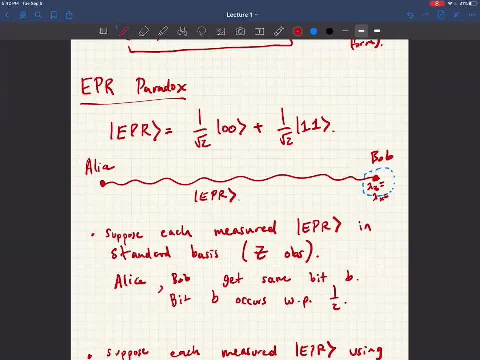 better theory of of nature that, uh, that explains all of this, right, because otherwise it would sort of indicate that somehow, by doing a local action on her part, alice could, you know, instantaneously affect the state of bob's system, and this really bothered. i mean, it doesn't affect it in a way that would allow alice to communicate to bob, but you know. 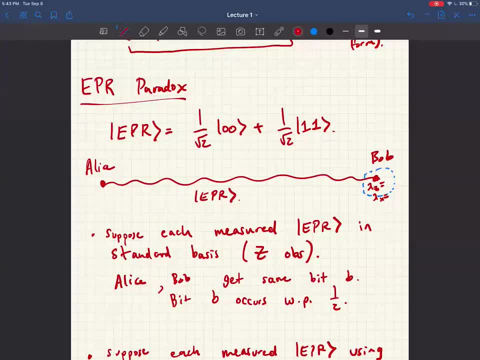 when you look at like what's happening, like you're still collapsing this quantum state in an instantaneous way- at least that's what the mathematics sort of seems to suggest- and and that sort of thing, like really bothered einstein, you know, because you know he created relativity after all. uh, and and so they concluded, all right, there has to be a. 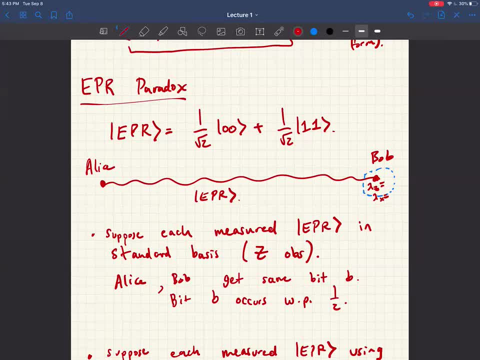 replacement theory for quantum mechanics that gets, you know, removes this instantaneous long range collapsing of states. um okay, xin chang is asking: sorry, what is zero, zero and one, one mean exactly. so those are, uh, uh, this, so this is a superposition of two classical states. you know, the two particles being in the state zero, zero or the state one one. 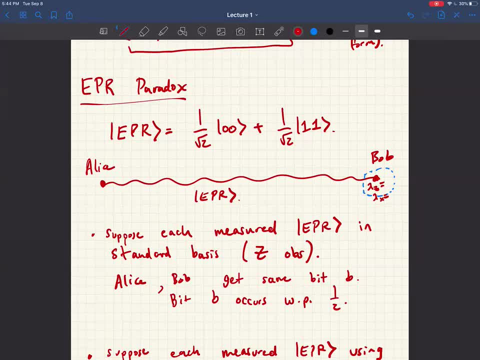 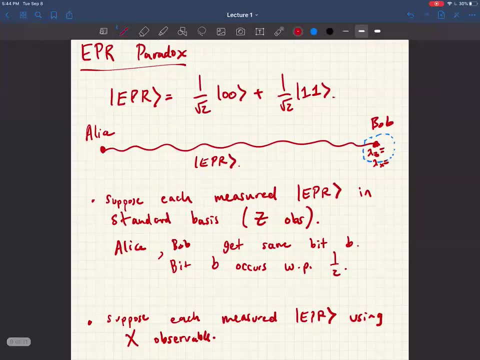 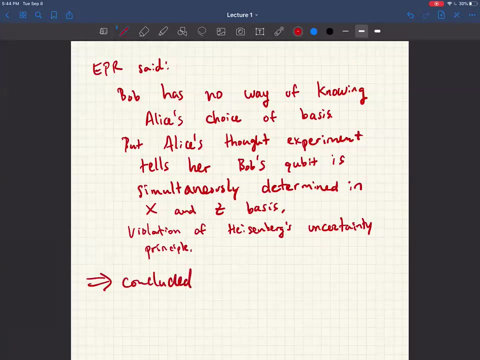 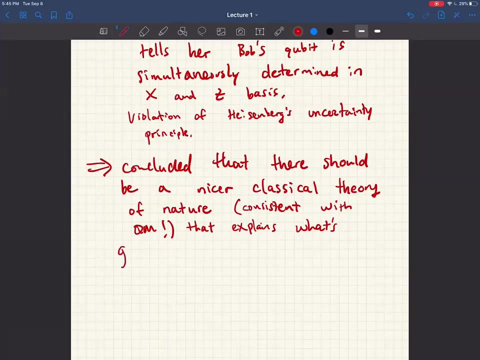 right. so like, for example, you know, like we saw earlier, if they both measured in the standard basis, they would both get zero, uh separately, and or one separately, okay, okay, uh. any other questions about the epr paradox? you, okay, okay, okay, okay, so you. So that was their hope. they wanted a nicer classical theory. you know some theory that? 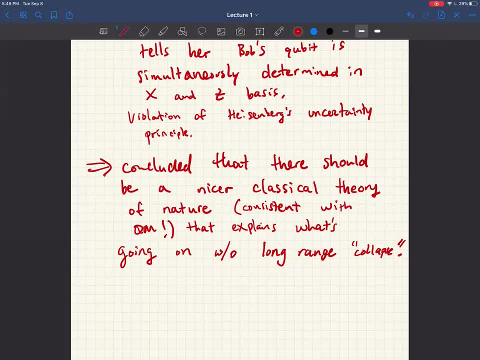 you know nice and classical makes more sense that that's consistent with the quantum theory. So before I think, you mentioned that when the plus axon zero, zero and x on one or two, So the plus doesn't it acts on the first. you know 00 refers to two particles, right, the 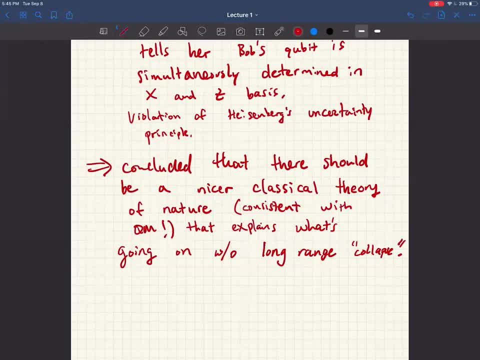 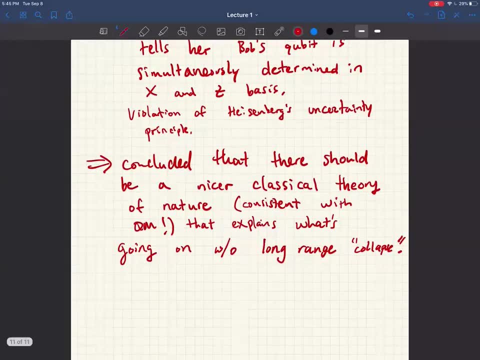 state of two particles and the plus projection is is just something that Alice is doing, So it just acts on the left hand zero or the left hand one right. so You know when I say 00 that that just you know that's talking about two particles. 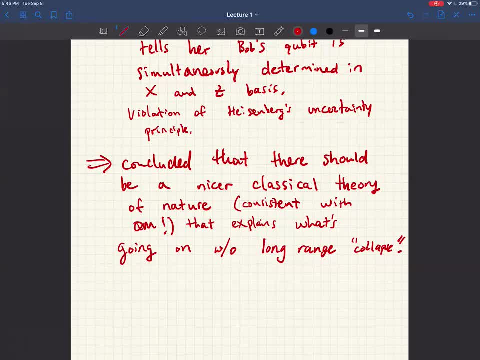 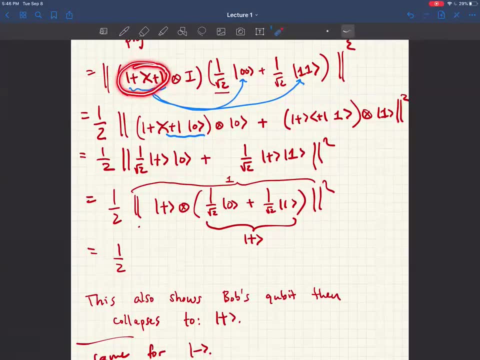 the left one and the right one And The. What I'm saying is that this projector, this, this is a two by two matrix. right, when considered by itself, It acts on just the first half of this 00 cat. Okay, I think we're close to. 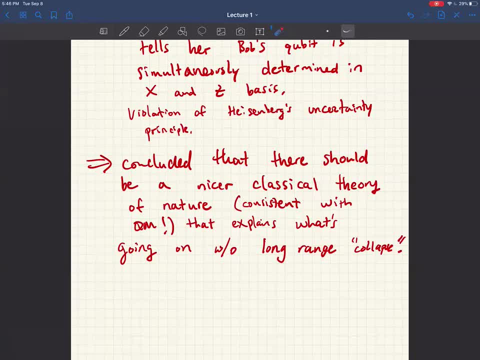 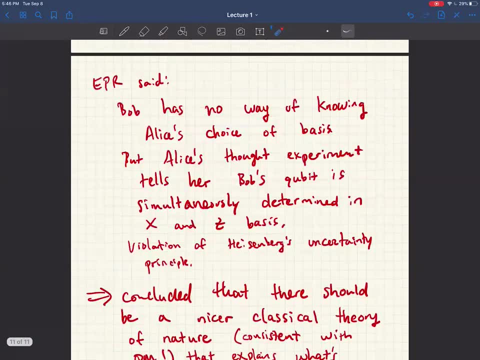 When would act on the second half? it wouldn't act on the second half of the. so Bob's. you know, when Bob applies a his measurement, then that's when it would act on the second half. So So, for example, Bob's Projection measurement. 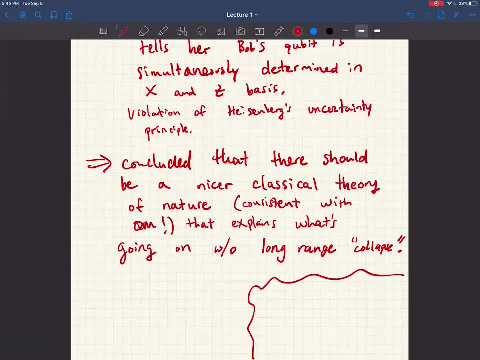 Well, let me draw an aside like, let's say, you know we reverse the order of things. We said that Bob measured first, then his projector would be, Would be this plus plus tensor identity, like this identity means Alice isn't measuring. 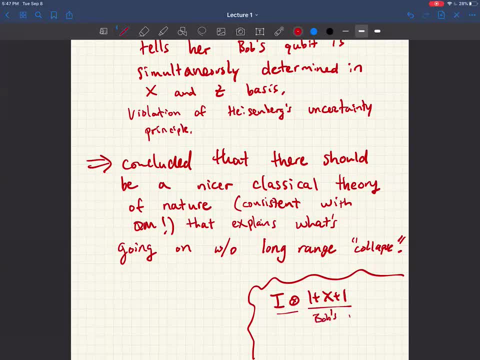 yet- And this is Bob's projector, Okay, Let's see. So, while lead is asking: is accepted resolution to the paradox that one has to abandon the principle of locality? See what's the what's a good way to answer this. 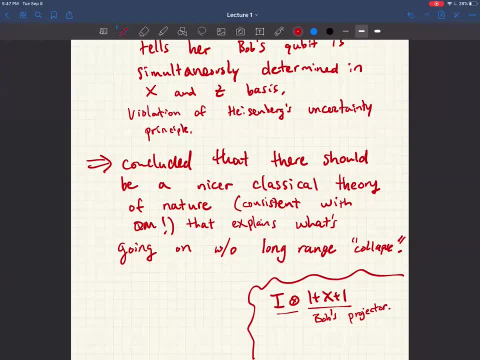 Yes and no. So So I think it gets confusing here because These terms Okay, So one answer is yes. It's saying that fundamentally like the only way to describe Yes, The only way to describe, mathematically describe- what's going on in a satisfactory way is 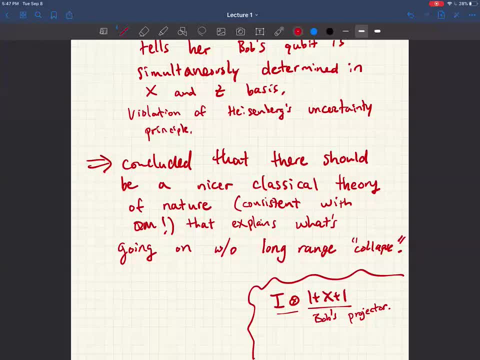 to say that Underneath it all, there's some non local behavior going on. like I do something in this part of the galaxy, It somehow changes the state at you know somewhere else in the universe. You know that sounds really freaky, but it's not in a way that allows you to instantaneously. 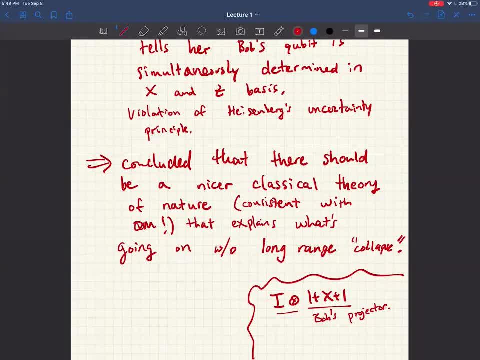 communicate With someone at the other side. So it's so in a sense. it's like All the predictions that you would make In your local part of the universe Is local, like you can explain everything just by saying you know the laws of nature act. 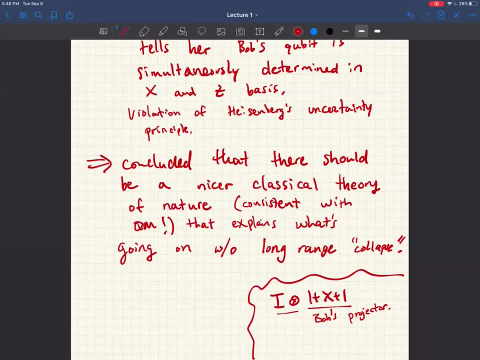 locally. It's just that when you combine the measurement results from one part of the galaxy with you know the measurement results with some other part of the galaxy and bring them together and you look at, you say wait a minute, There's some weird correlations between them. 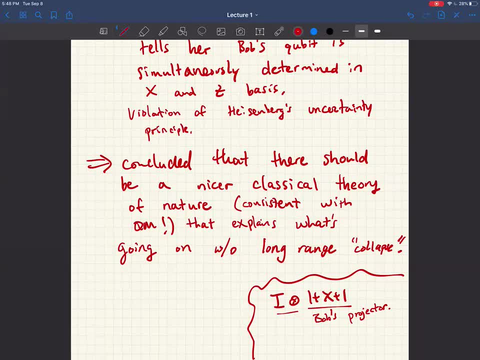 And it These correlations. These correlations are what are called non local. Okay, But before you brought them, these measurement results together, you wouldn't have known that there was any non locality going on. Okay, so maybe a vague answer, but maybe. 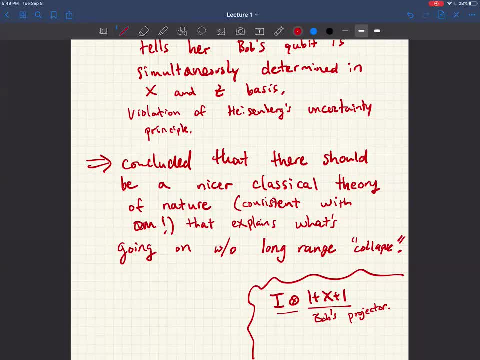 You got something out of it, Okay. Shen Yang is asking: what if EPR doesn't exist in nature for Alice and Bob? You mean the EPR states Yes. I'm saying that if it only happens, if they are local to each other, then it's not a paradox. 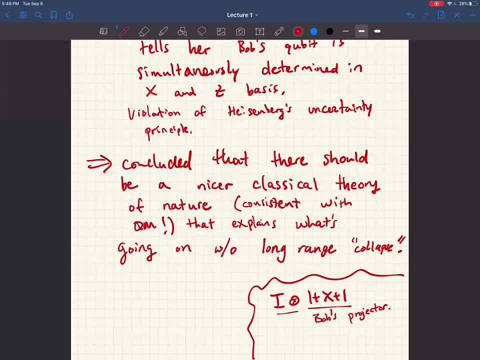 Oh, good question. You're sort of saying like: oh, maybe for some reason it's not possible for Alice and Bob to be on opposite sides of the galaxy and share this specific state? Right, Yeah, You know that is possible, but that was kind of as far as we can tell. That's, I mean. the only way that would be true is if you know the laws of nature change when you move to a different part of the Galaxy. but assuming that you know the laws of physics are the same everywhere, then you know. people have been able to prepare these EPR states and distribute them over thousands. 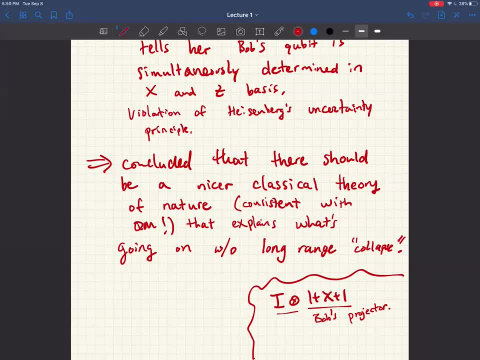 of kilometers, Or maybe hundreds, but anyways, pretty far, And there's no reason to expect that you couldn't. just you know if you're careful enough to continue splitting them up further and further apart. Okay, Okay, So you know I have 10 minutes left. you know, maybe I'll try to get started on explanation. 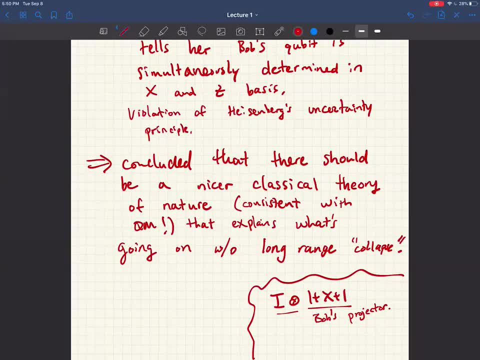 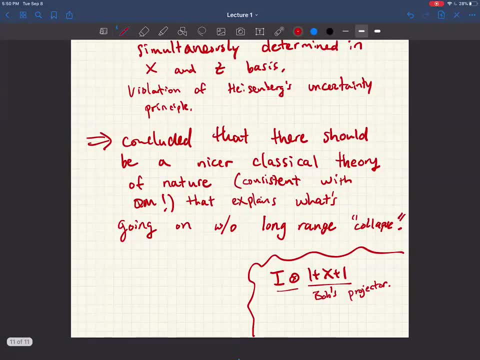 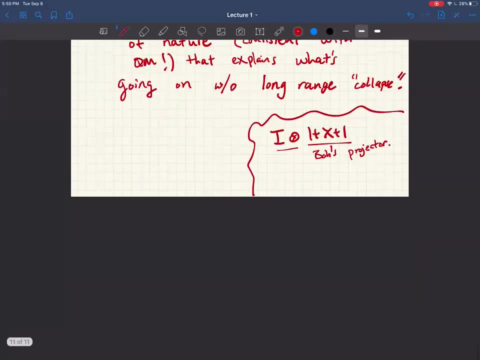 of Bell's theorem, And you know, I'll try to make as much progress on that before the class ends, And then I'm happy to answer questions afterwards. Okie dokie, So that's the EPR paradox. They were very confused. 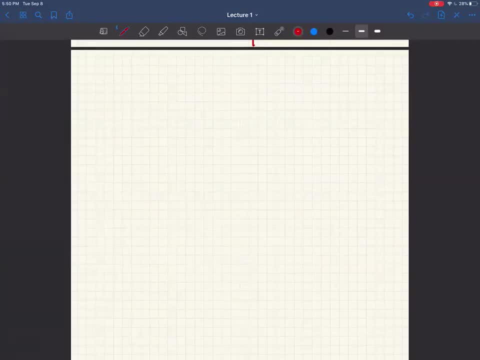 And you know, this caused like all sorts of philosophical debates That just lasted for 30 years until in 1964, John Bell came along and said: basically you know this dream of Einstein, Podolsky and Rosen of coming up with a nice classical. 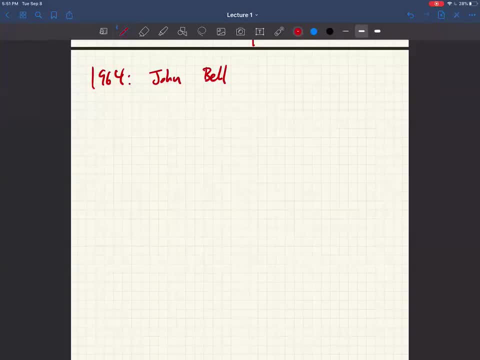 theory that explains all of this. this is not possible. Like I mentioned earlier, Bell's theorem shows that there is no classical theory that respects locality that could explain all of quantum mechanics. Right, No matter how clever you were, you cannot fit a local classical theory around quantum. 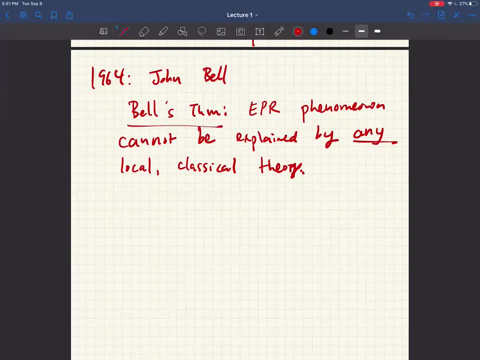 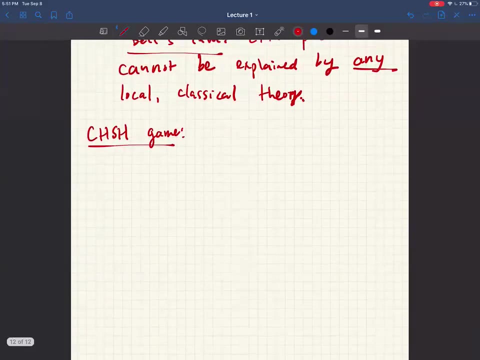 mechanics. So how did he prove this? Well, I'm going to explain it in a modern formulation, in the terms of this thing called the CHSH game. Okay, And this game, I mean, it was discovered after John Bell, and you know the way we explain. 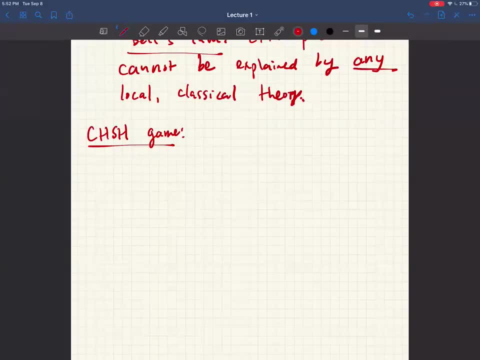 it now. it is sort of like much simpler than it was originally formulated. The way it works is follows: You know You have two favorite people, Alice and Bob, And let's think of them as players in a game, Right? So they're really far away from each other. 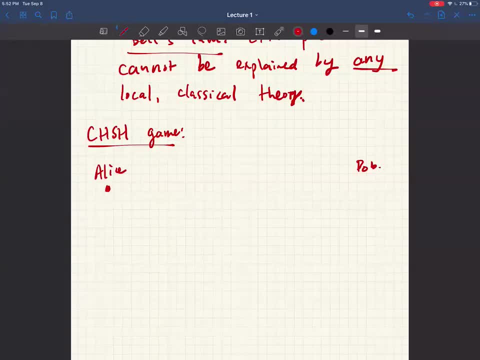 Right And so far that they're not able to send signals, to communicate, But instead they play this game with a referee who's in the middle, And this game is really simple. What the referee does is: the referee is going to first choose. 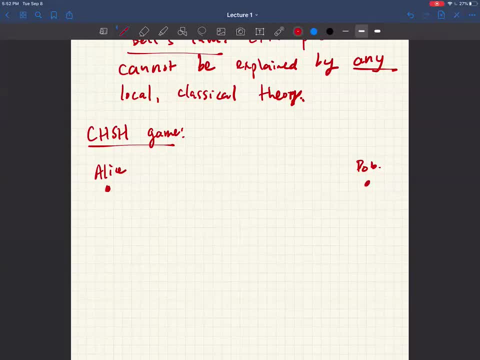 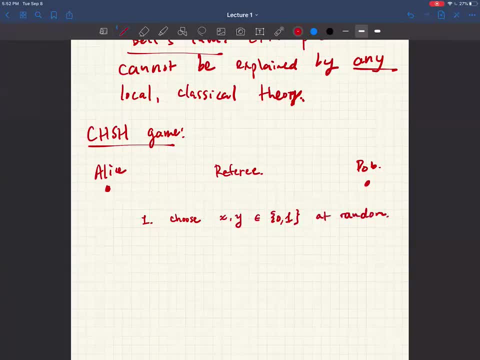 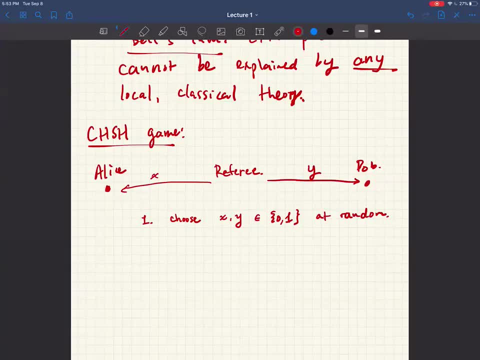 Two, One like, perform some physical process on their end and they obtain an answer. So Alice is going to return an answer instant. you know, at that very moment, some answer called A and Bob is going to return an answer called B. These answers: 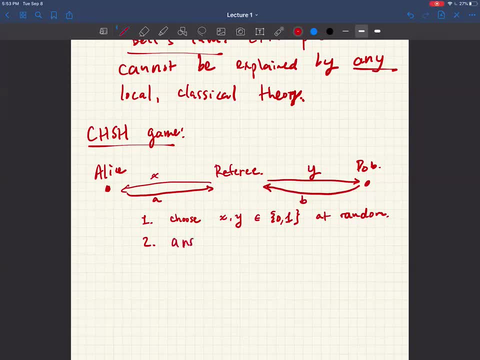 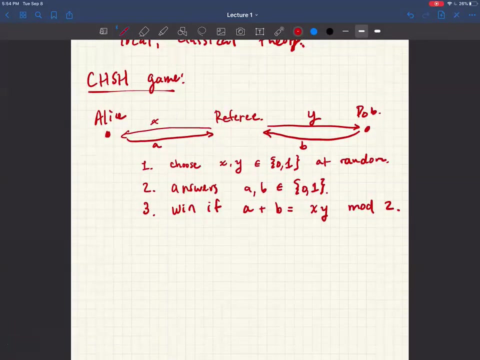 are also bits, Okay, and send it back to the referee. and at that instant the referee is going to decide whether Alice and Bob win the game. And they win the game if A plus B is equal to X times Y mod 2.. That's the game. it's very simple. So it's just one round. Alice has no idea. 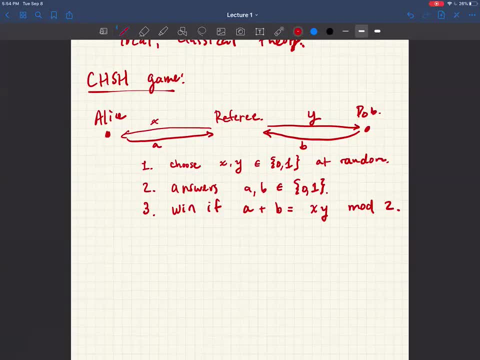 what Bob's question was. Bob has no idea what Alice's question was, but they're still supposed to produce these answers A and B that satisfy this predicate, This condition. Okay, it's kind of a strange game. We can now think: well, how is Alice going to answer the question? and the answer is B, So Alice? 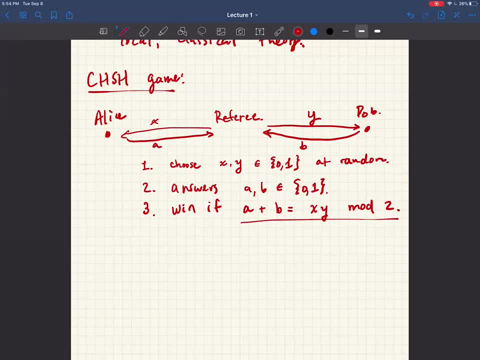 well, can Alice and Bob win right? So, Alice and Bob, they know the rules of the game, They know that this is what they're going to be tested on, So they want to come up with the best possible strategy to win it with the maximum probability. Okay, So what is that maximum probability? 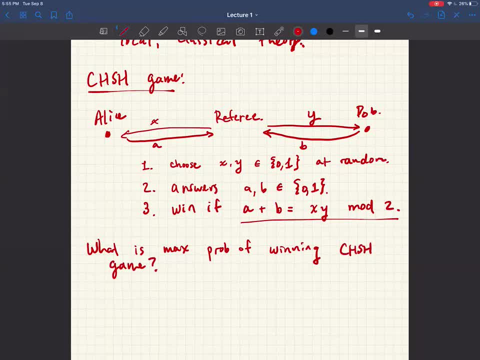 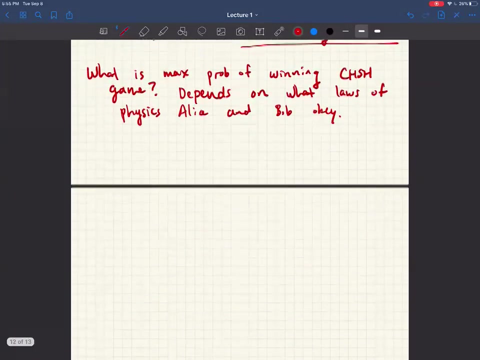 Well, this depends on what Alice and Bob are allowed to do, Like, what laws of physics are they subject to? Okay, So suppose that Alice and Bob are allowed to do this. So Alice and Bob followed a classical theory. Like you know, they followed some theory that 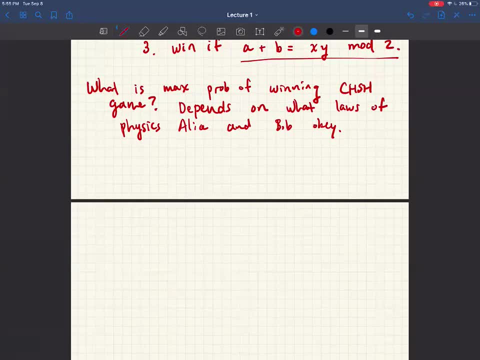 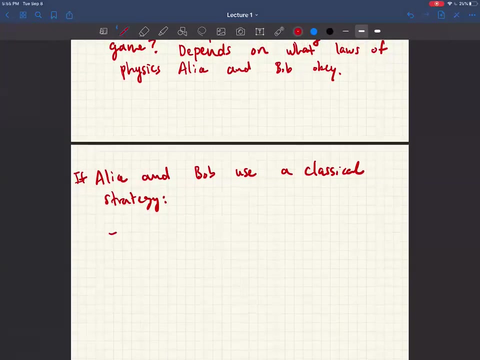 EPR would have liked right. So that means that Alice and Bob use some classical strategy. So if Alice and Bob use a classical strategy, so what's a classical strategy? Well, a simple type of classical strategy is if Alice and Bob are deterministic, meaning that Alice's answer A is some determined function of. 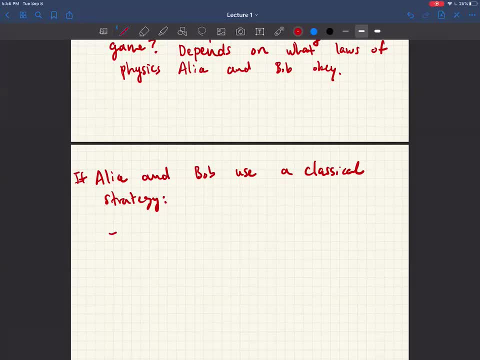 her question. So Alice and Bob are deterministic, meaning that Alice's answer A is some determined function of her question. All right, Meaning that before the game starts, Alice and Bob, they get. you know, they just plan on the best possible functions to respond with. 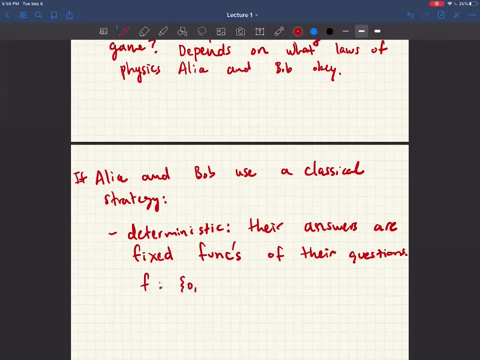 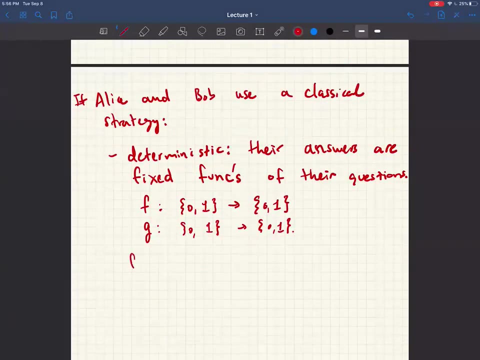 So Alice picks some function f that maps a question to some answer, And Bob has. he also comes up with a function right, And so their answers are just going to be f of x and g of y, So So, 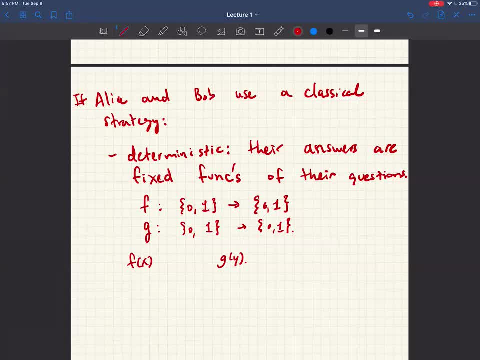 Yeah, you know the, so the you know. let's say they use this kind of strategy. It's certainly classical, right? They don't need to use any quantum physics in order to use a strategy. What is their maximum winning probability? 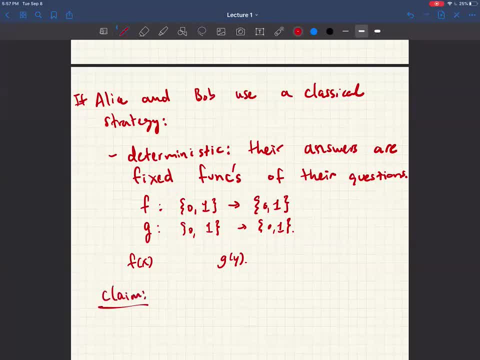 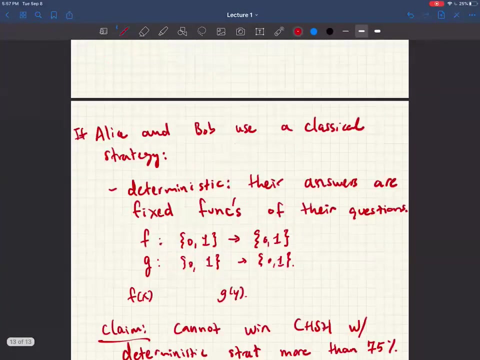 Right, And the claim is that they cannot win the CHSH game with probability greater than three-quarters Right, and when I say three-quarters, I mean over what? you know what probability. Well, the questions x and y were chosen at random. so, over the choice of the questions, 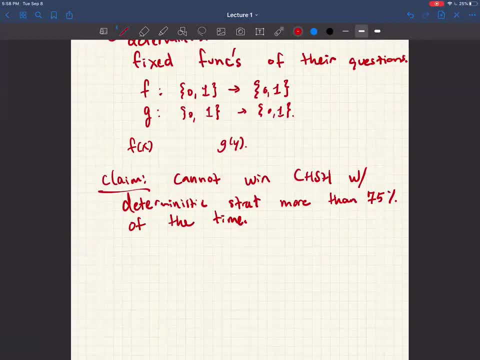 they cannot win more than 75% of the time, right, And there's an easy way to see this. you know, basically, no matter what functions f and g, Alice and Bob decide upon ahead of time, they're always going to output wrong answers, at least. 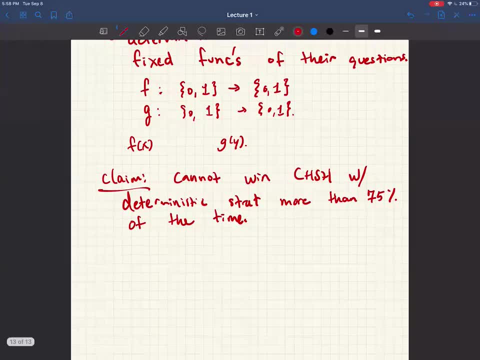 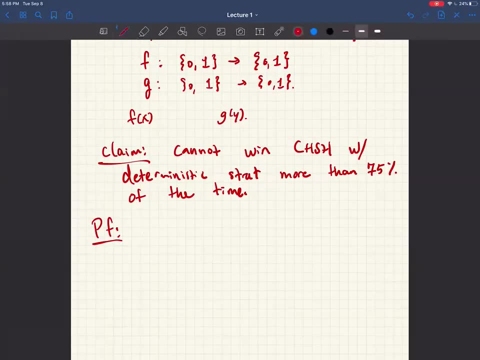 one-fourth of the time. right, And maybe I'll just end with this quick proof. So you know, suppose you fixed f and g, then you know there's four possibilities. right, Because for the questions, so we're, you know, assume for contradiction that they, you know. 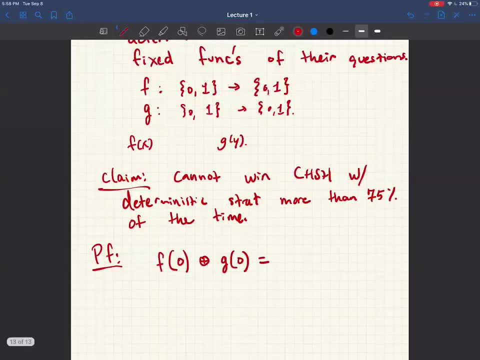 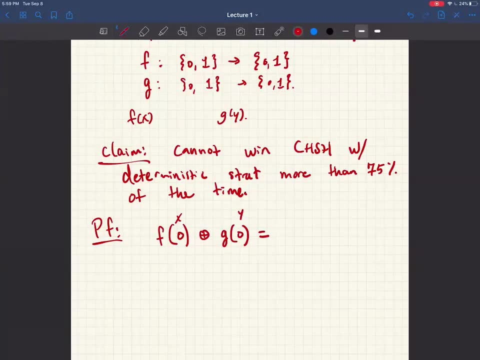 they picked f and g. that satisfied the game-winning condition 100% of the time. So when x is equal to zero and y is equal to zero, then this is the sum of their answers. right, These are the answers as equal to the product of their questions, which is zero. 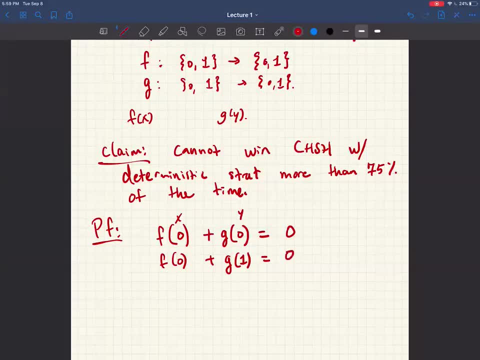 If Alice gets zero and Bob gets one, then you know, this is still zero, Also zero. But if they both get one, then somehow, magically, their answers is also equal to one right, And all of this is modulo two right. 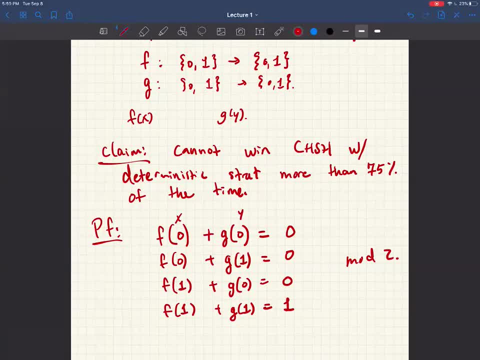 But you can easily see that there's a contradiction here, right? Because you know, if you sum up the left-hand side, you sum up all four equations, since we're summing up everything modulo two. if you sum up something twice, it just cancels. 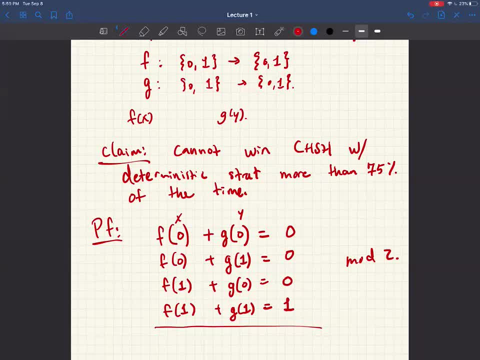 itself out right: F zero plus f zero is equal to zero. F one plus f one is equal to zero. Same thing with the g's, But on the other hand, if you sum up the right-hand sides, you get one right. 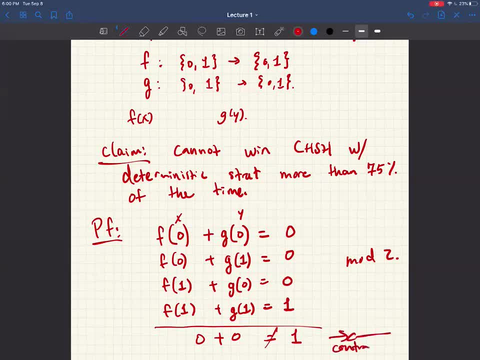 So you know we get a contradiction here. So it's not possible to find functions f and g that satisfy all of this right, So they can't have a deterministic strategy for winning this game Like at least one of these conditions. This must be false. 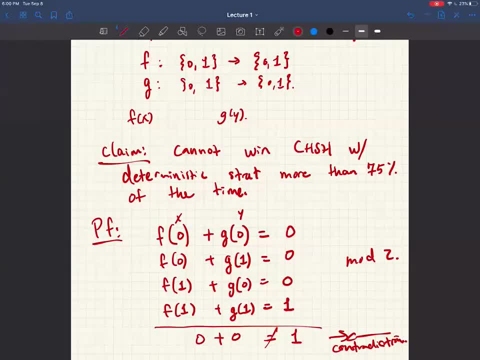 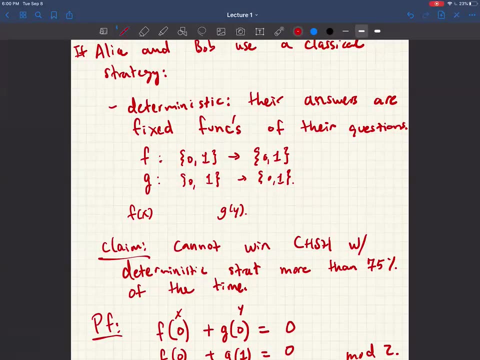 Make sense. Okay, So that's, you know, if they use a deterministic strategy, what if Alice and Bob use a, you know, not necessarily a deterministic strategy, but they're, you know, allowed to. you know flip random coins? you know to like, say, randomize their strategy. you know, maybe that can help. 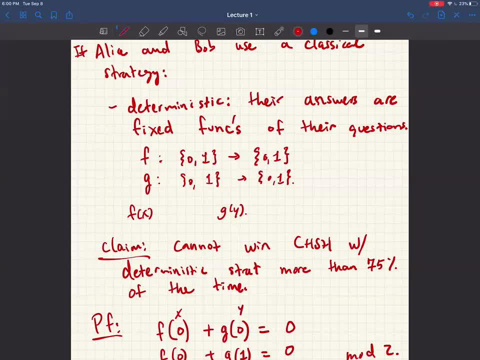 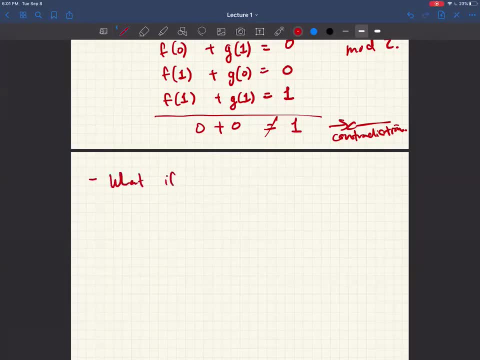 them win this game Better. Okay, This is really the last thing I'll mention Right, Instead of using a fixed function. maybe their fixed function depends on some randomness that they use Right, And what that means is that Yeah. 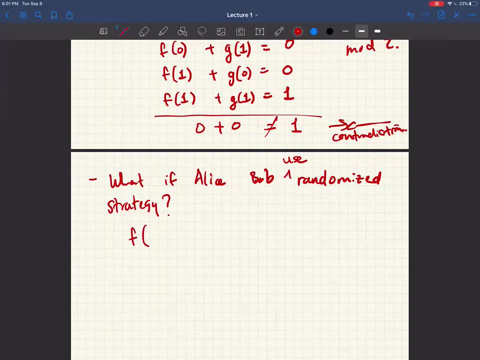 That their functions. you know their answers. you can model it as it depends on their questions, but some additional source of independent randomness are So their. their strategy is some function f of an, R and G depends on Y and R. Maybe this synchronized R allows them, helps them win. 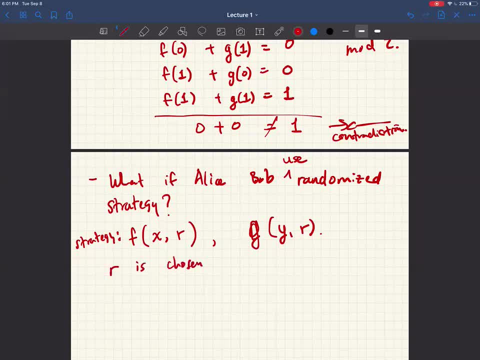 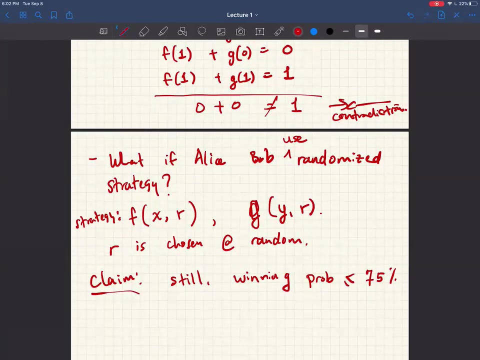 Yeah, Well, you completely into. Well, the claim is that this doesn't help. Okay, This doesn't. actually, you know, they might as well use a deterministic strategy. Okay, What we'll finish up with next time is: we'll see, you know, that if Alice and Bob instead use quantum entanglement, they can actually do better than 75%. 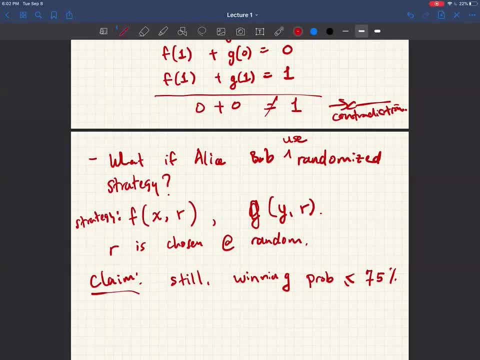 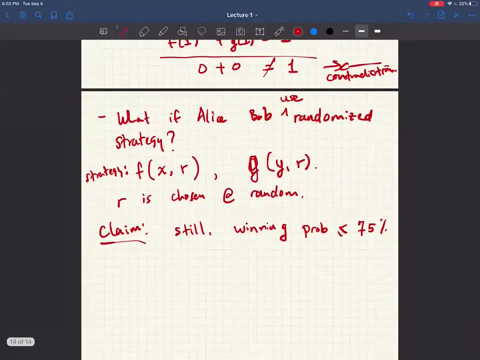 So you can do. you know, classically you can't do better than 75%, but using quantum entanglement you can. And that tells you that quantum entanglement cannot be described classically. Okay, well, so that's it for today. 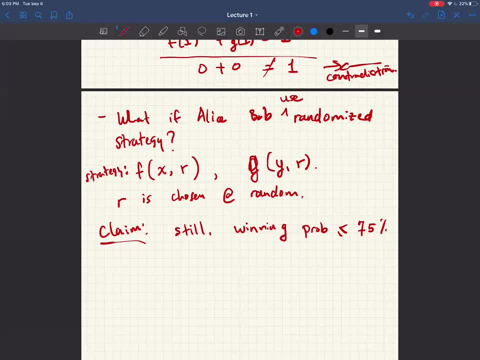 A couple of announcements. One is that please sign up for the Slack And it'd be great if you, you know, just you know. introduce yourself, say you know, said like you know, your status or your graduate student, what you're studying, what you're interested in. 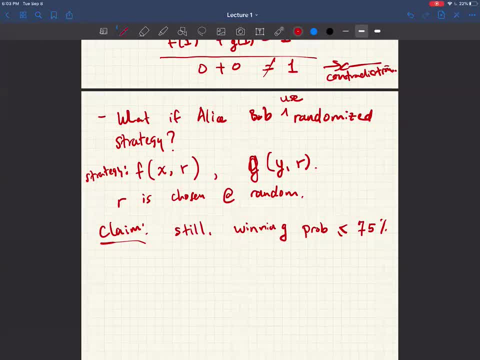 And that'd be great for you know, for finding project groups and problem site groups. Another thing is I've released problem set one And, you know, hopefully it should be a helpful way of you know, refreshing yourself in quantum information and determining whether you you know, whether you're you know, that you understand the background. 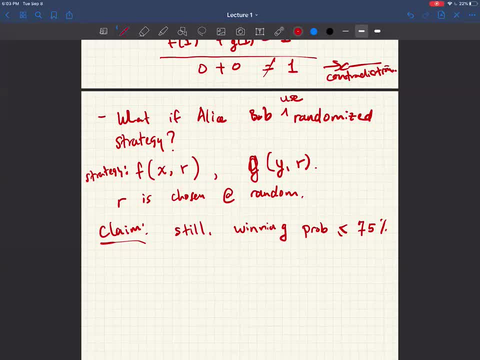 It's due September 21st, So about several weeks from today. And yeah, that's it for today. Thank you, Any questions? I actually cannot find the Slack link, the invite link. Can you reshare it? on the Quarkus? 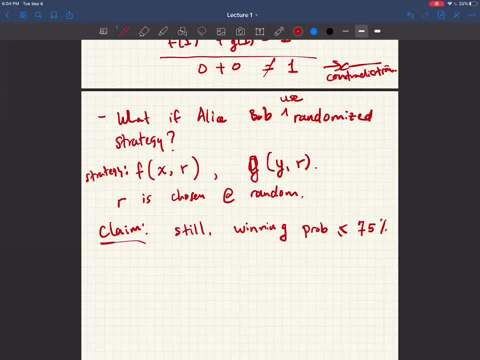 Oh, sure thing. Yeah, Yeah, Yeah, It's in the syllabus, but let me post it. I'll post it a couple times in different places. Yeah, Sorry, Thank you very much, Uh-huh. Yeah, I just have a question about notation again. 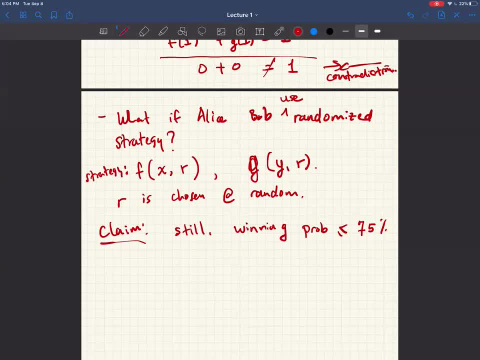 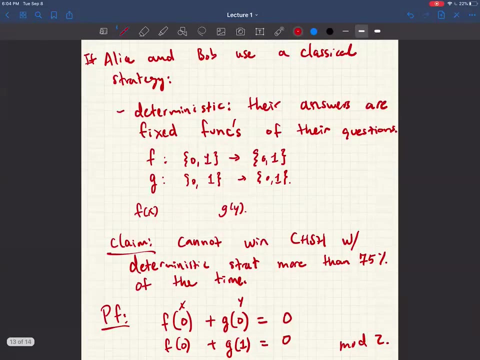 Sure. So in the last example you're using um like F of zero. uh, one, not of, but like F with a curly bracket: zero one, Mm-hmm, Wondering what those are. Oh, you mean this thing. 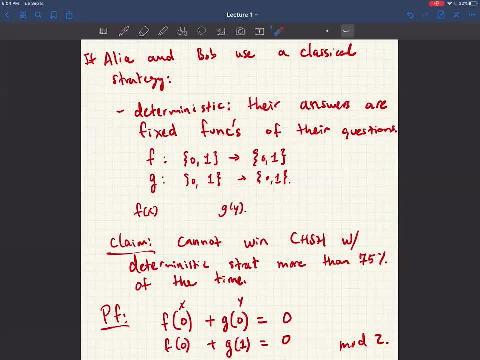 Yeah, Oh, that's just saying that F is a function from the set zero one. Uh, so it takes in either zero one and it outputs zero one. So it's a very. it's a function of, of of a bit and outputs a bit. 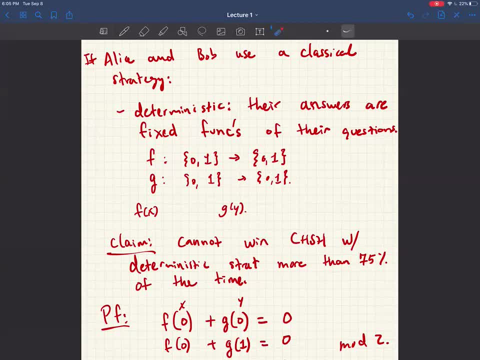 Okay, So it's not. it's not a qubit, No, It's just uh like a fixed mapping, Like you can think of it. as you know. it's just a table. you know. F is saying: if I get input zero, uh. 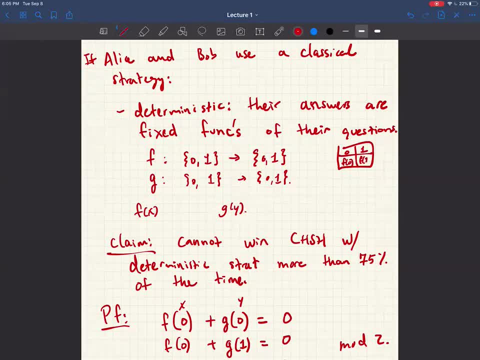 then I output. If I get output F of zero, if I get one, then I'll put F of one. Okay, I was trying to relate it to the qubits and I was getting confused. Okay, Oh yeah, Here There's nothing quantum. 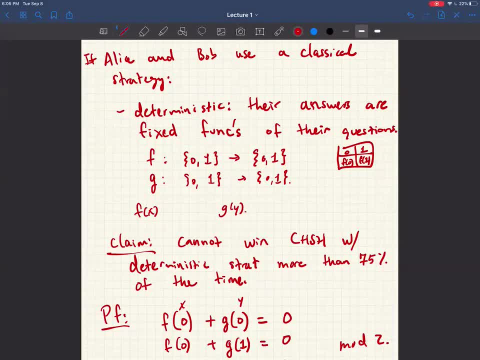 Like so far, I'm just talking about classical stuff. Okay, Got it. Um. and then one more question, uh, for the zero, zero and the one one. I was a little confused. Um, like w with the Yeah. 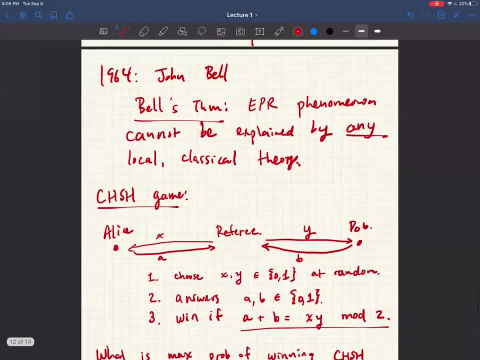 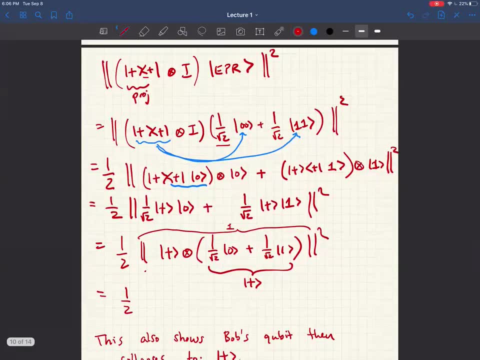 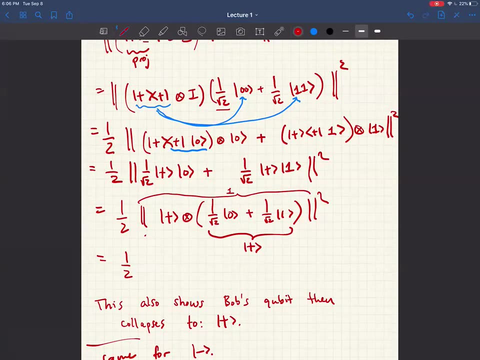 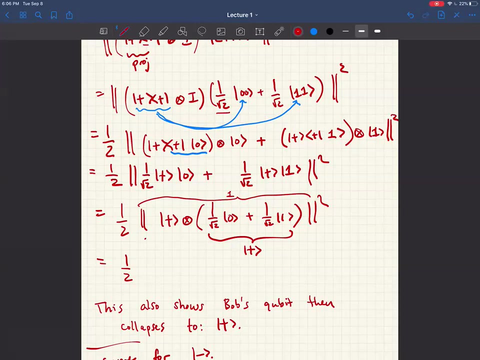 Yeah, So I guess, why would it? it would apply to the first one and you would get one over two. um, like in in the first, in in the first blue arrow, Uh-huh. Um, I guess to why that would apply to the, to the first zero. 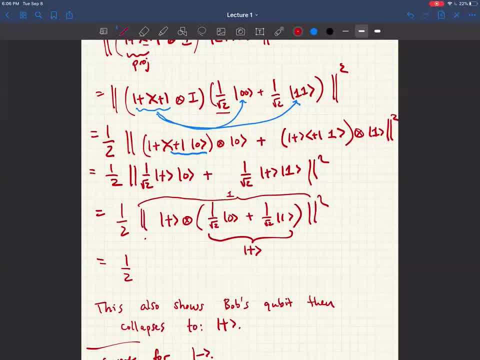 And then you mentioned that you would get like one over root two. Oh right, So let me draw a little aside. I think it might be just notation for me, or Yeah, So, um, so, let's, let's forget, let's say there's just one qubit. 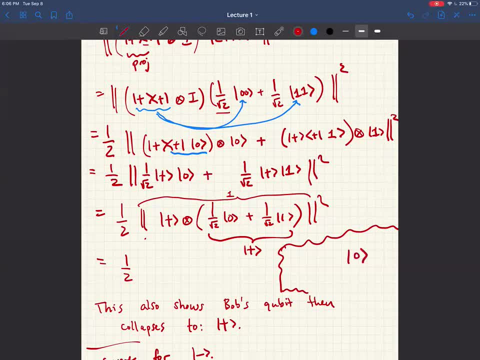 Um, so let's say I had one qubit in the state zero and I applied a projection like, say, plus the plus projection, or, let me say it again, I wanted to project the zero qubit onto the Okay, The zero qubit onto the plus state. 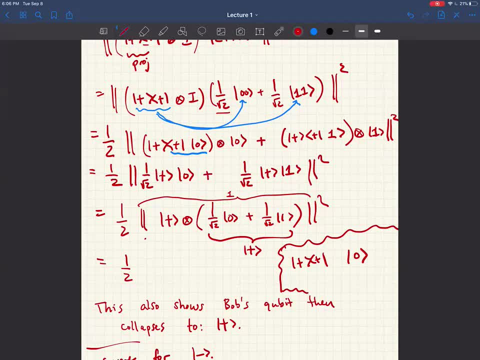 Okay, Uh, so mathematically that looks like this: I'm, this is a matrix, right, Because it's, uh, it's the outer product of a vector with itself, uh, which is, uh, it's a matrix times a vector. 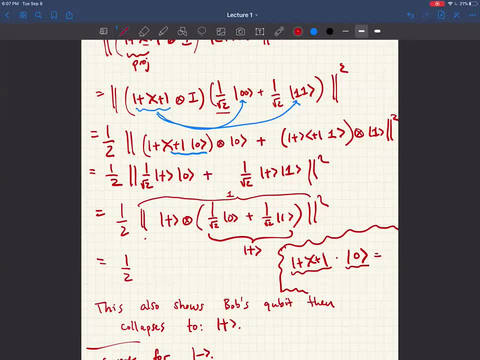 So you're going to get a vector right, Um, yeah, But but we're going to also use this nifty like this is why this broadcast notation is is, uh, helpful because, Okay, Because we can sort of move around these together. 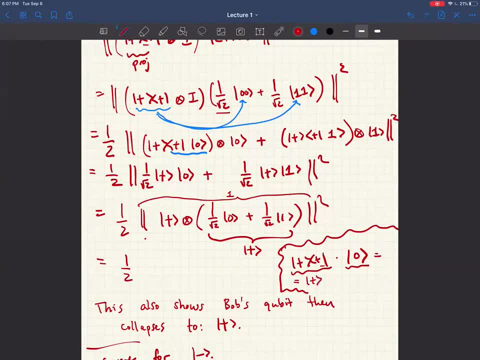 So this is the same as just plus, and then I'm going to move the plus and the zero together, Right, Like algebraically this: these are exactly the same things, but, uh, I'm going to regroup them so that this, this is a vector- times it's transpose. 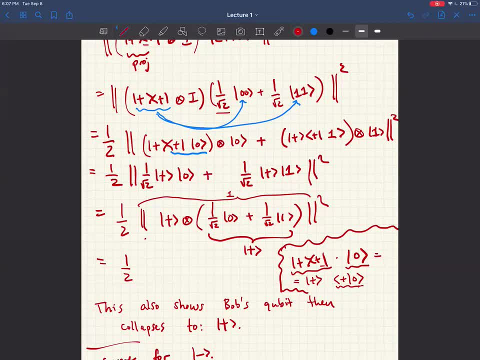 And this is a number Vector times. it's uh, okay, Right, So this is going to be like a row vector, which is the plus state times, The column vector, Yeah, Which gives you a number, And then you're left with a vector. 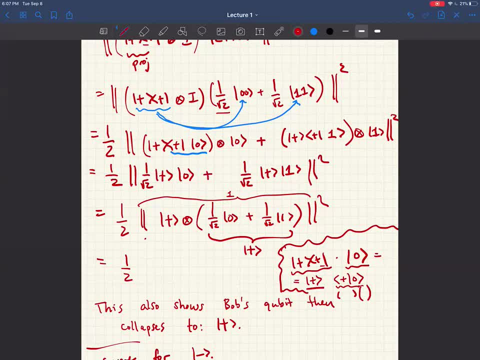 I mean, which all works out right, Because you're multiplying matrix times a vector, you get a vector. It's going to be the plus state times this number. Well, what is this number? Well, it's the inner product between the plus state and the zero state, which is one over root two. 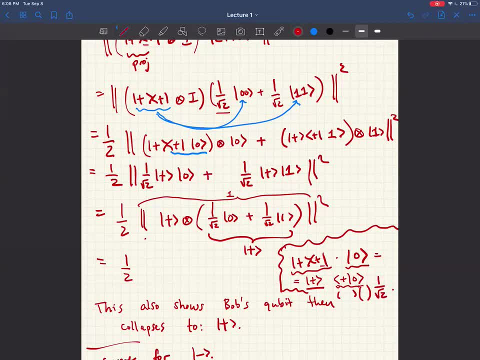 Okay, So it's. so it's not just one over two, It's one over two times. uh, this vector plus Okay, And that's because we can rearrange the bras and cats Exactly. Yeah, Got it. Thanks so much. 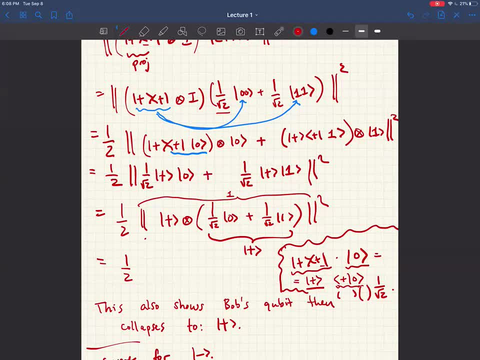 Yeah, And so, and feel free to. uh, you know, use the Slack to ask questions. I'll try to answer throughout the week and you know other people feel free to answer in. Okay, Um, but uh, other than that, I think that's it for today.